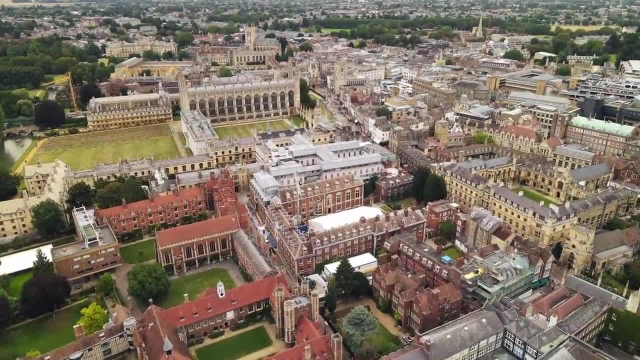 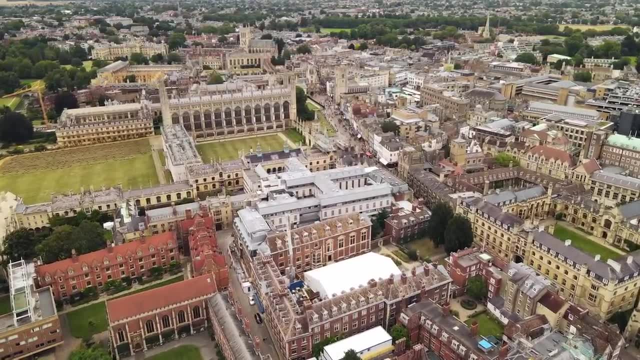 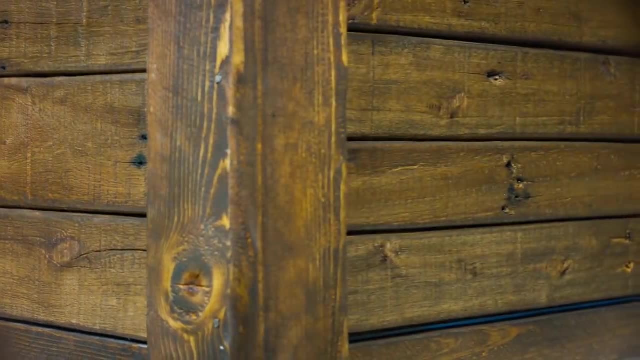 heavy oak door of the ground floor lodgings. It is just as well they are on the ground floor because the parcel that greets him fills the entranceway. It is a huge crate, battered and splintered. It must have taken three or four porters to. 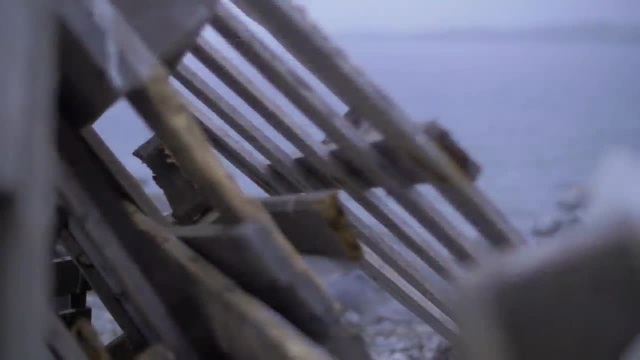 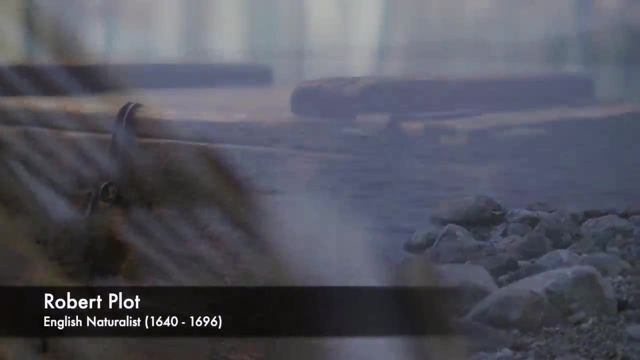 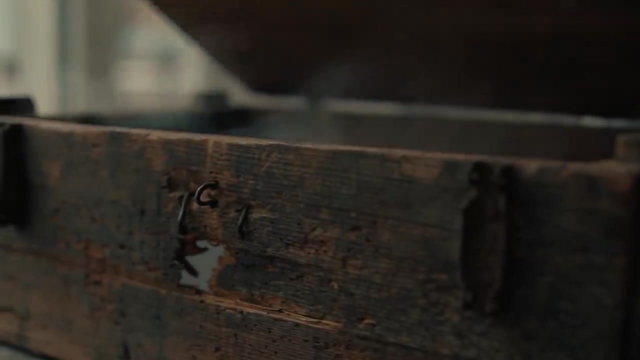 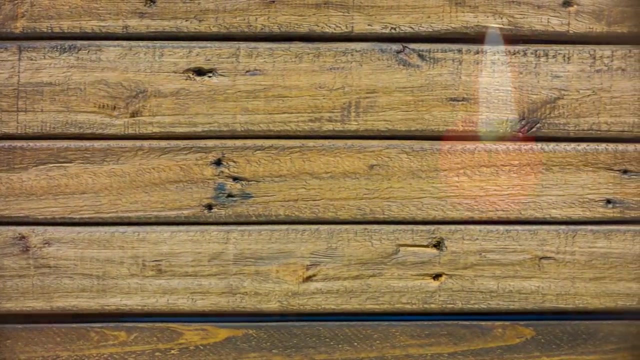 bring it inside, not to mention the poor horses that pulled it all the way from Cornwall. Plott wastes no time in prying the wooden slats apart and revealing the bounty within. Nestled among straw and wooden shavings, there are rocks, Curious shapes and patterns. each 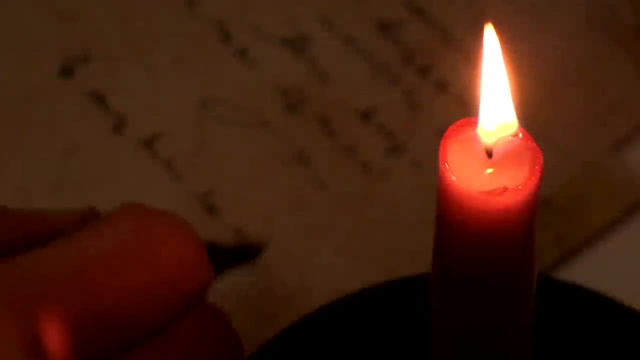 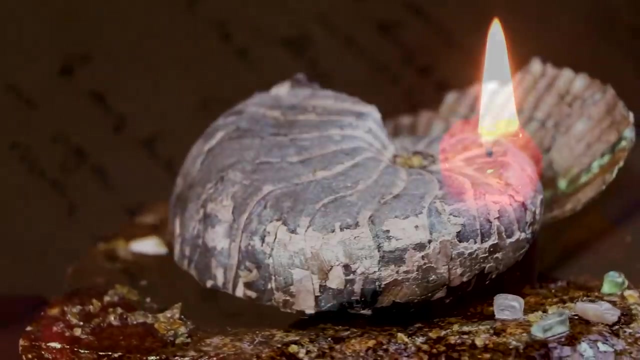 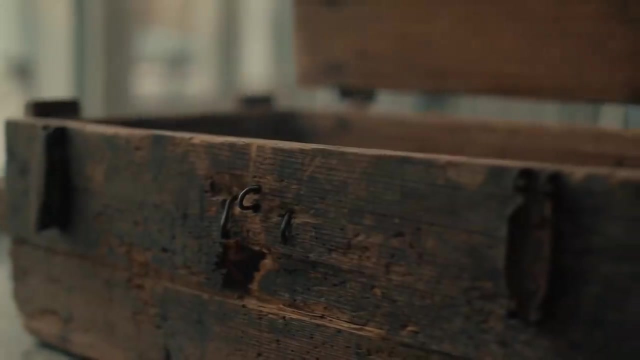 accompanied by notes written in loose, flowing cursive. He pulls each one out, briefly admiring it, turning it in his hands before setting it down and reaching in for the next. When the crate is almost empty, his searching hands encounter a smooth, rounded surface. 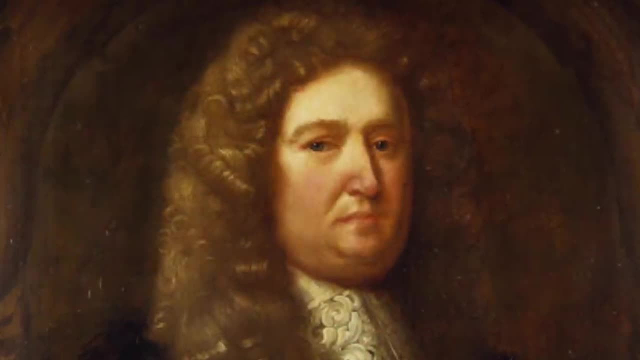 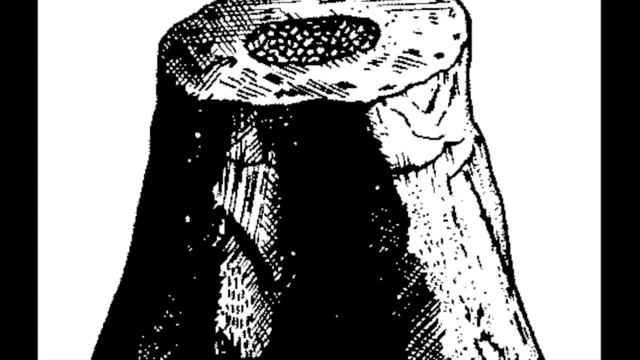 to pull it from its nest. The reverend marvels at this unique specimen. The crate is almost empty. his searching hands encounter a smooth, rounded surface. The reverend marvels at this unique specimen. Two rounded bulbs join where they touch and morph into a smooth cylindrical stem with 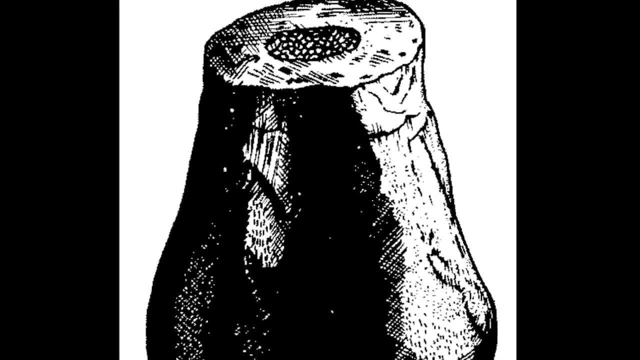 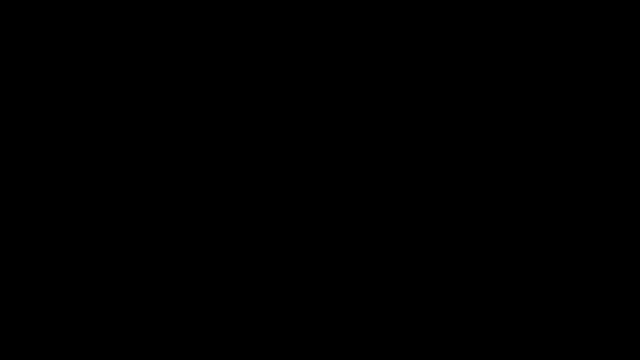 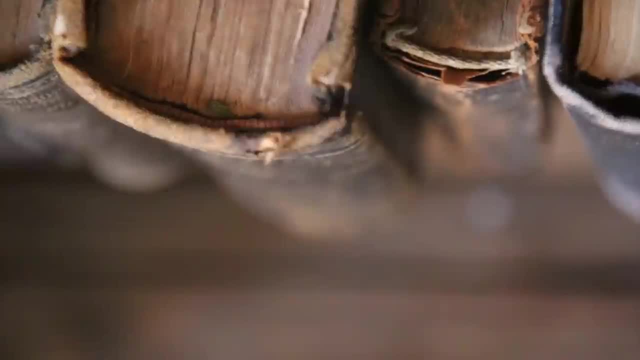 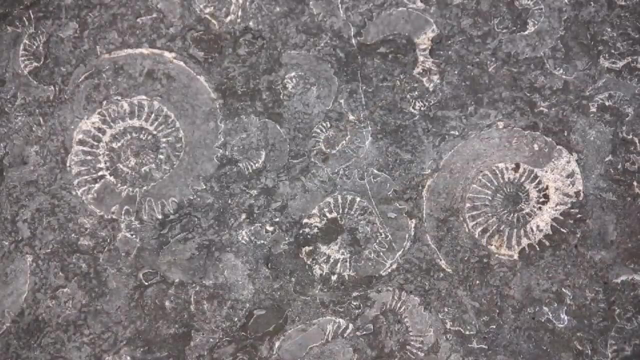 a seemingly hollow centre To Plott. it looks like a bone, But it is made from stone and it is unusually huge. At this time in the late 17th century, debate runs rife among natural historians as to the true nature and origin of fossils. 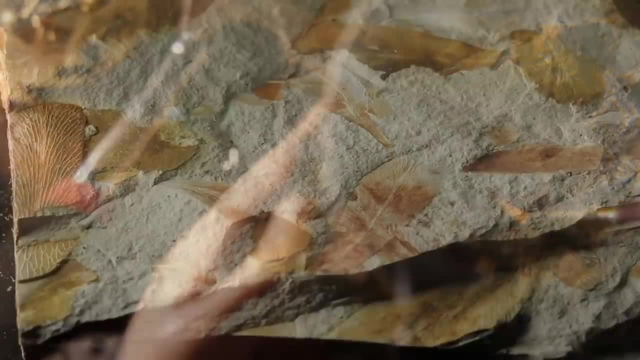 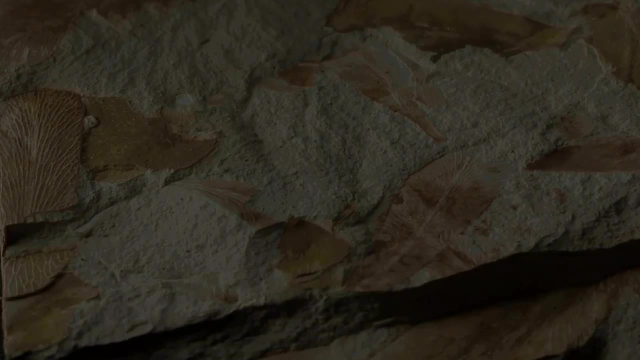 Some believe them to be the remains of ancient creatures long since dead, while others prefer to dismiss them as tricks of the eye, shapes that are formed naturally by the growth of salt crystals beneath the ground. Others still suggest that fossils are the so-called seeds of plants and animals that 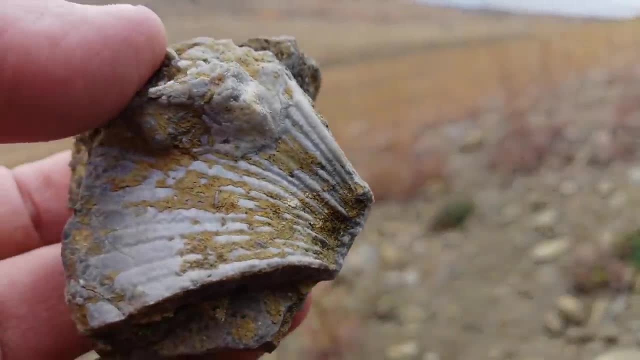 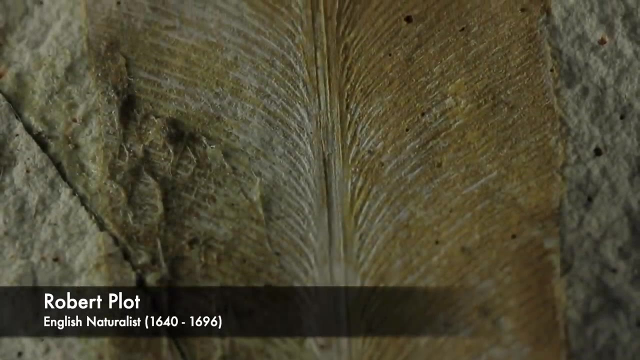 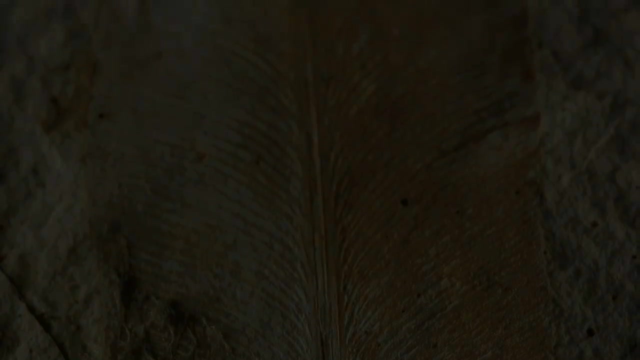 have descended deep into the earth and begun to germinate there. But Robert Plott is a sceptical man of science and, with no way that he can see for living things to be preserved in solid rock, he tends to favour the salt crystal interpretation. 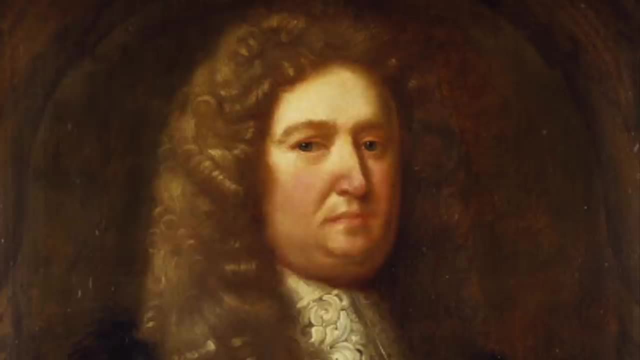 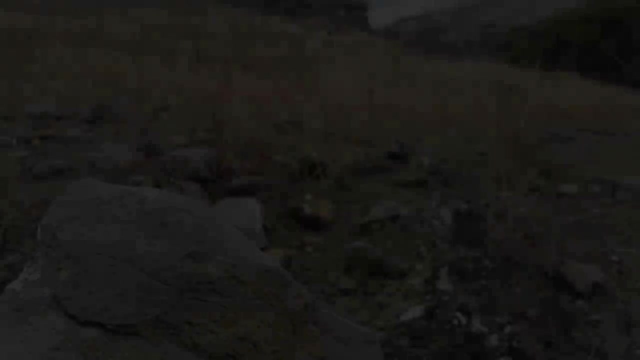 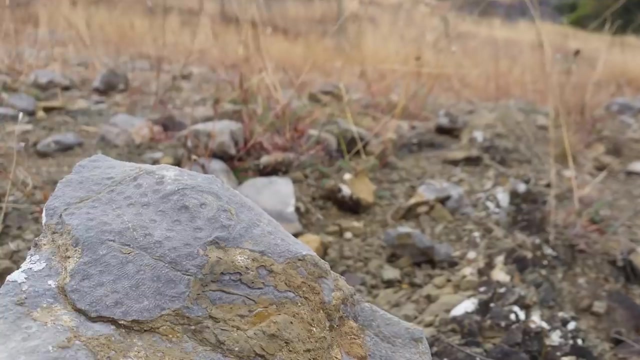 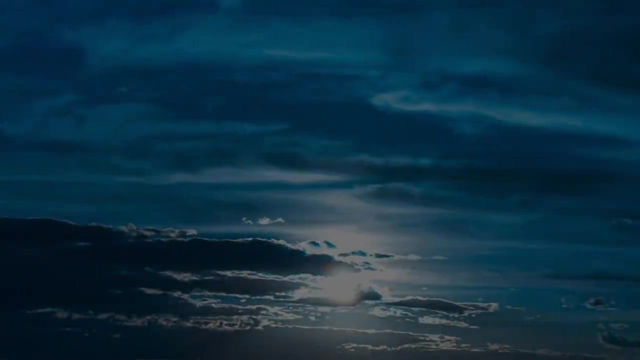 He has spent the last few years studying the shell-like fossils found in Oxfordshire quarries, likening them to the crystal patterns produced by, of all things, crystallised urine. But not all structures to be found in the rocks can fit this simplistic crystalline. 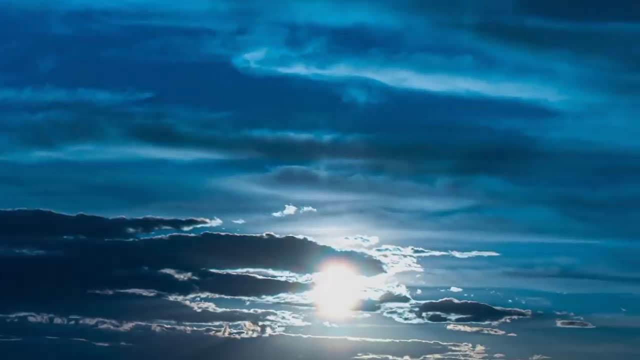 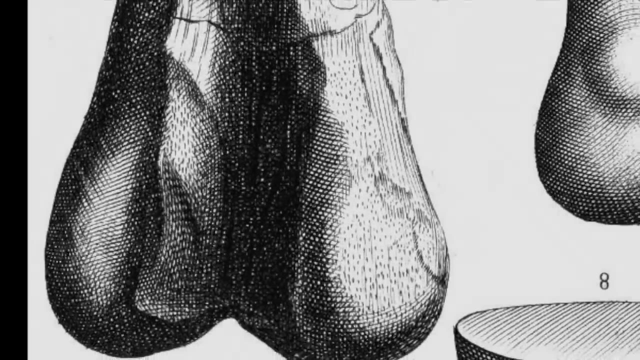 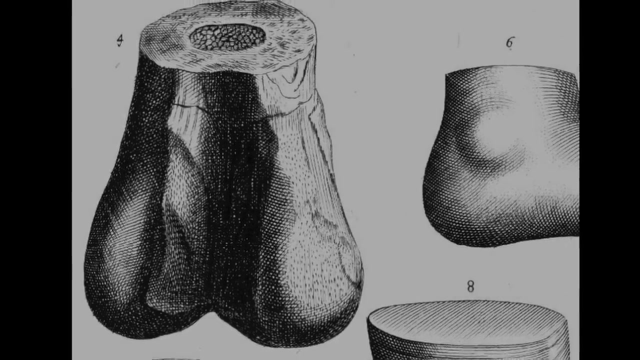 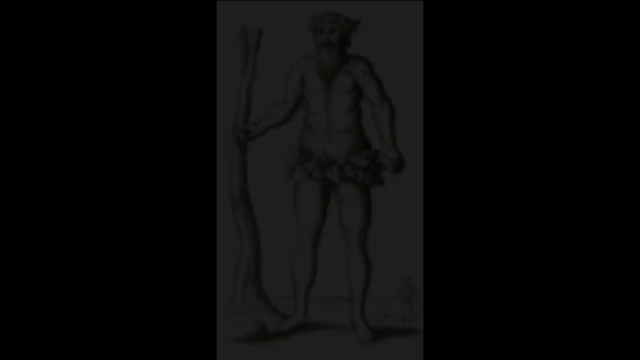 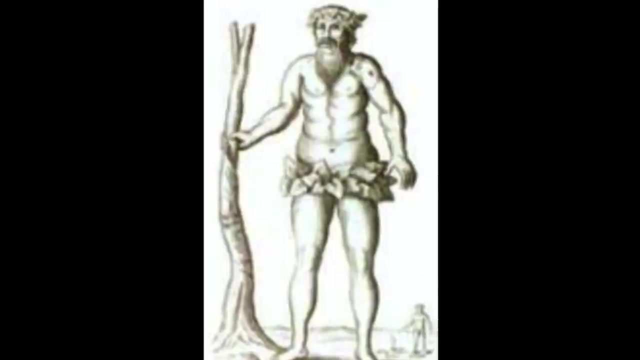 explanation, Plott eventually concludes that this magnificent specimen is in fact a petrified leg bone of some unimaginably large creature. Perhaps it comes from something like the impressive Roman war elephants he saw in the flesh just a year earlier. or perhaps it belongs to a long-lost race of giants. 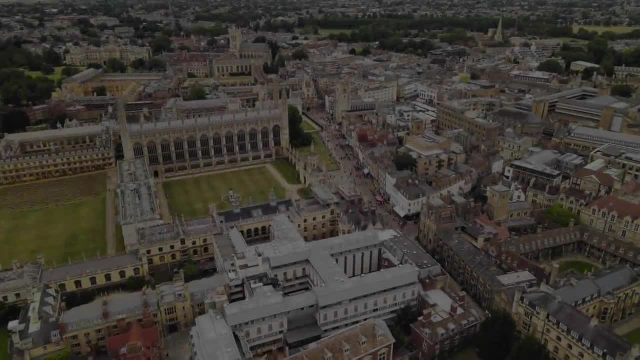 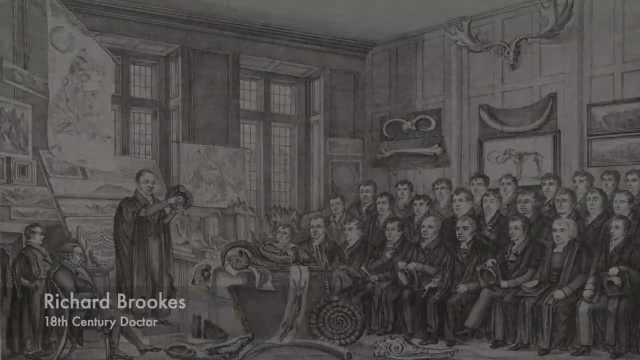 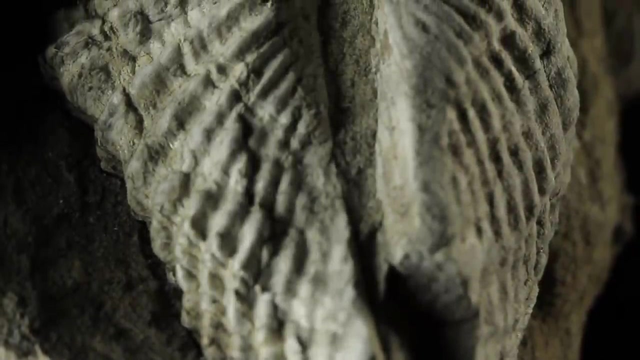 And so, 100 years later, the bone, now part of Oxford's natural history collections, is studied again by another man of science. His name is Richard Brooks. The understanding of fossils had advanced by this point, and many more accept the possibility. 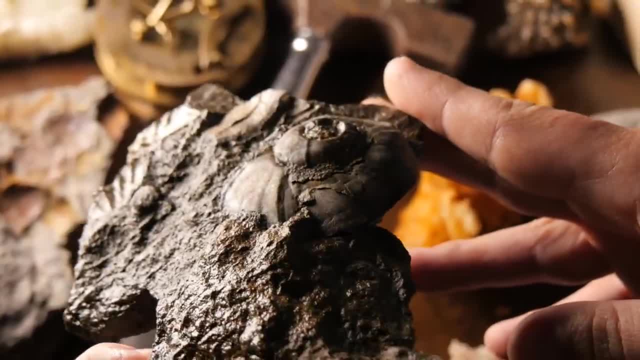 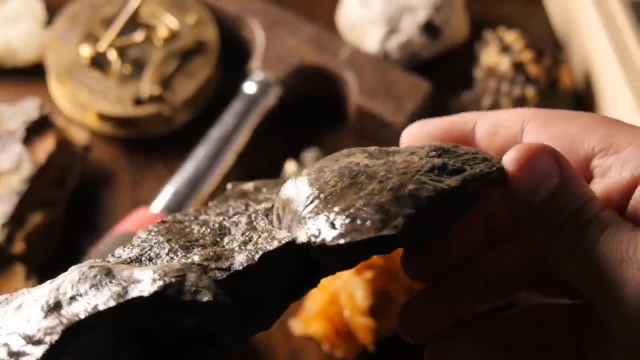 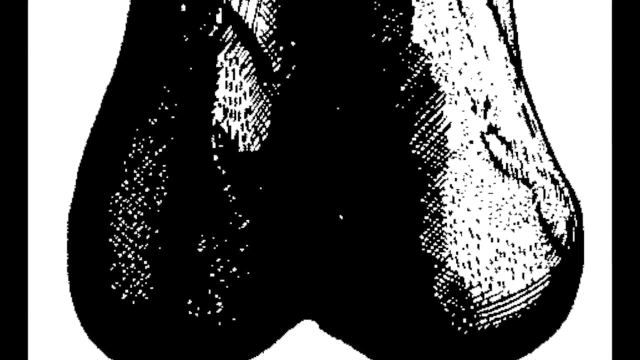 that they are remnants of long-dead creatures, And Brooks is keen to use his knowledge of animal and human anatomy to interpret this curious specimen. For the first time, he gives the rock a name: He calls it STAROCK. 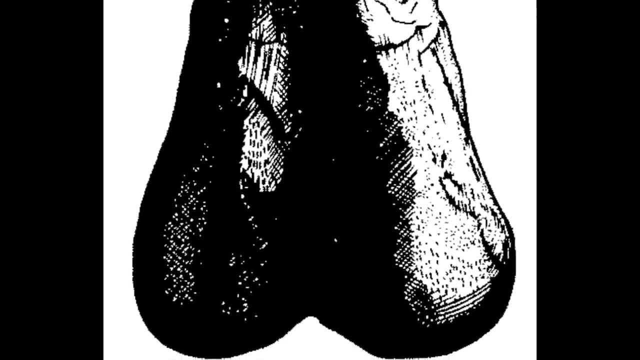 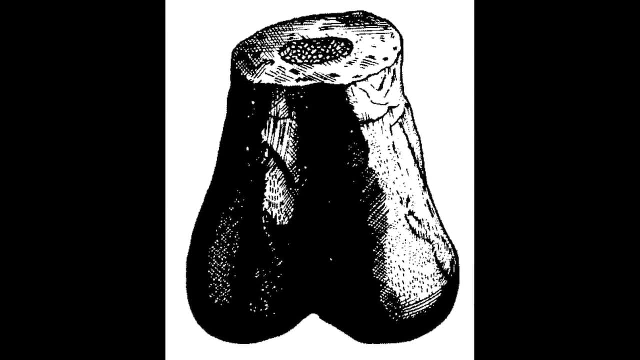 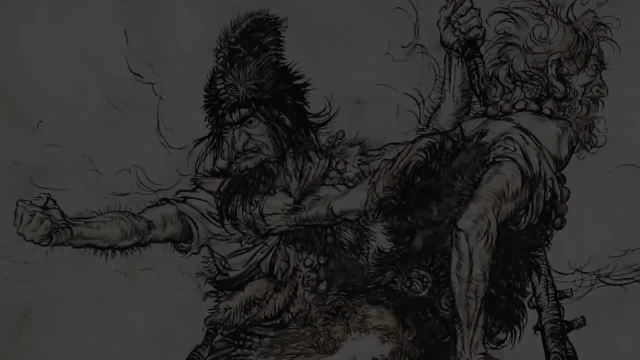 STAROCK 行 and calls its scrotum humanum, making clear the fossil's kinship with a certain specific part of a giant human's anatomy. Of course, Brooks's interpretation was a little off the mark. We have no evidence of a race of giant humans, either by the bones or the stones they left. 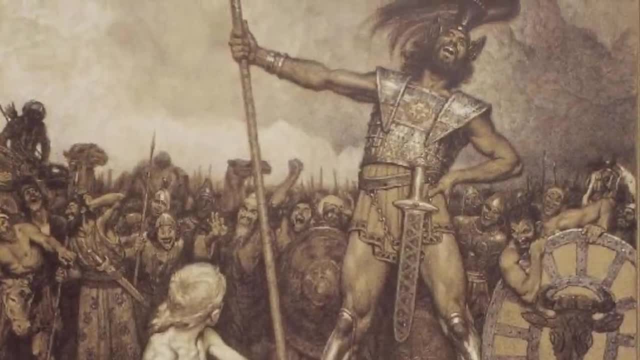 behind Plott's Cornish bone has now been identified as the thigh bone. One character namedbound in the X Prize is then identified with its rock. The billions have been up to the bones. Of course, this makes much less sense since versus its actual structure- and everyone is. 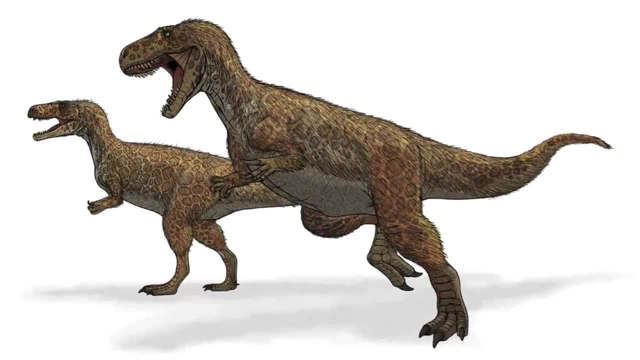 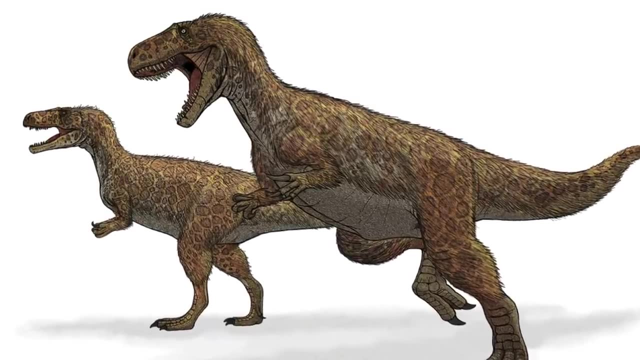 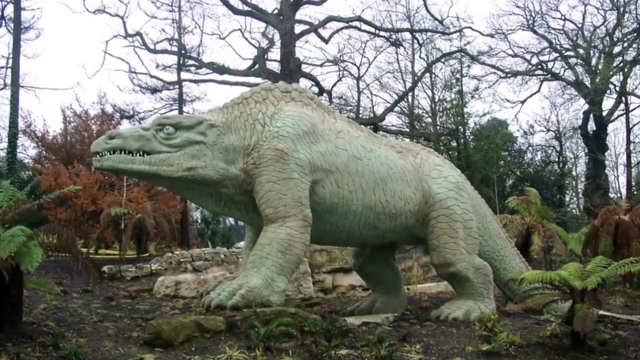 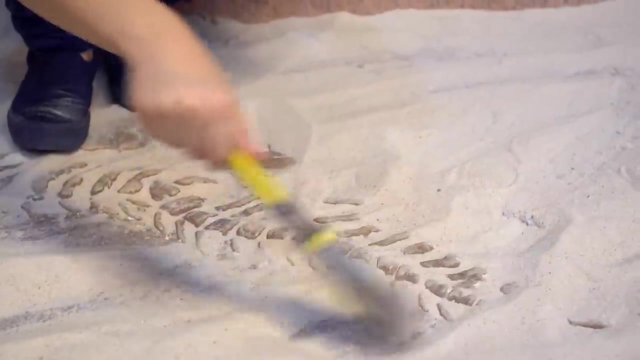 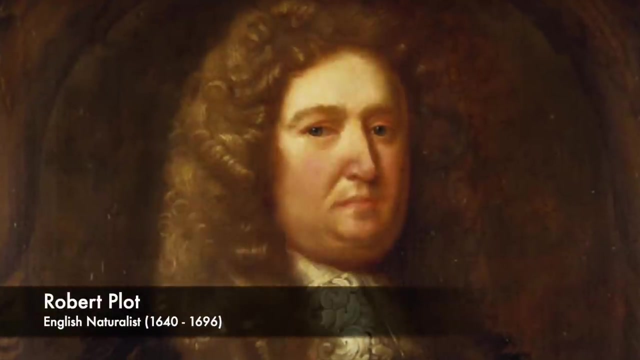 of a megalosaurus, the first dinosaur ever to be described. Since the dawn of paleontology, scientists have been forced to challenge the assumptions about what is and isn't possible, about what Earth's rocks really tell us. Plot and his contemporaries were occupied with whether fossils 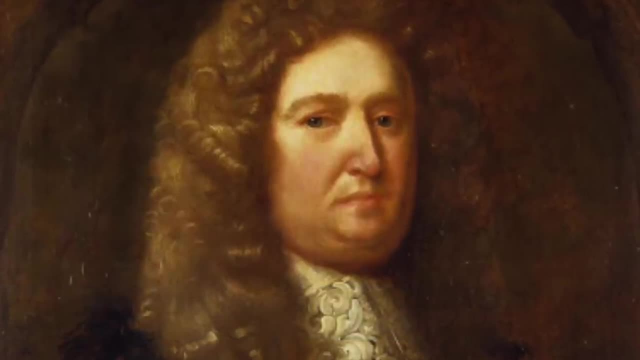 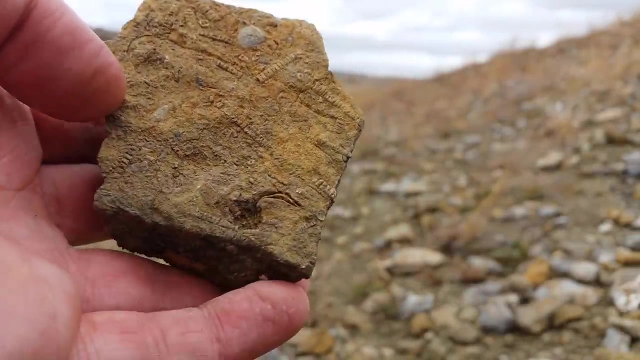 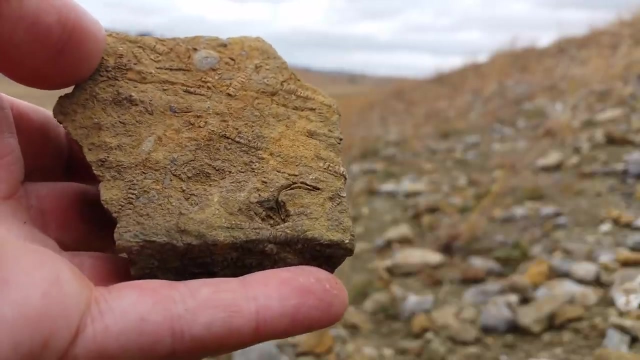 were even real at all, But now we use them as a tool to probe our own multi-billion year history. Just how much can the fossil record show us? How far does it go back Can we use it to find the first complex life? 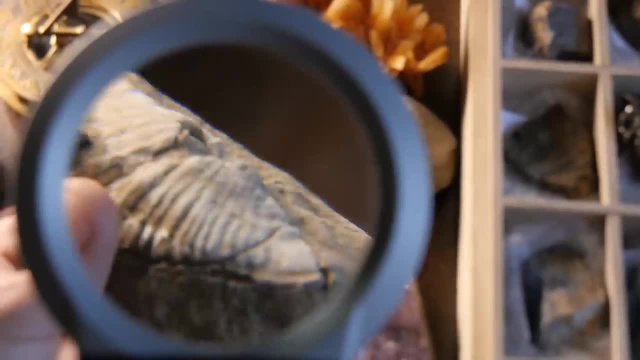 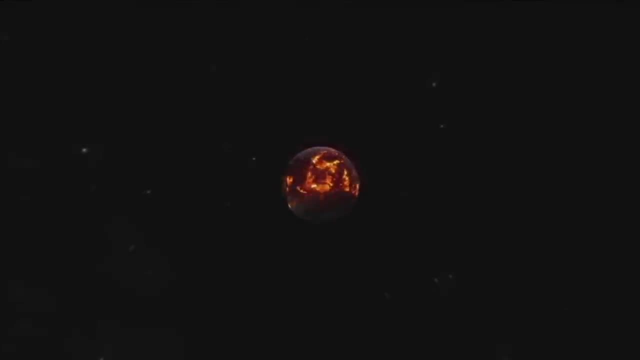 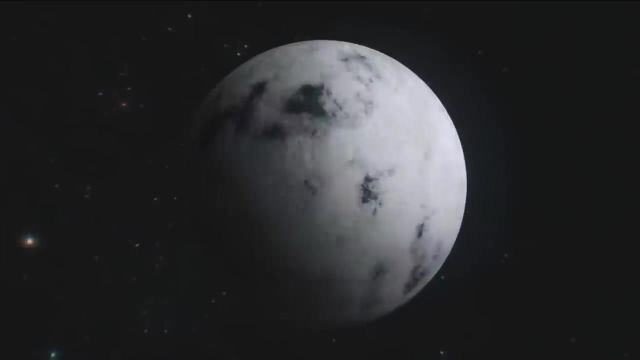 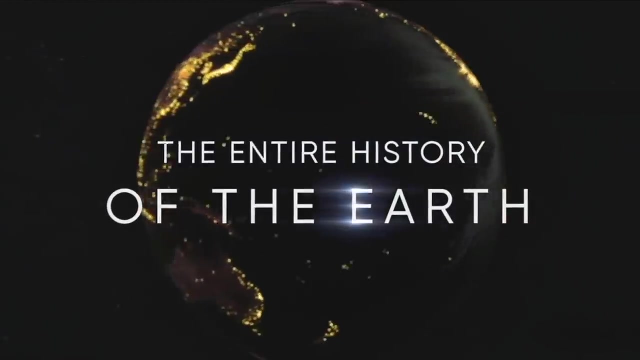 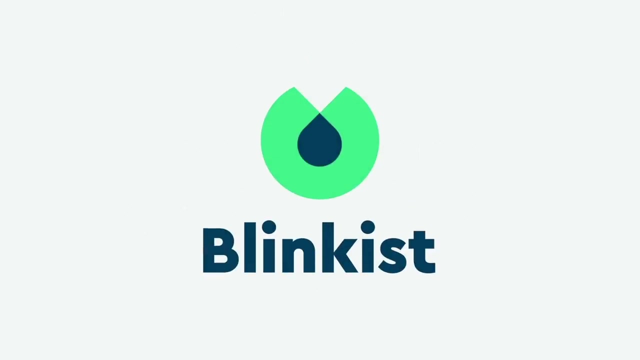 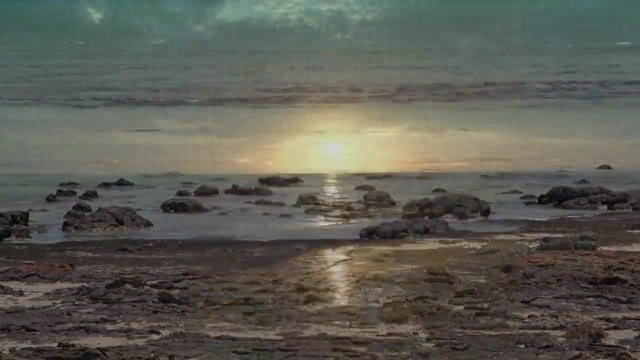 And how Can we be sure our interpretations are correct? This video is sponsored by Blinkist, an excellent tool for absorbing knowledge wherever you are Ever wanted to read a classic book, but simply couldn't find the time. Well, Blinkist is here to help you out. 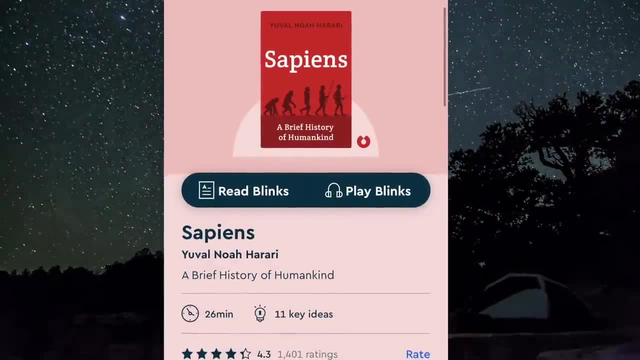 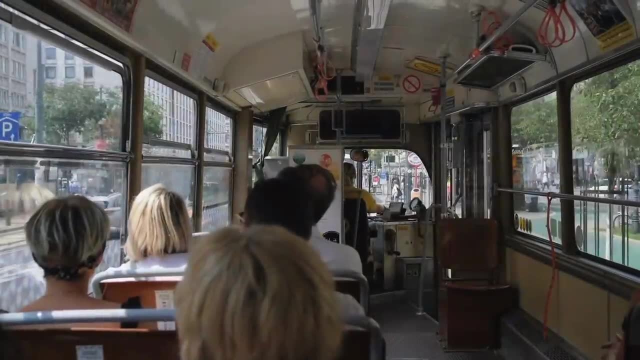 Breaking down epics ranging from sapiens to the origin of species into 15-minute bite-sized chunks you can easily absorb on your commute or other times that would otherwise be wasted. It's a truly excellent tool for lifelong learners and a great accompaniment to our channel. 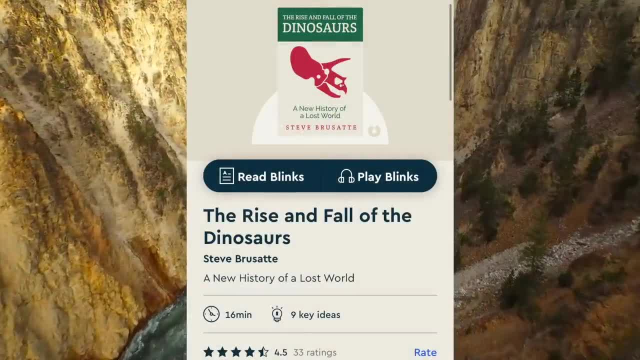 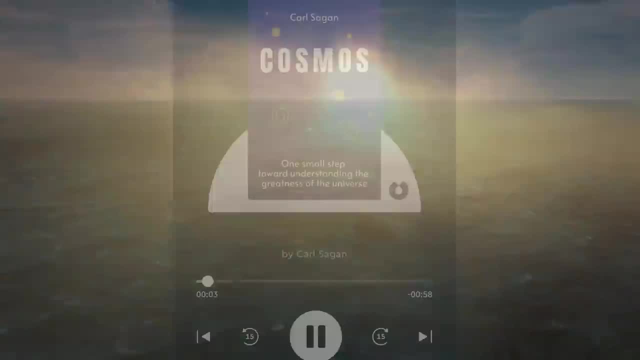 should you wish to learn more. Like other educational apps, all you need to do is download the app, sign up for an account and you can listen wherever you are And when you do. make sure to use our link. We've teamed up with Blinkist to offer you. 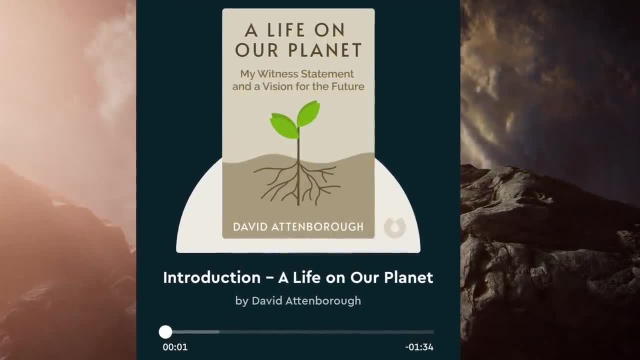 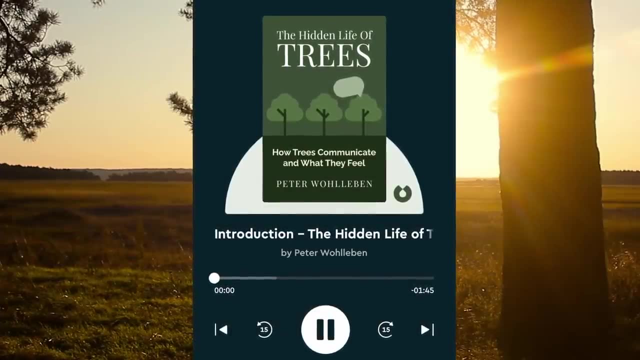 an exclusive seven-day free trial and 25% off a premium membership. More than 5,000 titles are already available, with more being released all the time, So click on the link in the description below to activate your free trial now. Thanks, 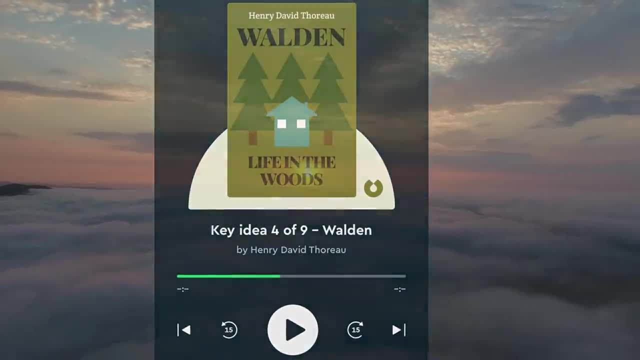 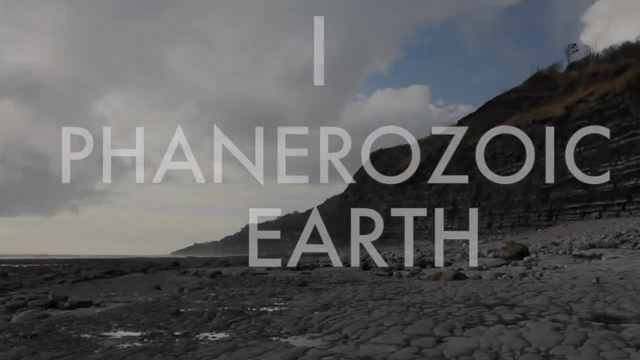 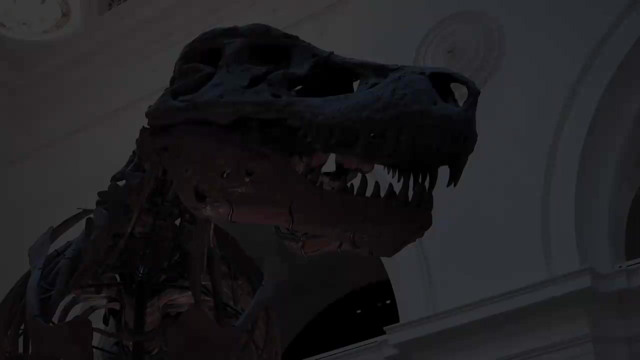 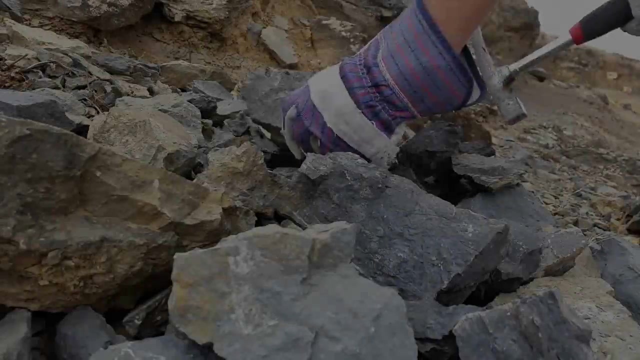 Now back to Earth, Earth's distant past. The chances of anything becoming a fossil, be it a towering T-Rex or diminutive dragonfly, are vanishingly small. The circumstances and conditions that allow traces of life to persist through geological time are so few in number. 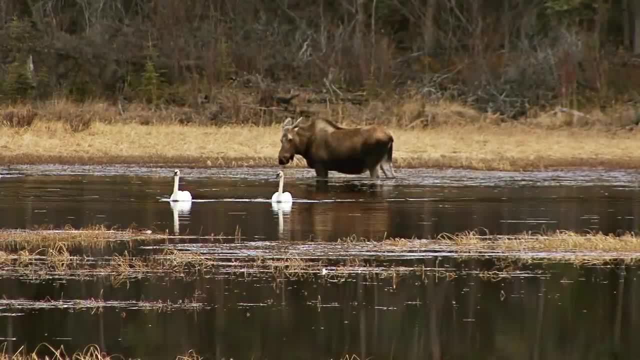 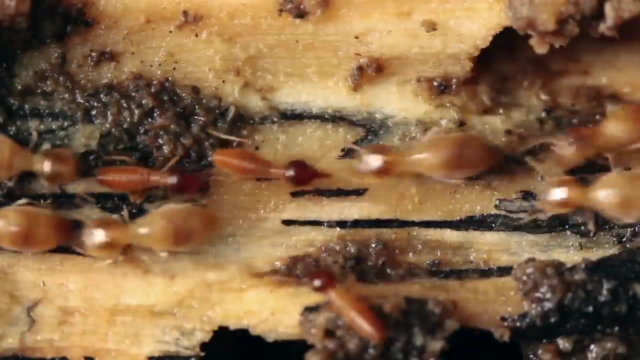 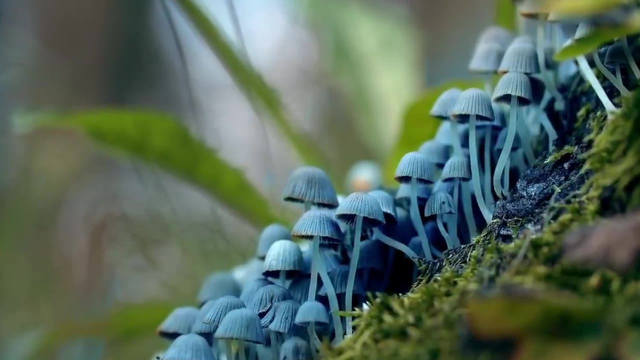 as to be almost impossible to engineer or predict. Normally, when an organism dies, it is simply eaten by another creature, recycled back into the great circle of life, Even if not consumed by a predator or scavenger. microscopic detritivores and saprophytes. 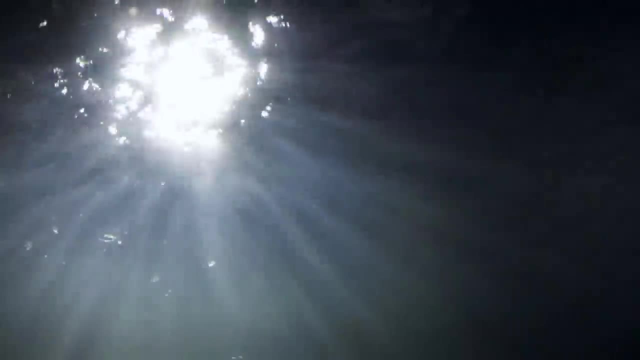 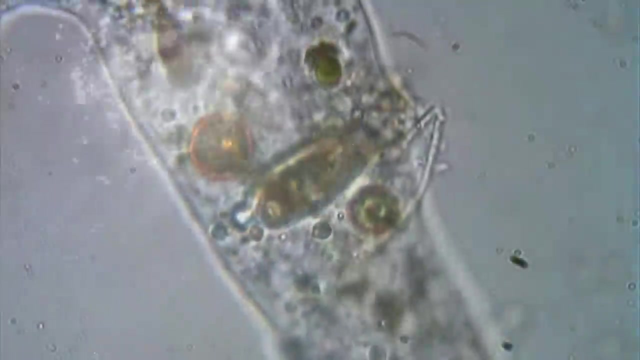 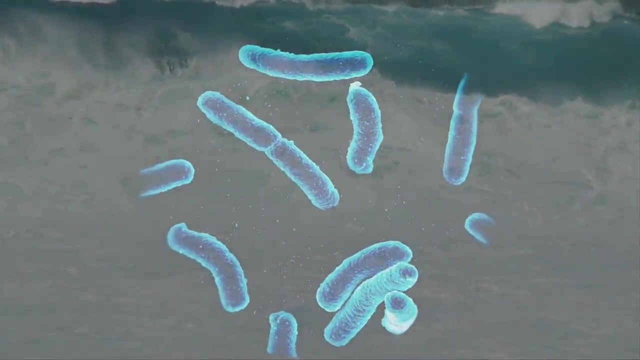 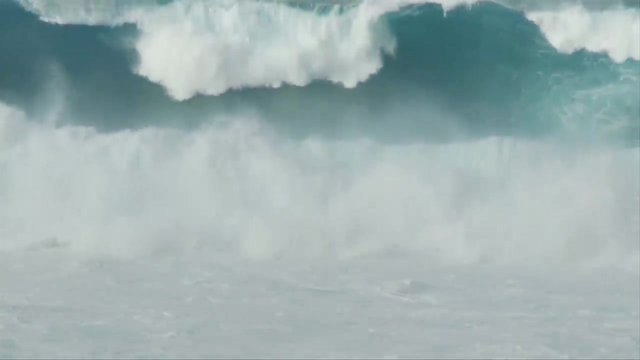 colonizers of forest floors, riverbeds and ocean bottoms make short work of any organic matter that falls into their DNA. Bacteria break down and water washes the rest away, leaving only the hardest bones and shells. In time, these too will oxidize and crumble away to dust. that becomes soil and nutrients for the next generation of life. This is the fate of almost anything that has ever lived to be so thoroughly broken down to our component molecules and reincarnated in the next cycle of life. But in some exceedingly rare cases. 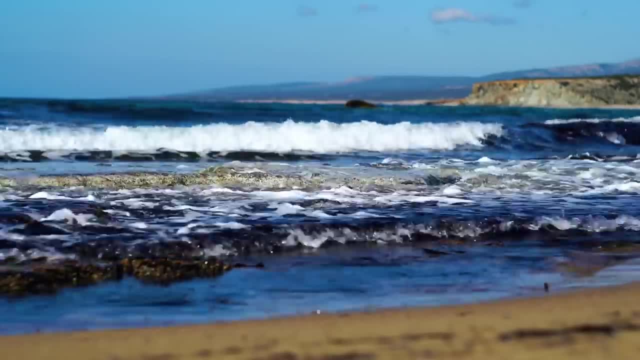 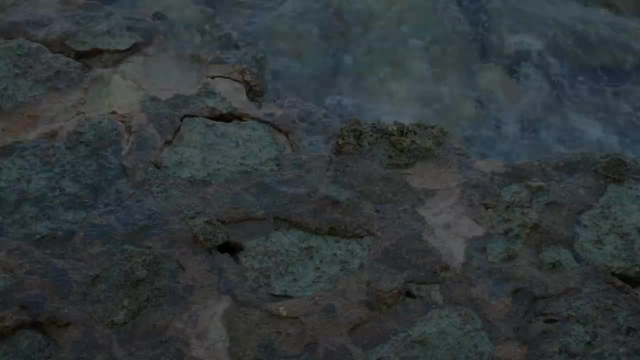 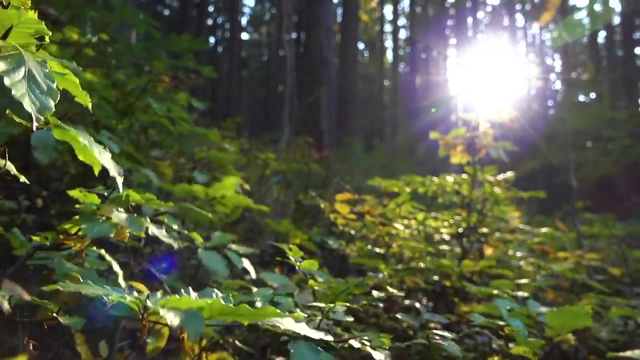 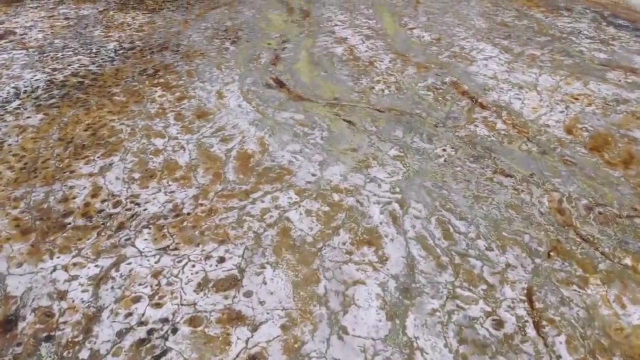 a dead organism, against all probability, is able to break the wheel to escape the endless cycle. There are a few places on Earth where the relentless recycling of organic matter is sufficiently slowed to allow some remnant of a creature to persist long enough to leave a trace in the rocks. 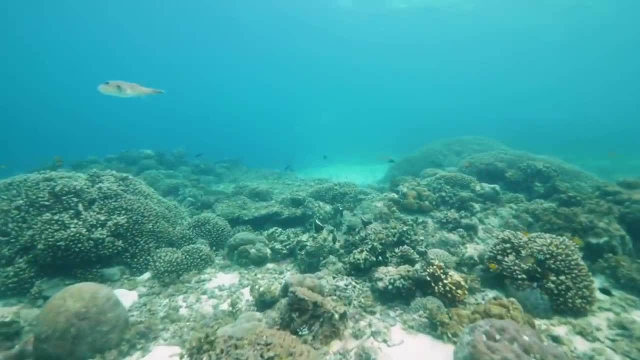 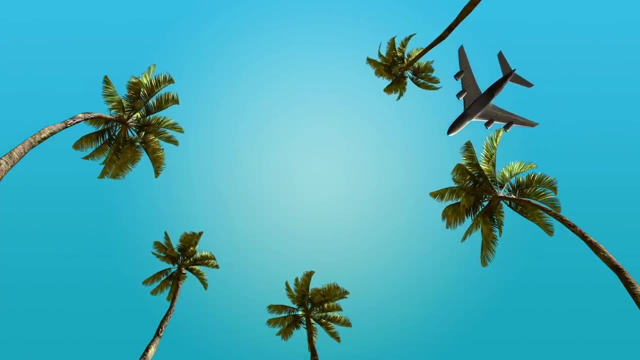 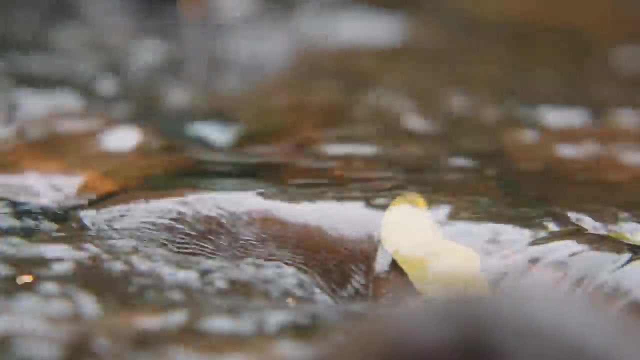 Perhaps an animal is washed away to the ocean depths, never stopping anywhere long enough to become food. Perhaps a fallen tree is so quickly covered by mud and sand as a river breaks its banks that it's swamped before the rod sets in. Or perhaps a freak change in water chemistry? 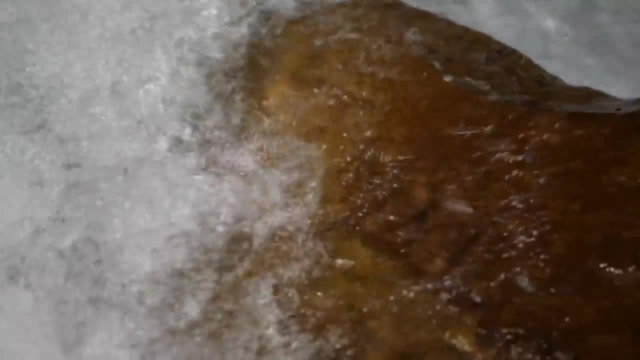 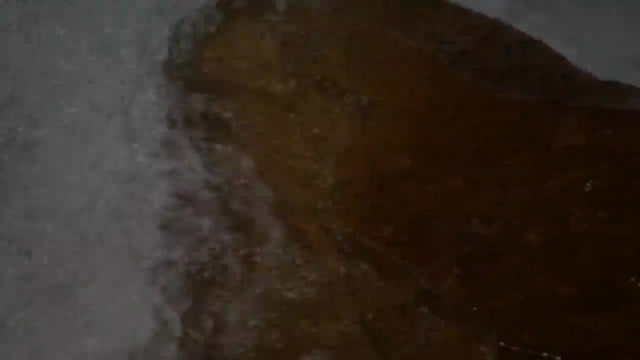 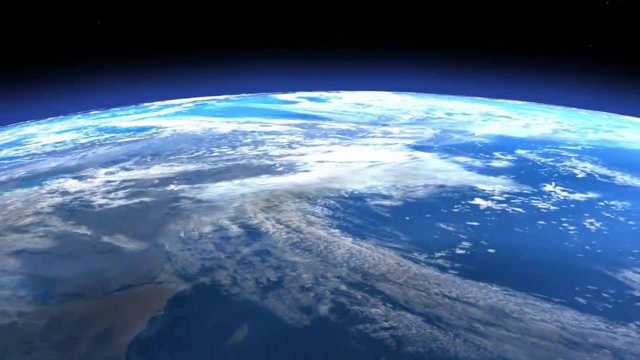 is enough to kill everything stuck within its toxic extent, excluding potential scavengers, for many years to come. Of course, life on Earth is famed for its tenacity, and there are a few physical or chemical phenomena that can keep voracious bacteria from escaping. 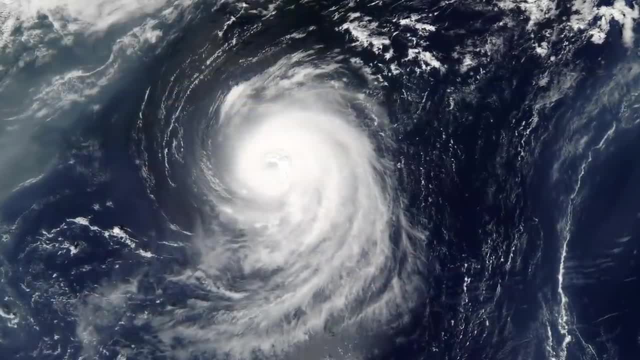 But there are also a few physical or chemical phenomena that can keep voracious bacteria from escaping. But there are also a few physical or chemical phenomena that can keep voracious bacteria from escaping At bay, Even in the deep dark ocean, depths meters below the surface of a tarry swamp. 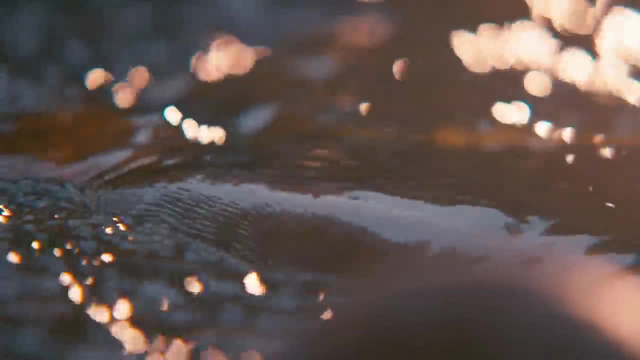 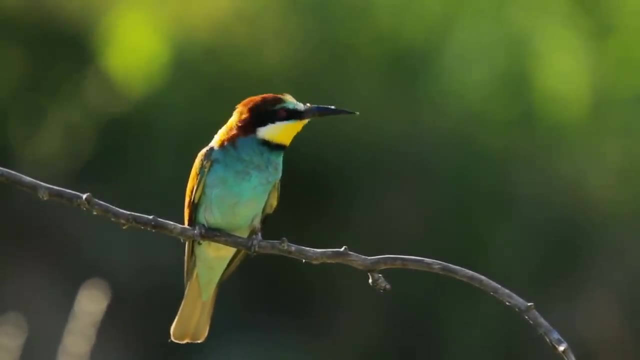 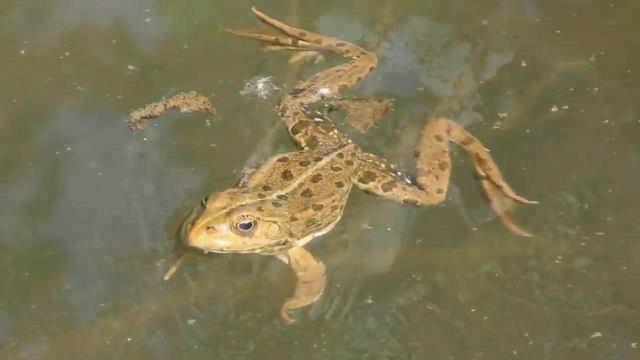 or in a seemingly toxic pool of acid, there will be bacteria able to survive and feed on the organic bounty that comes their way. Soft flesh is easy pickings for these microscopic scavengers, and they leave only those hard parts: bones, teeth and shells. 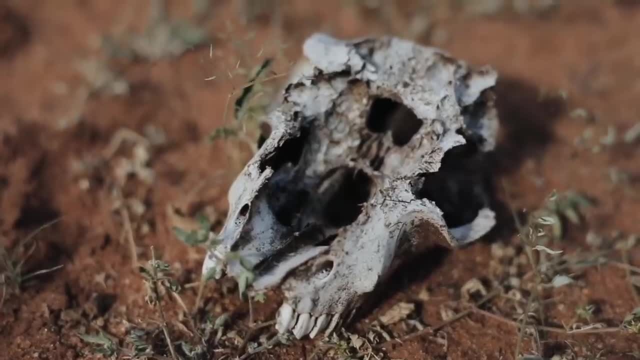 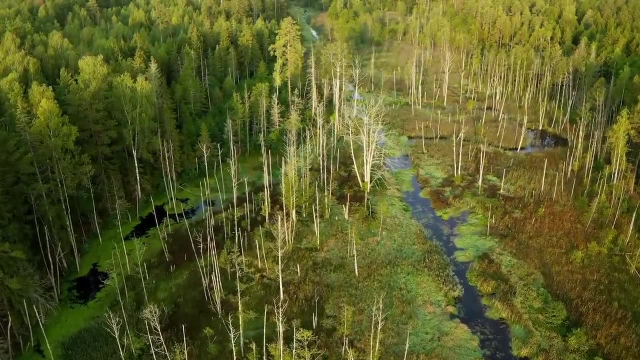 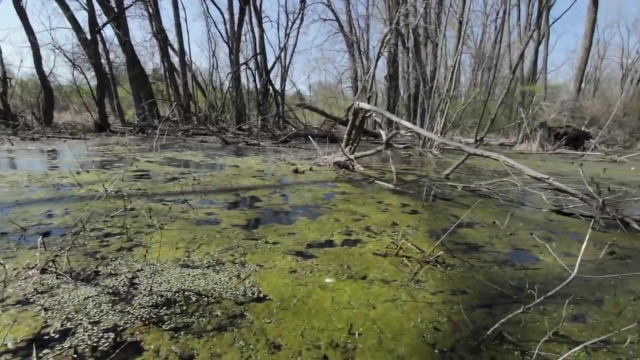 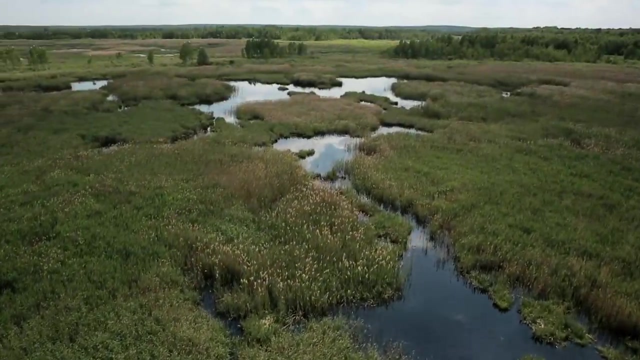 that are too tough to consume. so in these dark, buried chemical exclusion zones, the hard parts persist and become one with the rock. over time, the soft sediments are compressed by the weight of more deposited on top, water is squeezed out, new minerals are precipitated, and old 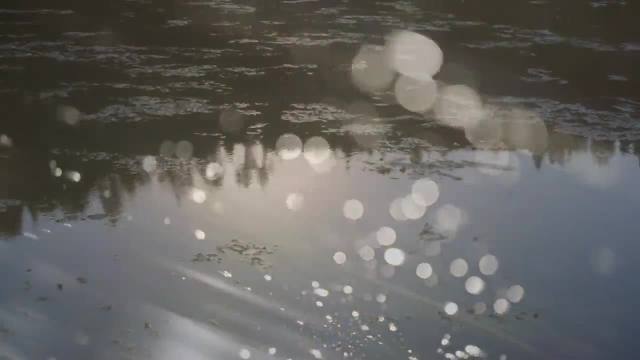 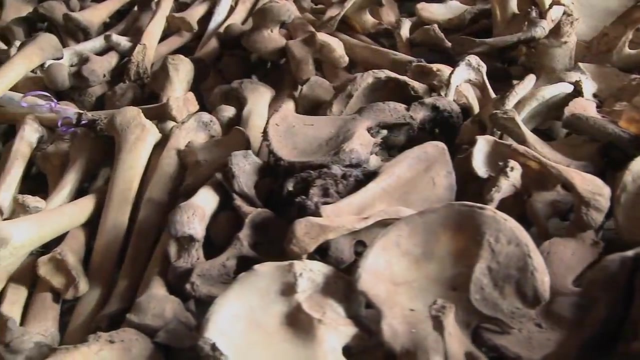 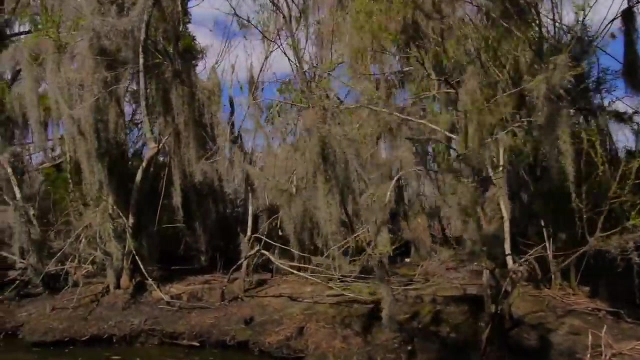 minerals are lost. fossilization is now a race between chemical and geological processes. as sediments turn into rock, can new minerals move in and preserve the structure of the bones, teeth and shells before the original minerals are lost? in the rare cases that they do, a fossil is born. 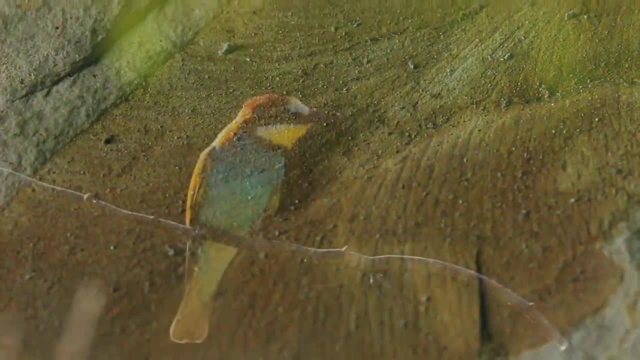 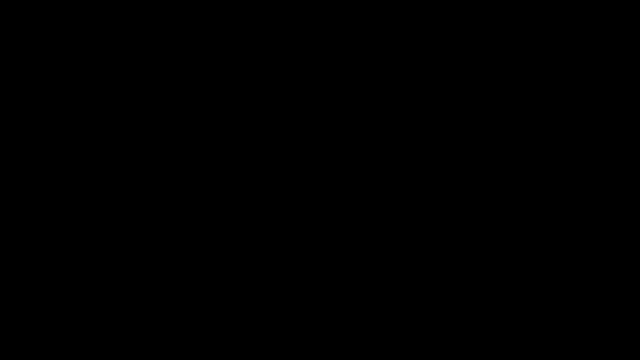 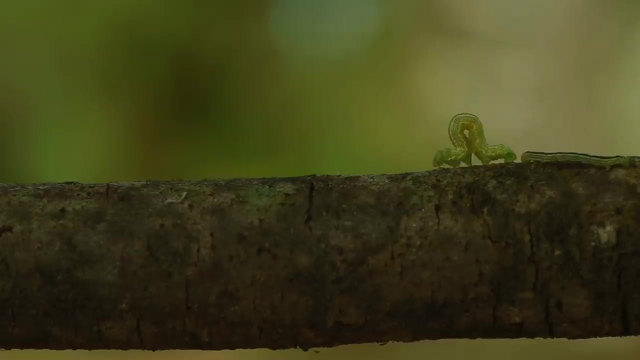 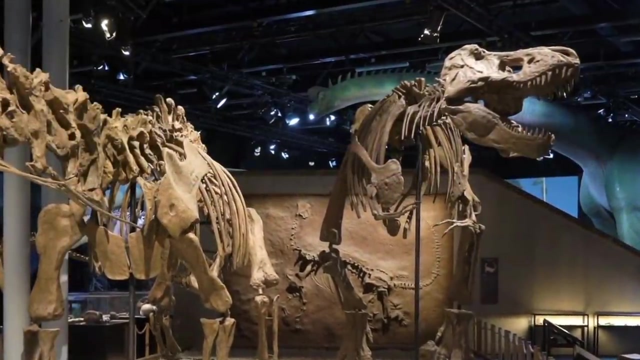 if not, then even the hardest of shells is dissolved and the void it left crushed out of all existence. this unforgiving gauntlet, which every dead organism must run if it hopes to be granted a fossil afterlife, sees only one bone in a billion preserved within the 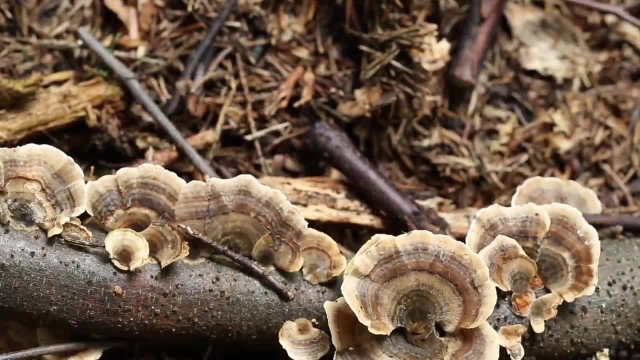 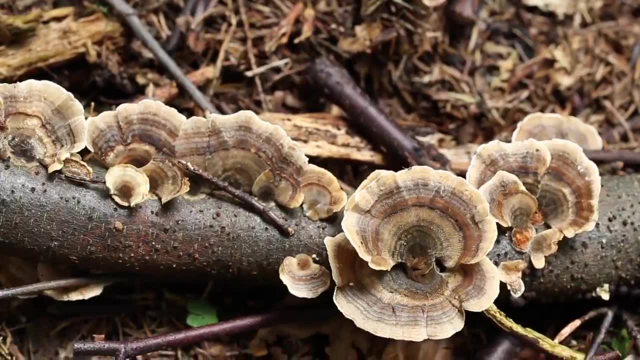 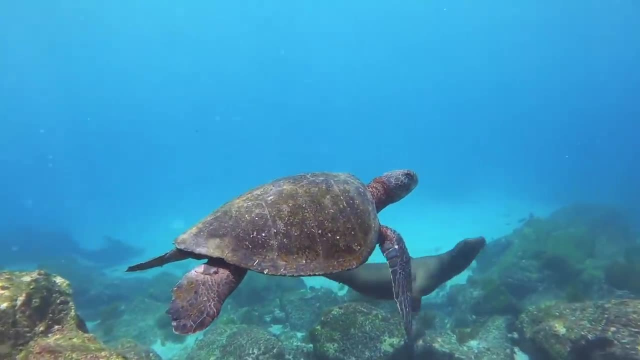 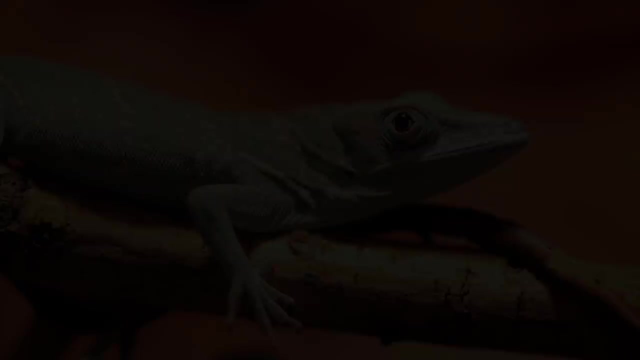 rocks. for creatures with no natural hard parts or which live far from the kind of environments that favor preservation, the odds are stacked against them. paleontologists estimate that less than 0.1 percent of all species that have ever lived have become fossils, and far fewer of those fossils have actually been found. 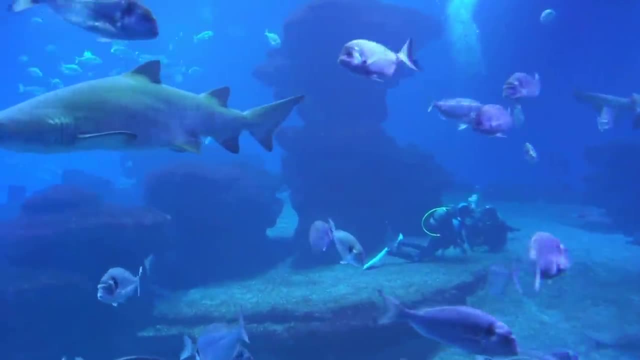 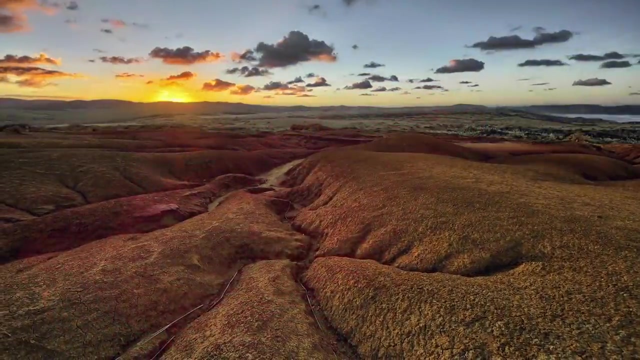 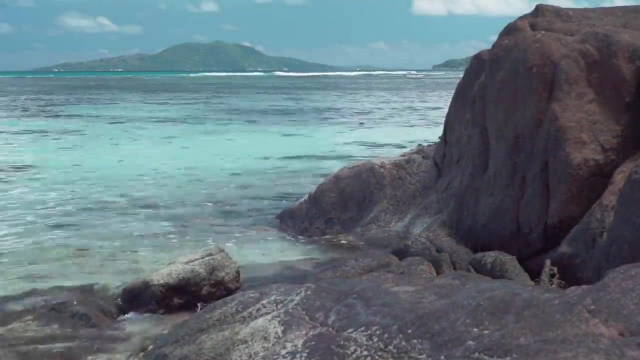 nevertheless, and perhaps testament to the sheer number of organisms that have walked, swam, flew or slithered across the ocean to find a fossil that is still alive the earth. there is an astounding wealth of fossils to be found in our rocks. the very existence of a fossil record is what defines an entire eon of Earth. 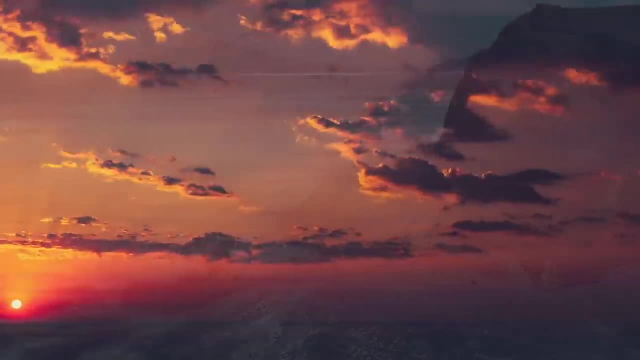 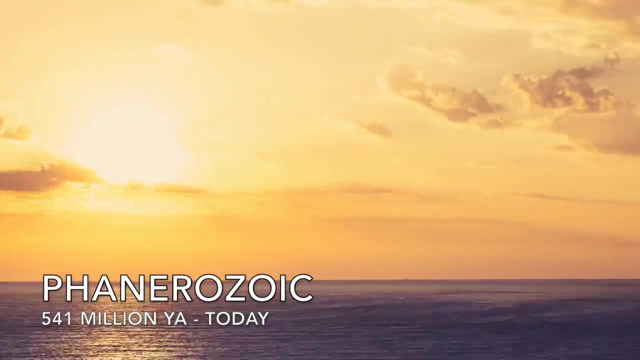 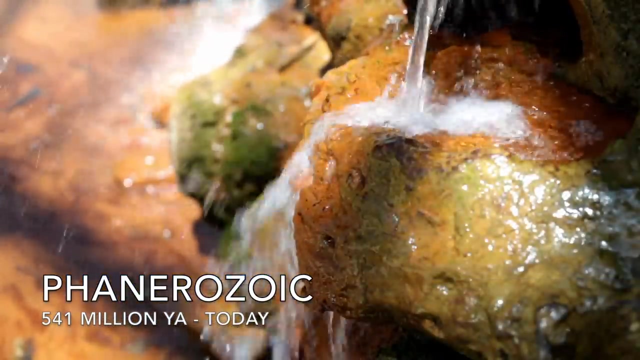 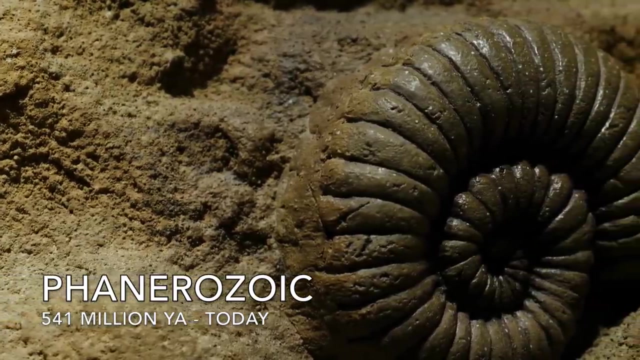 history. the phanerozoic from 541 million years ago to today is so named in Greek after the visible life within rock layers dating to this time. there are bones, teeth and shells, but also the impressions of trees and leaves and, in especially rare cases, footprints, fur and feathers. 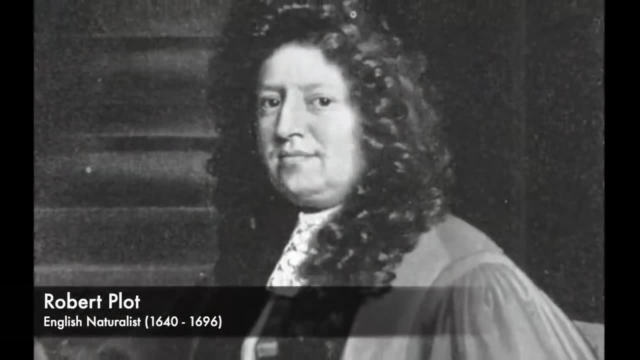 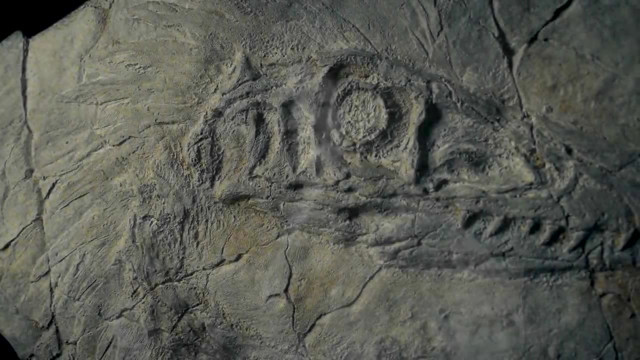 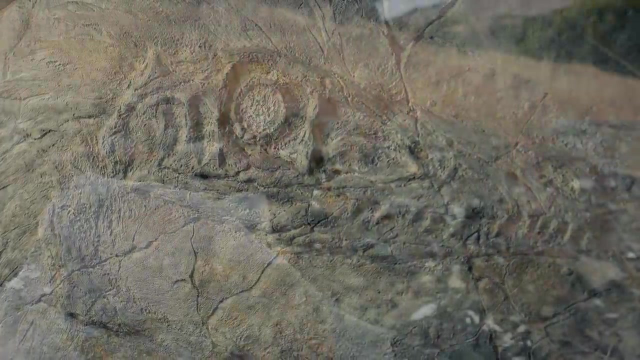 reverend Robert Plot was among the first to tap into this phanerozoic treasure and, in the centuries since, paleontology has grown to interpret life, evolution and environment on the of these fossil remains and tracing the fossils of the Phanerozoic back through. 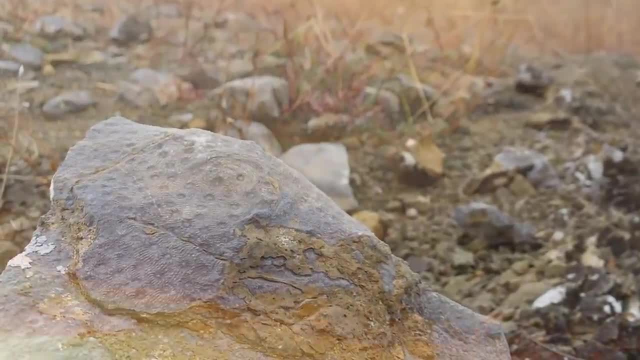 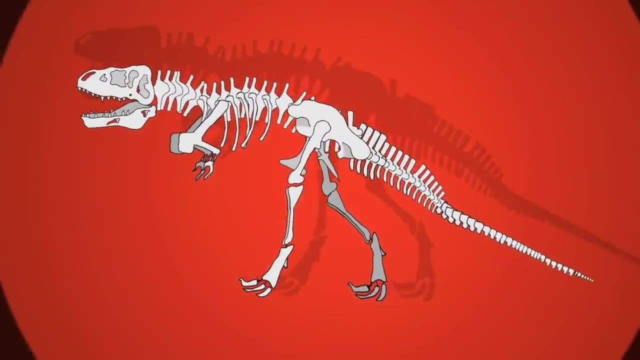 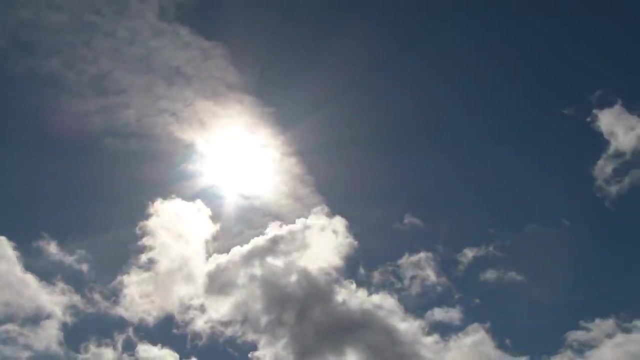 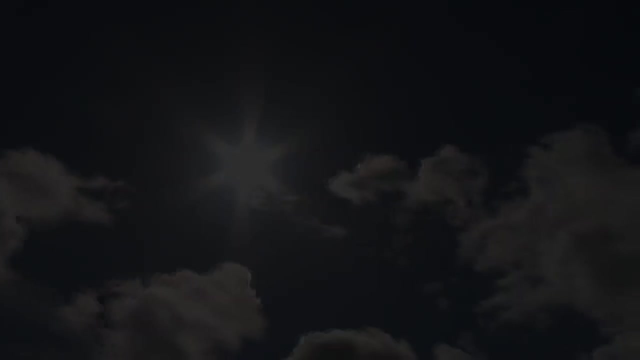 time, a pattern emerges of increasing simplicity. with increasing age, Large and complex skeletons give way to more rudimentary carapaces and modest shells, and then to first appearances, at least in the lowermost Cambrian rocks that mark the beginning of the Phanerozoic. the fossils just stop. 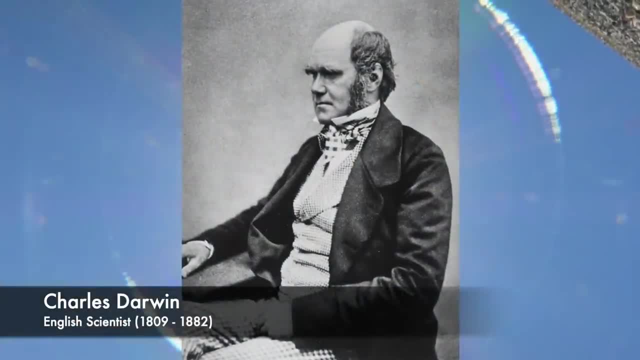 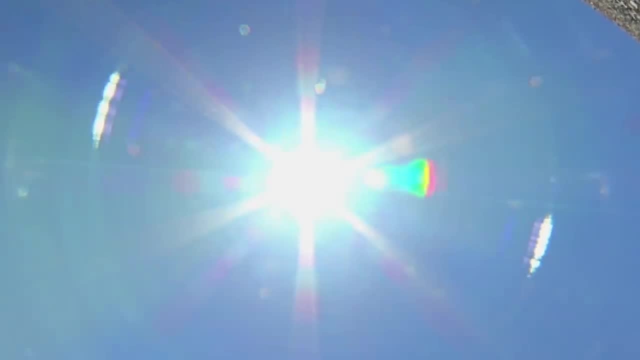 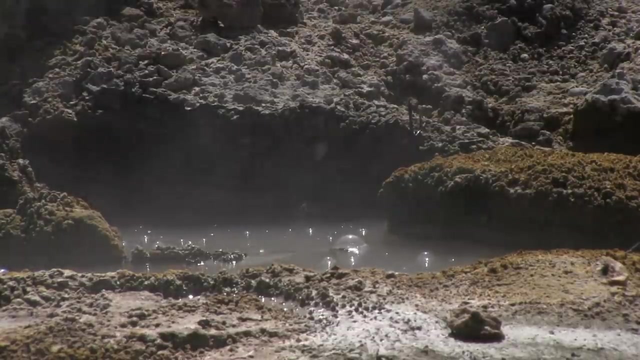 Charles Darwin himself remarked in 1859 upon the strange and sudden termination of our paleontological lifeline into the past. The problem of Earth's missing pre-Cambrian life is that it is not only the origin of life itself, but also the origin of our past. The pre-Cambrian life has come to be known as Darwin's Dilemma. 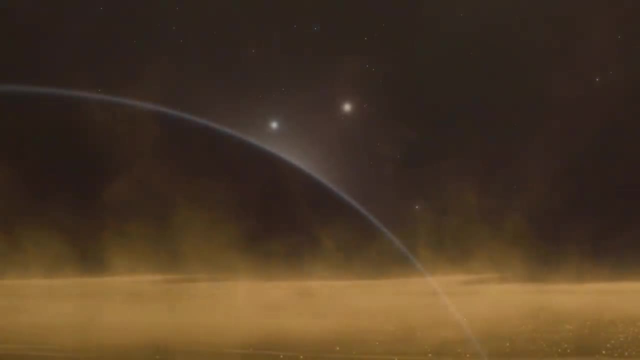 How could complex, hard-shelled life have seemingly sprung from nothing 541 million years ago? Where did all that complexity come from, and why can't we see it? The answer we know now is that we simply didn't know. The answer we know now is that we simply didn't know. 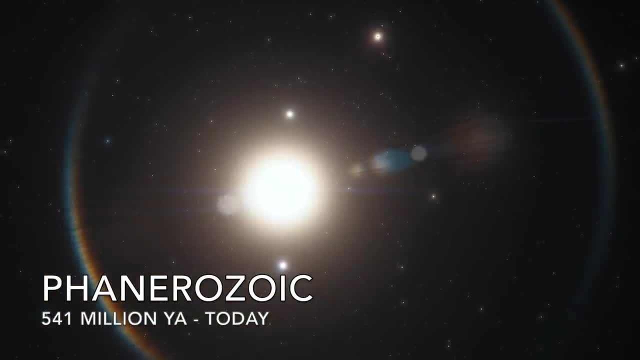 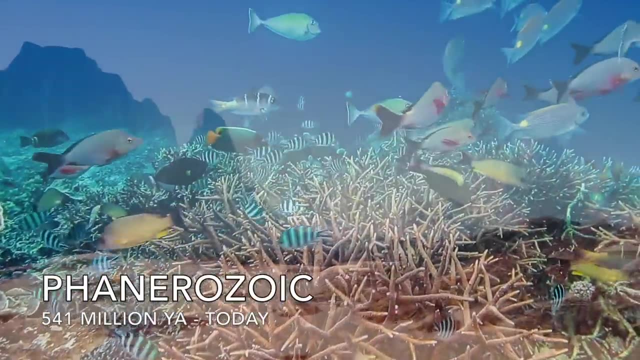 We were NOT made up of unlimited things. we were not made up of mountains��라 perma-solar beings, the people of the past life to come. We were able to experience life in a way that was more than we could ever imagine. We were not able to see life as much as we could have imagined. We were able to experience life as much as we could have imagined. We were able to see life as much as we could have imagined. We were not able to experience life as much as we could have imagined. 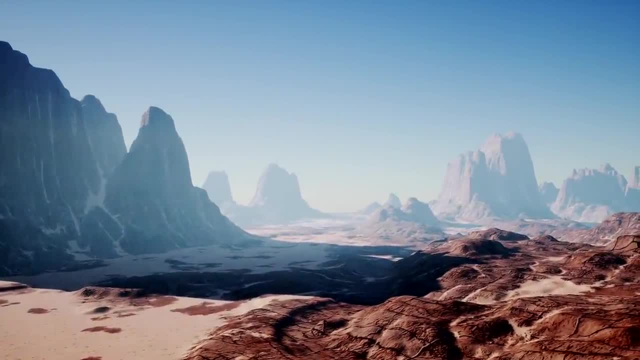 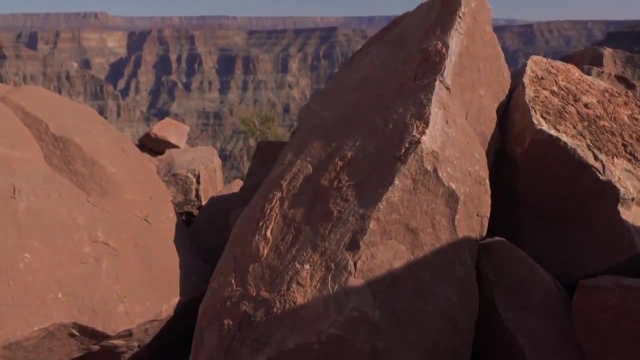 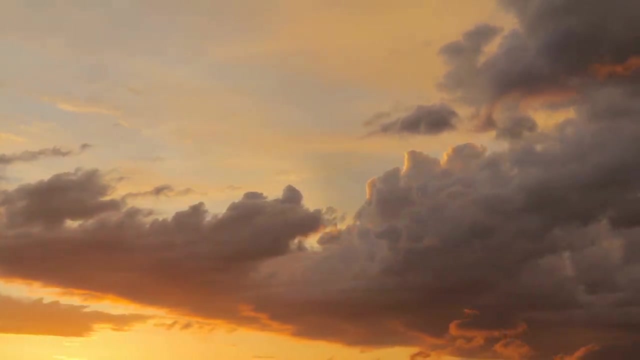 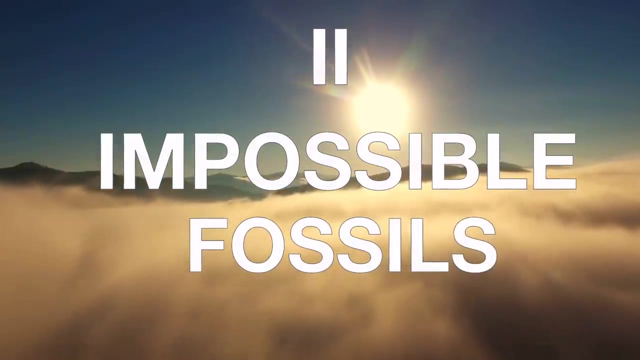 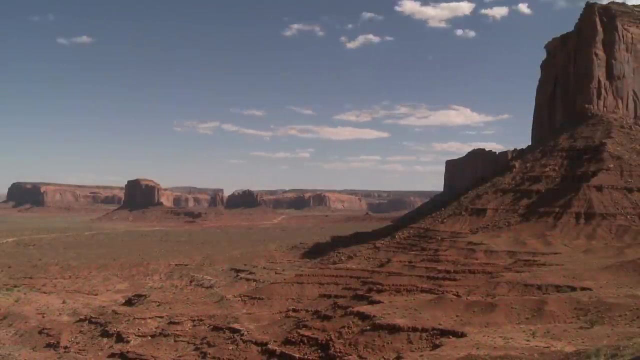 we know now is that we simply didn't know where to look. Against all possibility, there are impossible fossils lurking in rocks from long before the eon of so-called visible life. In the northwestern corner of Arizona, the Colorado River cuts deep through flat layer. 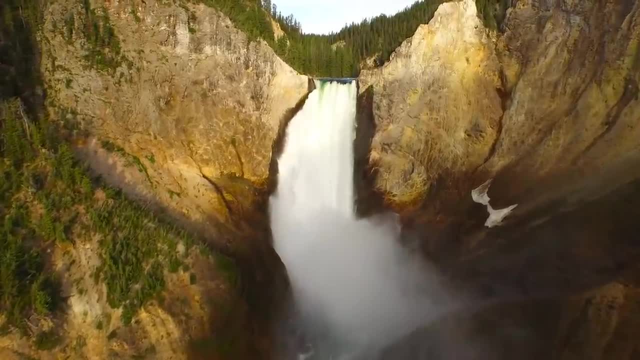 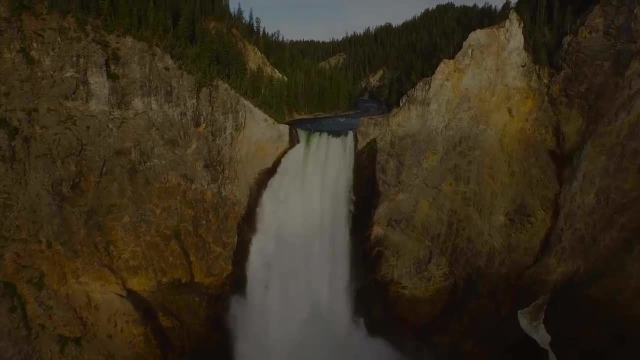 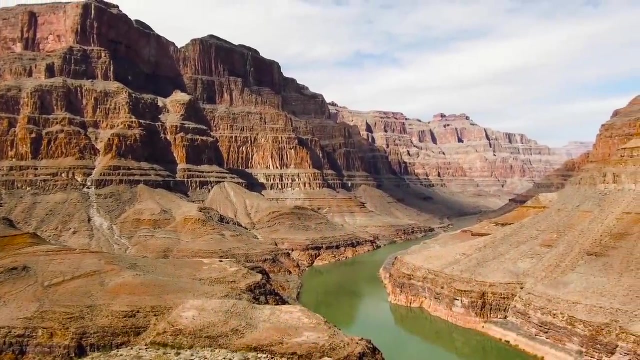 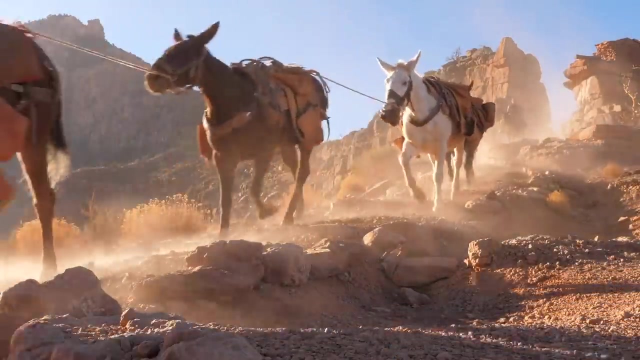 cake strata of the Phanerozoic, carving out one of the most magnificent geological features on Earth, the Grand Canyon. And on a cool autumn day at the end of the 19th century, the chief paleontologist of the US Geological Survey picks his way down the narrow switchbacking path, descending 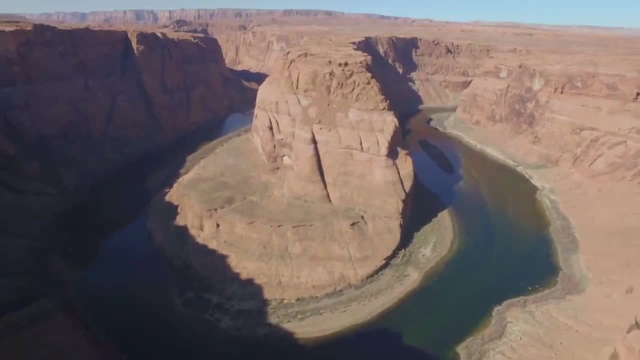 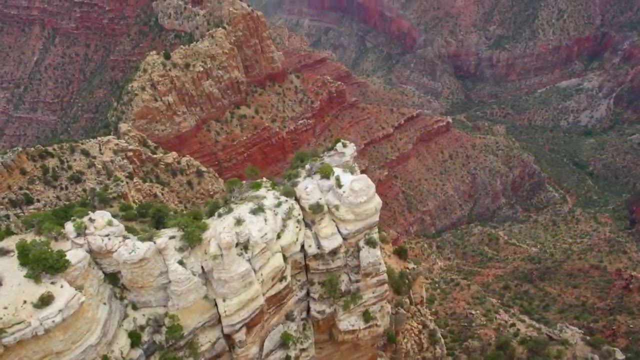 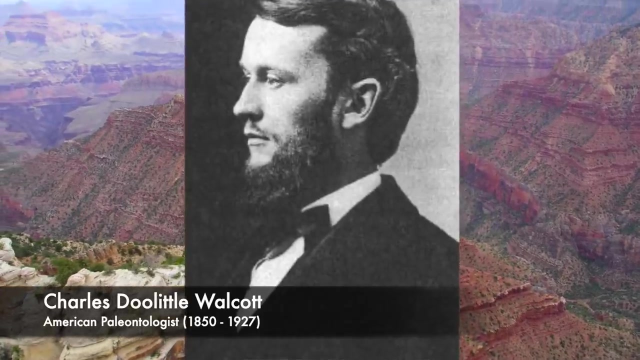 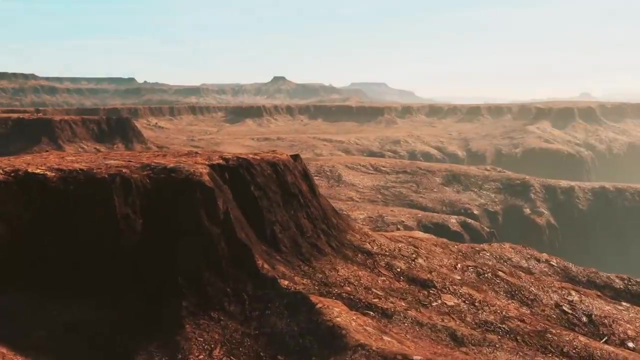 deeper into the canyon and deeper into time. Charles Doolittle Walcott Is a self-taught geologist. He began his paleontological career as no more than a professional fossil collector, And yet his eye for something new and special among the ordinary proves the key to his academic 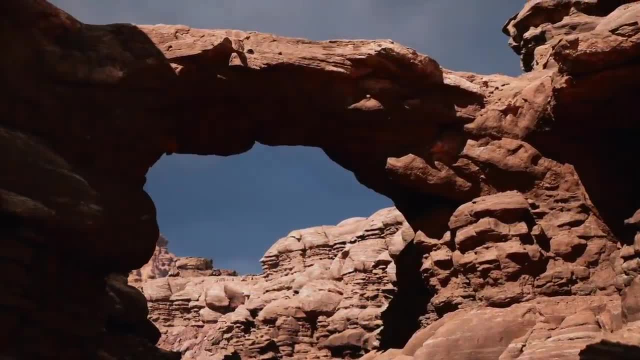 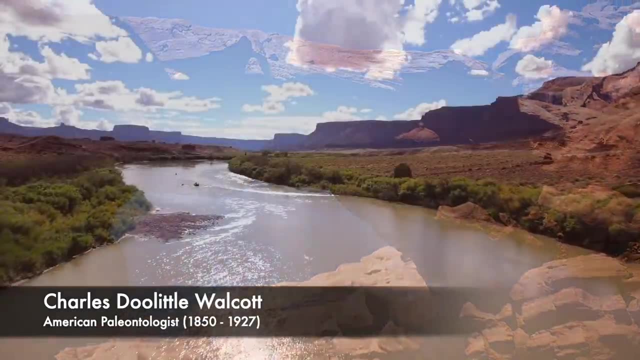 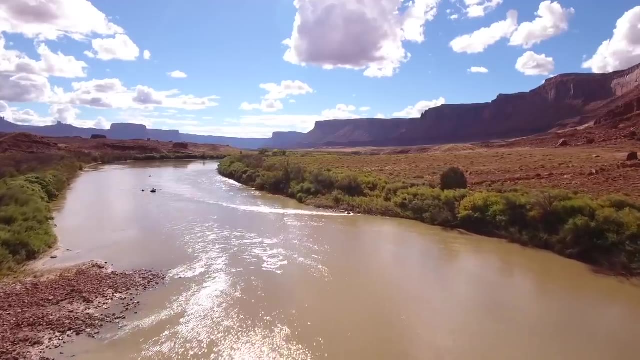 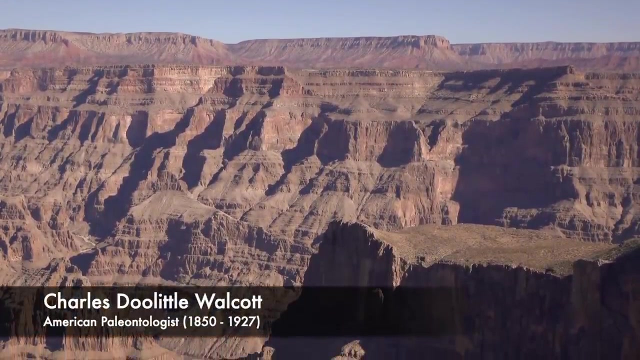 success. Never having been told what should or should not be geologically possible, he looks at the world with fresh, unbiased eyes, Seeing things that his contemporaries are wont to overlook. Descending into the cool, shadowy depths of the Grand Canyon, Walcott spans thousands. 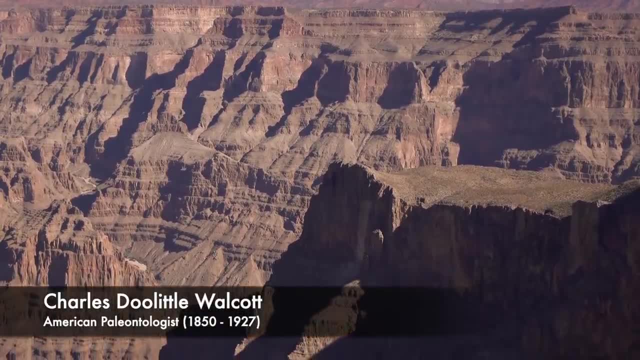 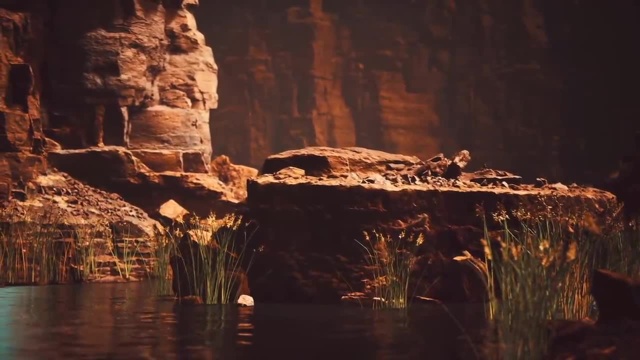 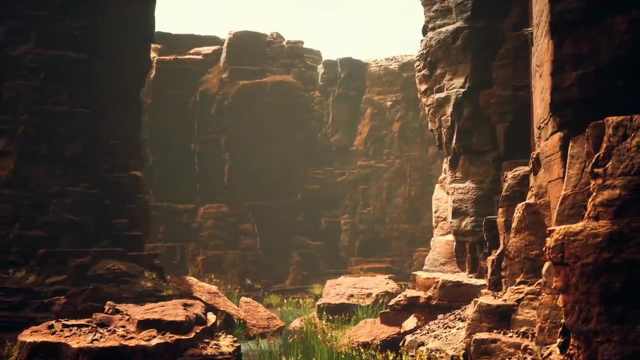 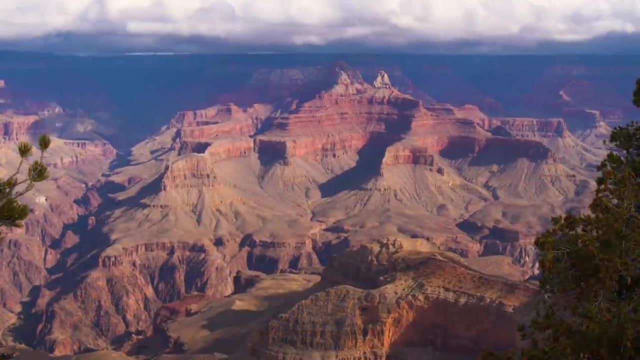 of years, with each downward step, Until near the chasm's floor, a single stride suddenly transports him 200 million years deeper into the past. He has crossed an unconformity, a sharp boundary in the rocks, marked not by gradual deposition but by ages of erosion. 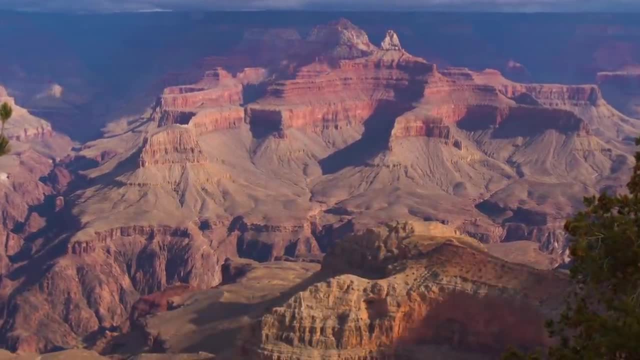 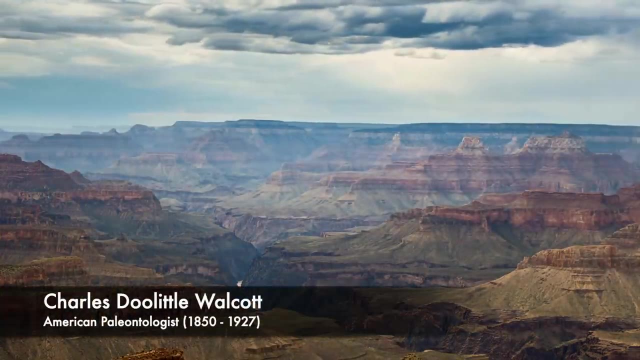 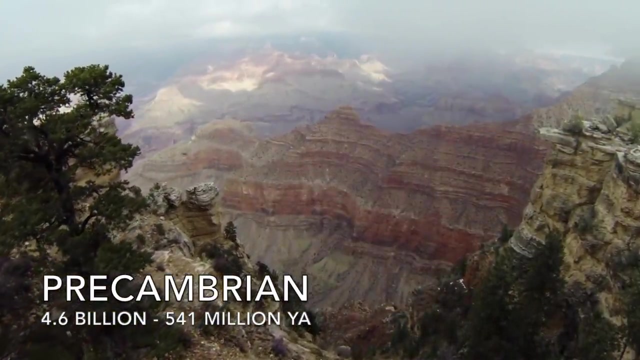 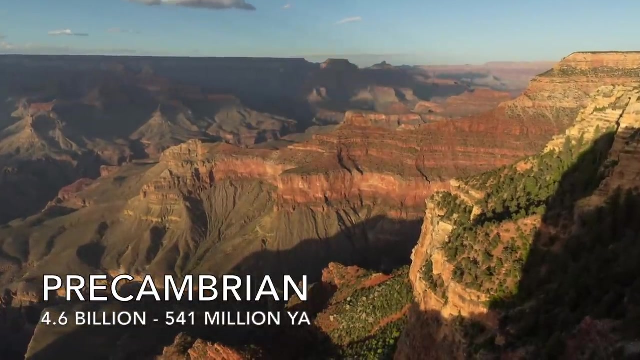 In this case, 200 million years of time have been lost. Walcott was first walking upon familiar Cambrian rocks, but is now adrift in the Pre-Cambrian among rocks that are some 750 million years old. These are the layers he has come to see. 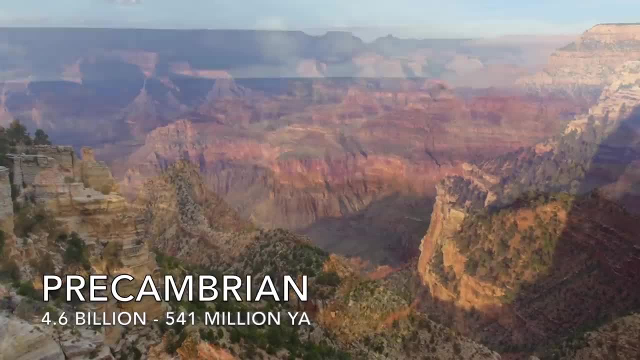 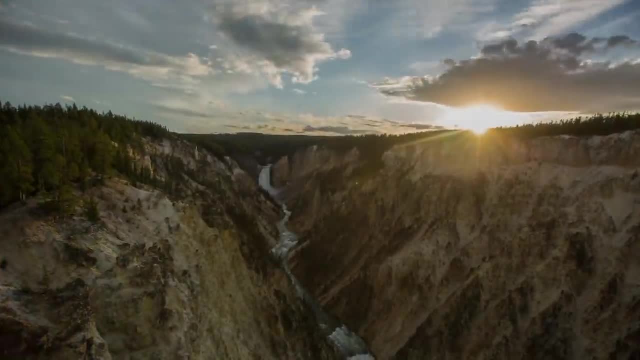 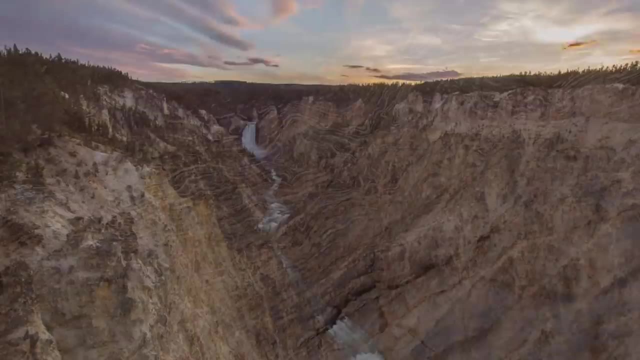 And with his collector's eye he is quick to assess the geology before him. His attention is soon caught by a strange pattern, Something he has never seen before, in rocks of any age Seen from the side. perpendicular to the rock's bedded strata, there are domed cabbage-like 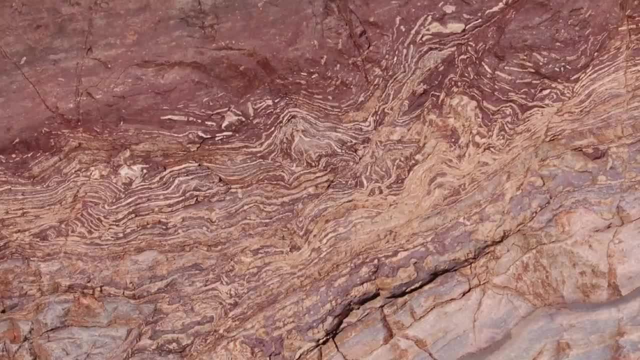 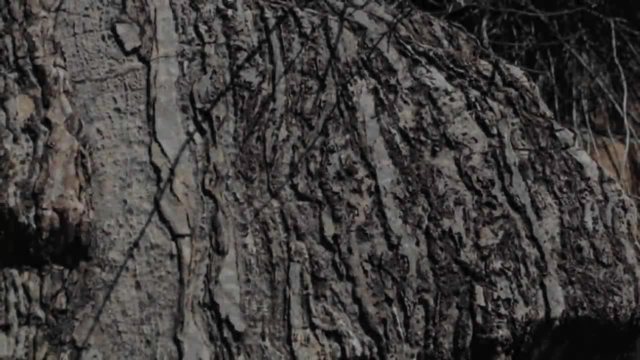 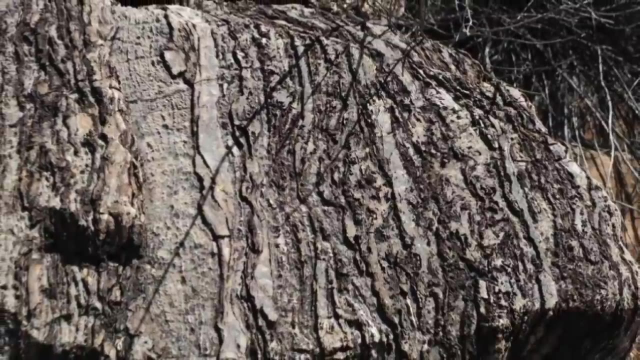 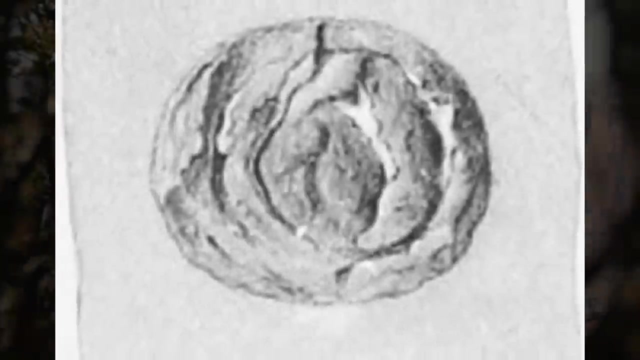 layers, Sometimes broad, sometimes tight and compact, Even pointed. When surfaces parallel to the bedding are exposed, the tight layers are successively cross-cut to form fine concentric rings. Without any comparison, Walcott considers what could have formed these curious structures. 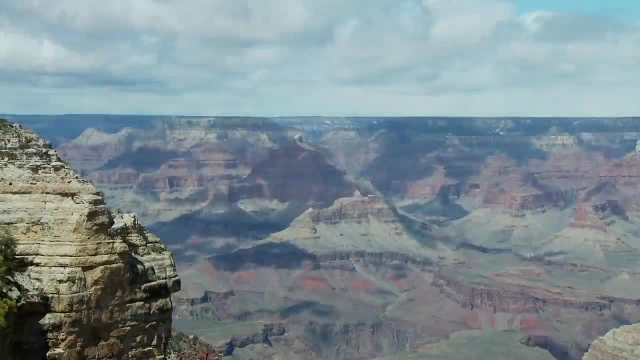 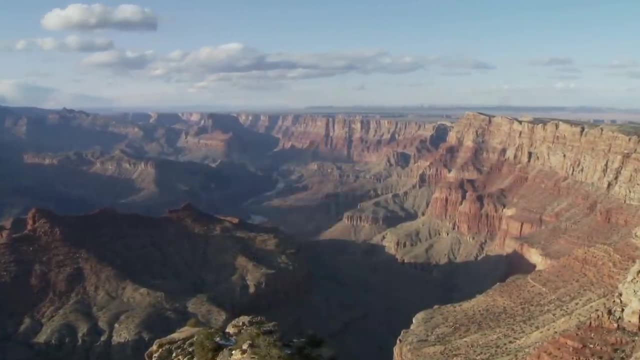 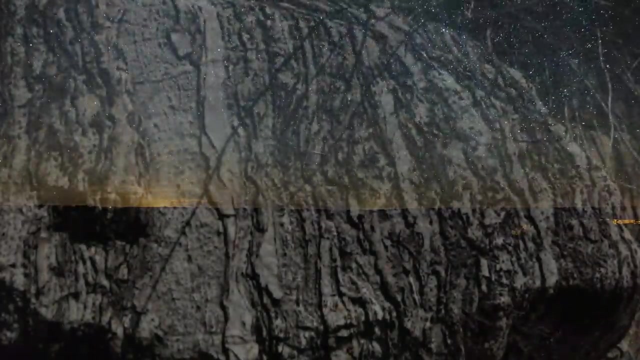 Their layering is much finer than his, Much finer than the grains of the surrounding rocks would seem to allow, And their shapes are not those easily formed by any physical processes. he knows. In his notebook, alongside their sketches, he posits that they could have been shaped. 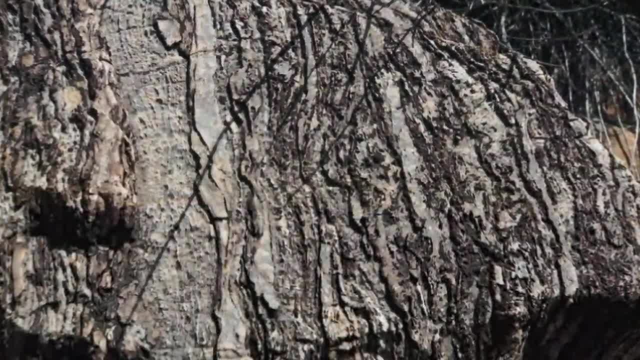 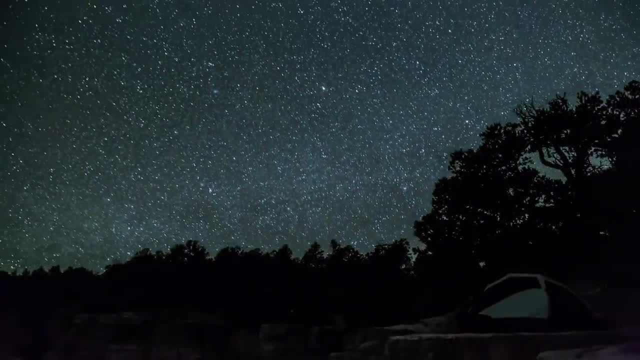 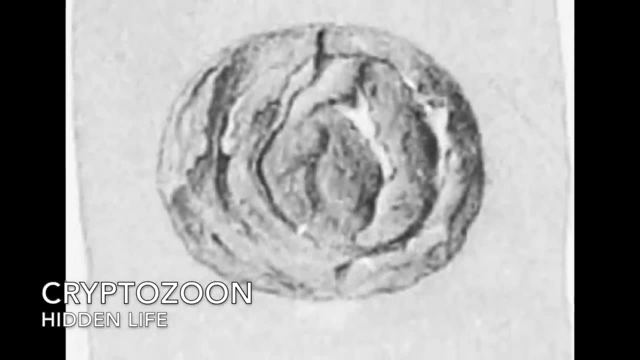 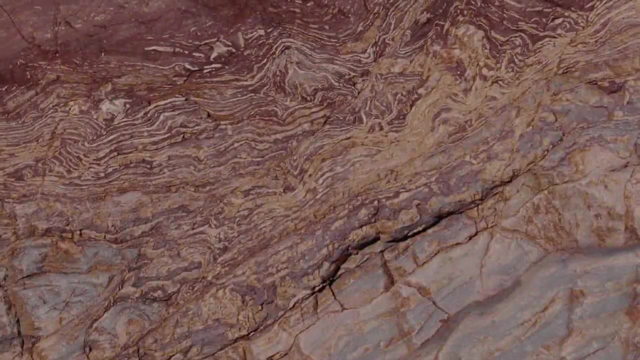 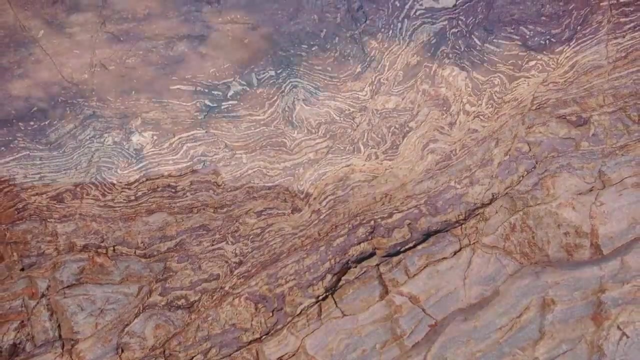 by some kind of ancient life, Although precisely what kind of life he isn't sure. He gives them a new name, Cryptozoon, Meaning hidden life And reflecting the many questions still surrounding these strange formations. Many more examples of Cryptozoon were subsequently discovered in pre-Cambrian rocks. 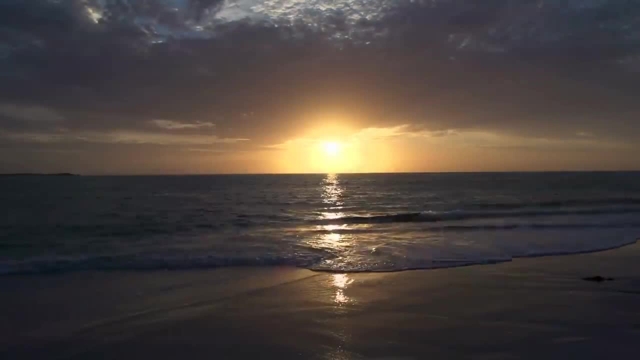 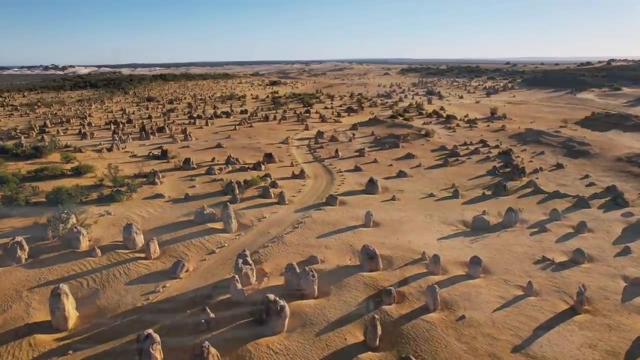 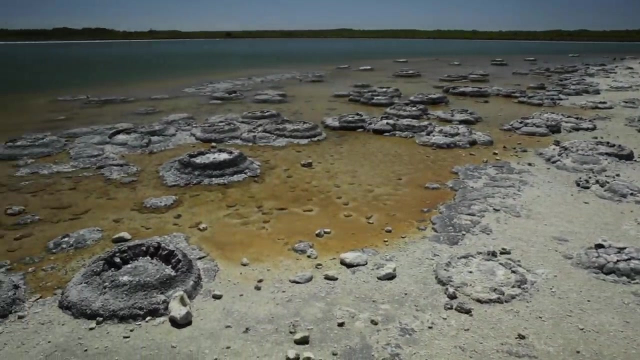 But it wouldn't be until the 1950s, long after Walcott's death, that this hidden life would be revealed for what it really was. In several salty bays of Western Australia, rocky blobs cluster in the tidal shallows, And ecological analysis revealed these smooth domes to be composed of layer upon layer of 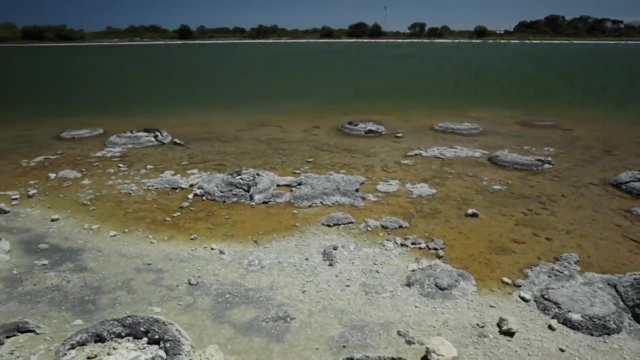 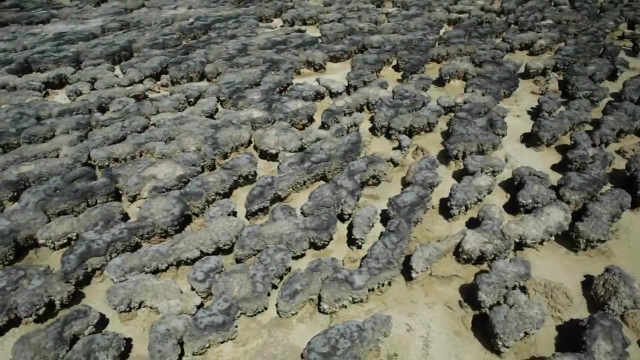 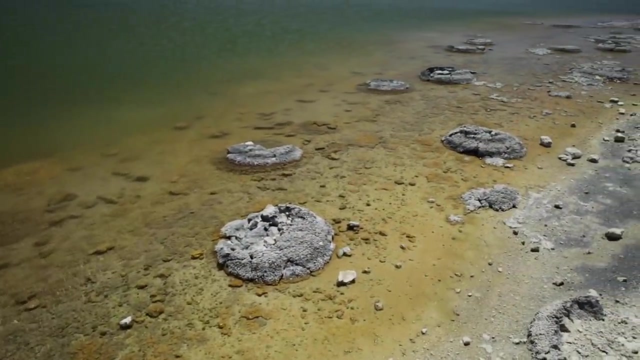 fine sediment and organic matter And in the uppermost layers, photosynthesising cyanobacteria reach for the sun. These are stromatolites, Multilayered microbial tower blocks, which only the uppermost levels are occupied. 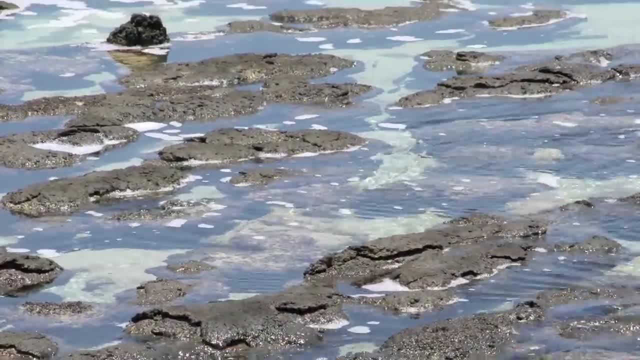 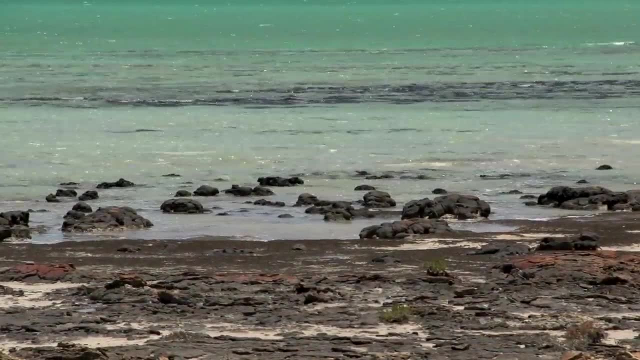 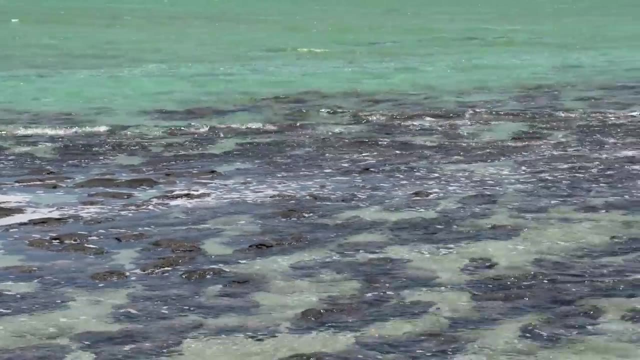 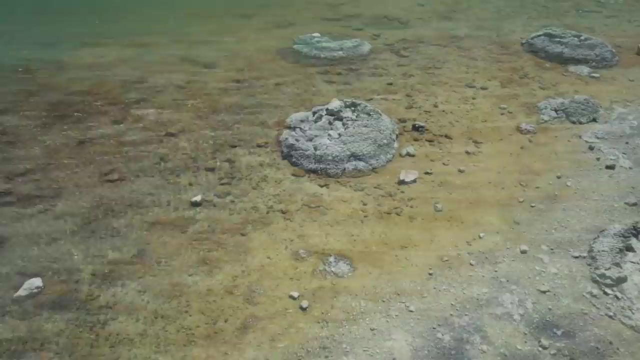 They grow with geological slowness driven by the photosynthetic need for the sun. Tidal waters wash fine sediment over their tops and the cyanobacteria must form a new layer on top if they are to survive. Shaped by tidal ebbs and flows and the gentle action of waves in the bay, the layers are. 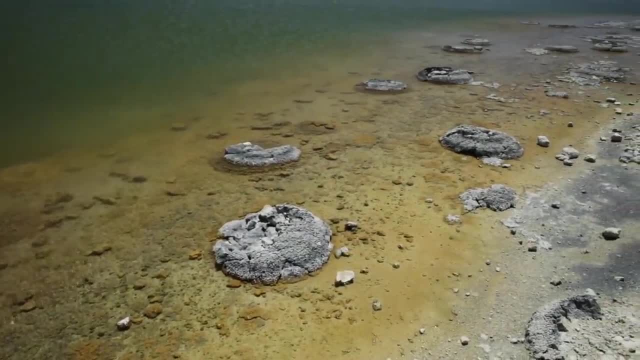 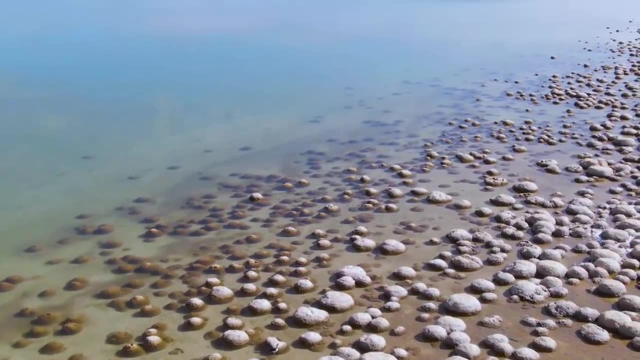 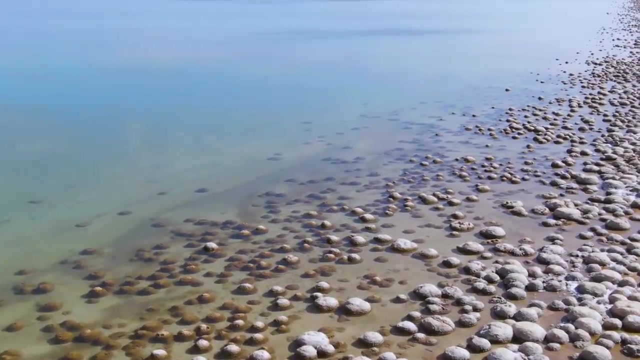 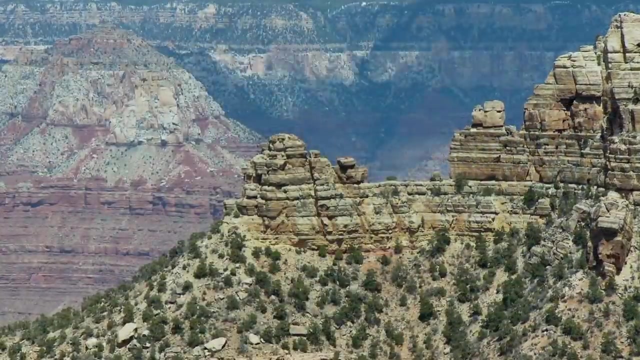 moulded into individual domes, cauliflower-like in cross-section and concentrically ringed when eroded flat. These living stromatolites are a perfect match for the Cryptozoans Walcott found in the Grand Canyon, And just as the modern domes are formed by life, so too are their petrified Precambrian. 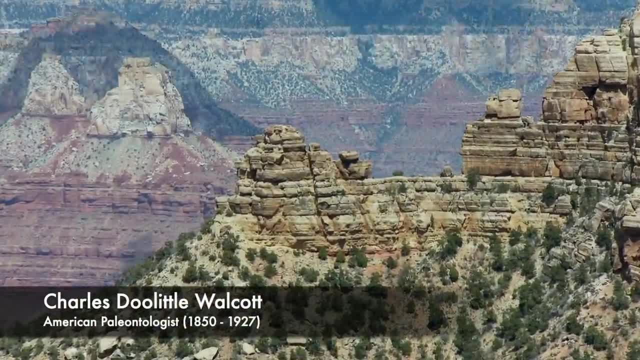 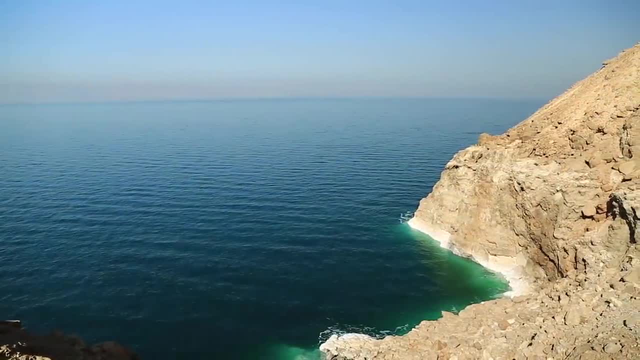 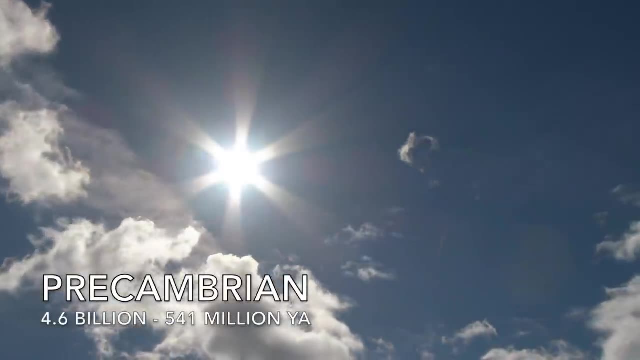 twins, Charles Doolittle Walcott, had unwittingly found the first evidence for life before the Phanerozoic, Proving Darwin's assertion that life did indeed exist in the Precambrian and offering a hint as to why it was still hidden to us. 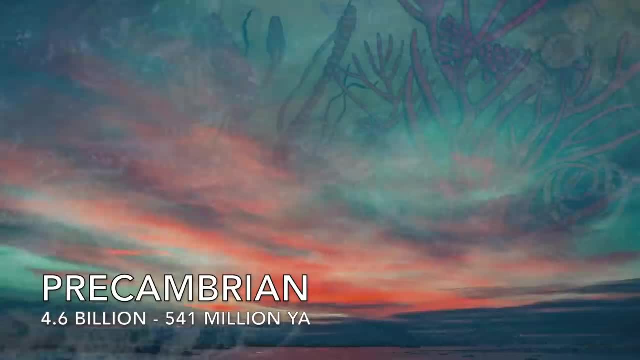 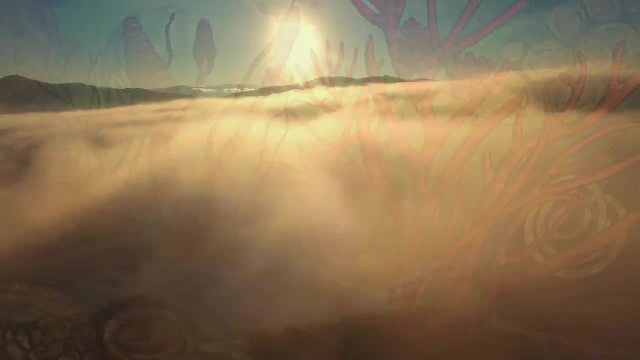 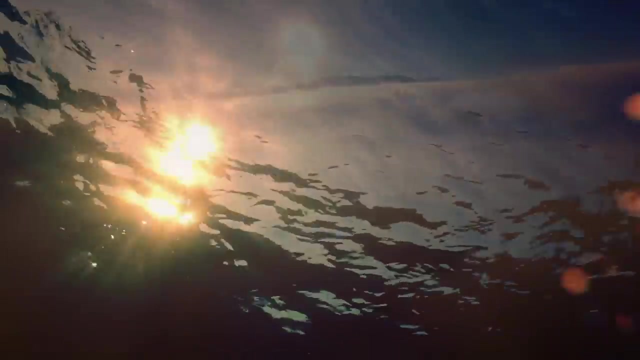 Quite simply because it was too strange to be believed. The Precambrian Twins. Since the mid-20th century realisation that the Precambrian fossil record does indeed exist – if only we know where to look – protozoic paleontologists have had to challenge their 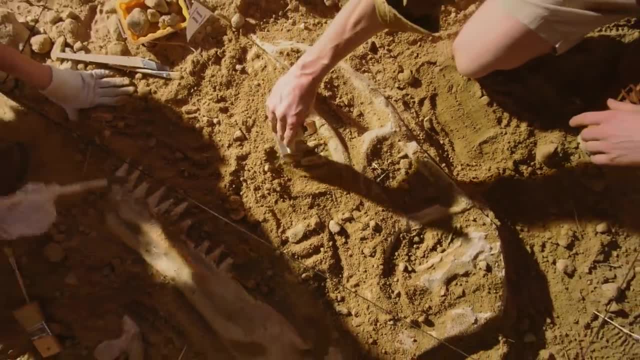 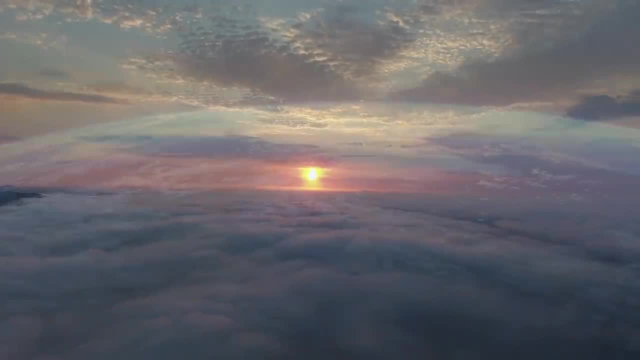 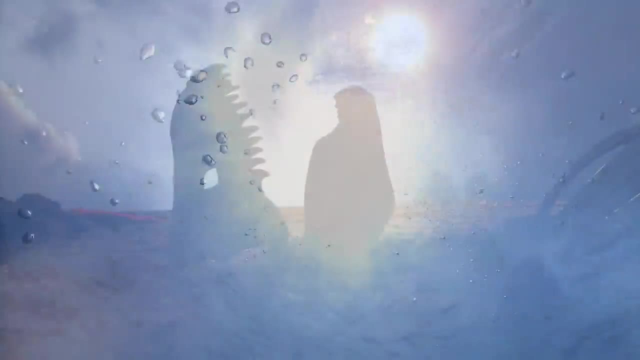 assumptions and put aside their biases about where and how some of the earliest forms of life might be preserved. Now the scales have fallen from our eyes and the jewels of the Precambrian are revealed. We may not find bones or teeth, or even simple shells. 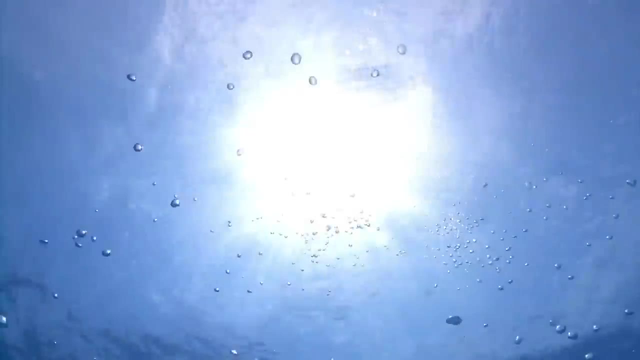 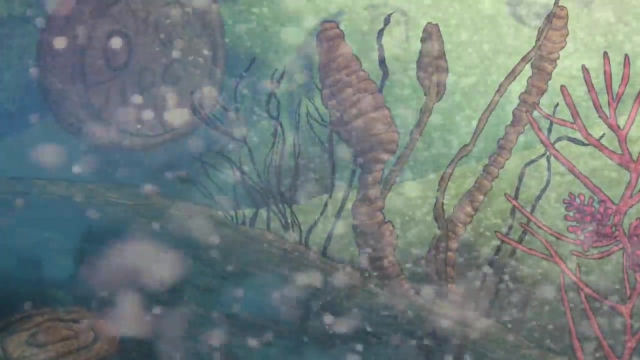 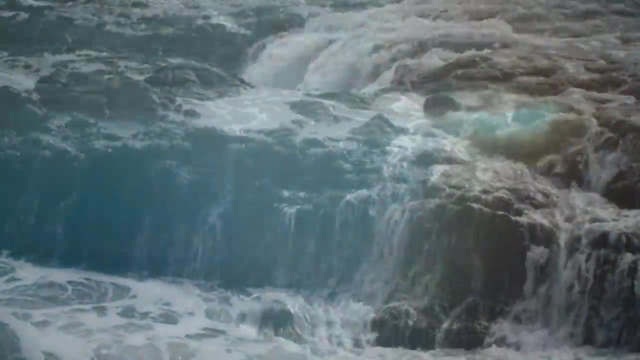 But we do find hints and clues of the life that existed before this mineralised protection, When the stage was set for this complex life to find its figurative feet. It may seem an impossible task to preserve a soft, squishy organic body in the face. 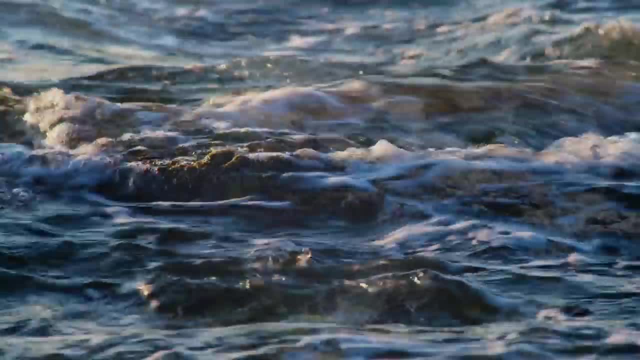 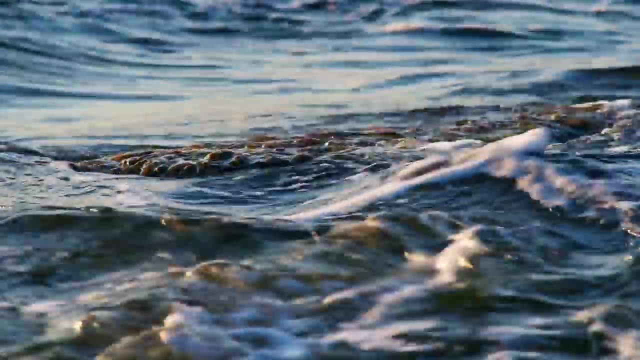 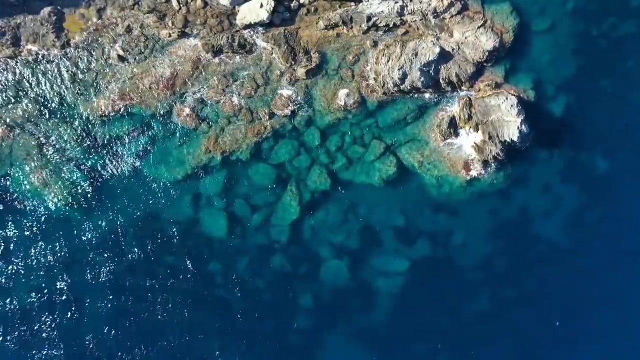 of biological recycling. But, as stromatolites have shown us, there are certain quirks of rock formation that allow even microscopic bacteria to be preserved throughout eons. In this case, sufficiently large communities of tiny organic organisms are able to exert enough influence on their local environment that the normal processes of rock formation. 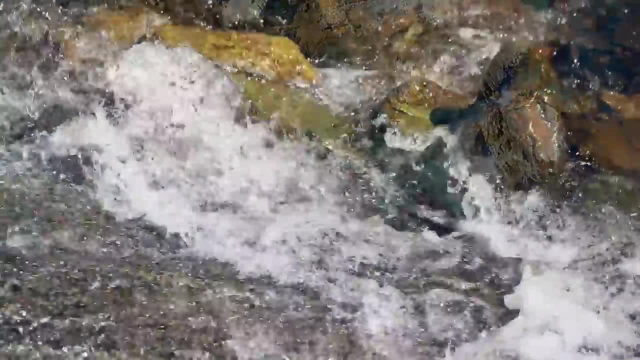 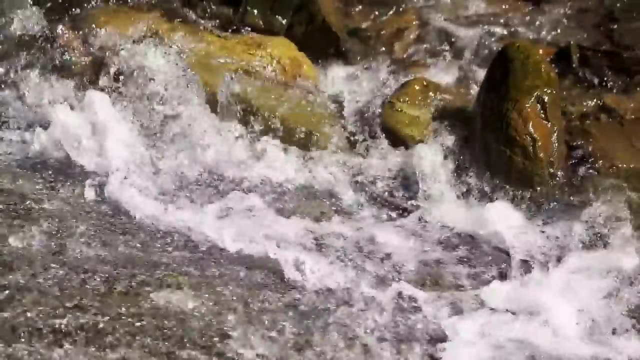 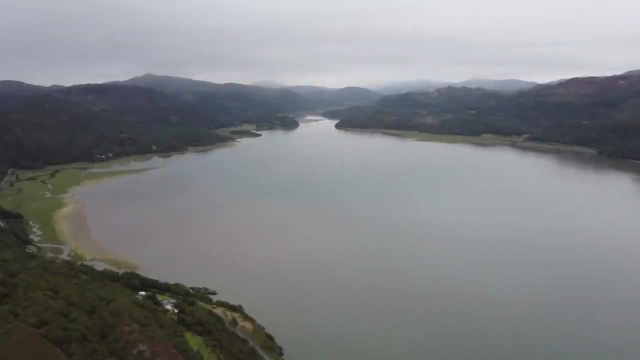 are subtly altered. With a thorough understanding of the kinds of structures life can build today, we can search the rocks for such traces as well. For instance, tidal estuaries are ideal habitats for microorganisms that don't mind the brackish. 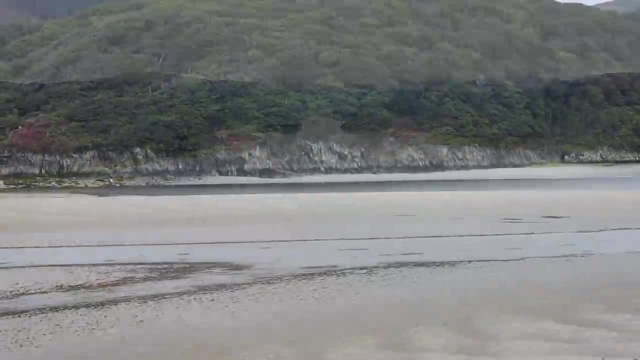 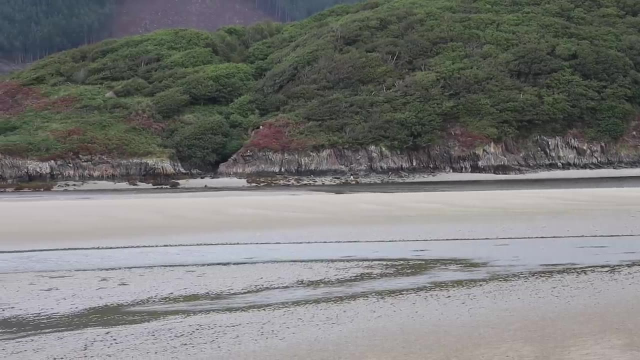 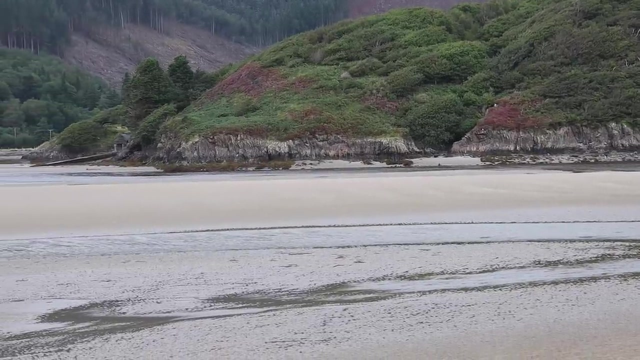 part-salty waters that wash over them. Nutrients delivered by the river are deposited, along with fine sand and mud, in shallow tidal waters that are protected from the worst of the battering waves. Here, vast layered communities of microbes can grow on and in the sediment spreading. 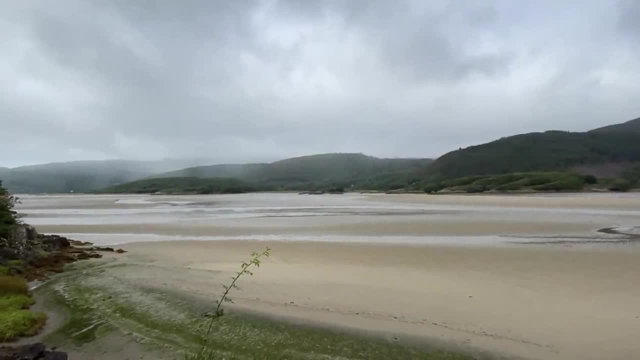 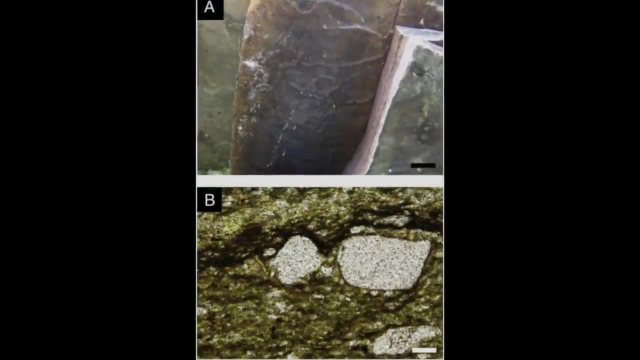 out to make the most of the sun's rays. Even if the conditions don't contrive to build stromatolite tower blocks, these biomats can still leave a trace in the resulting rocks. Their surfaces become tufted and wrinkled by the action of water on their organically. 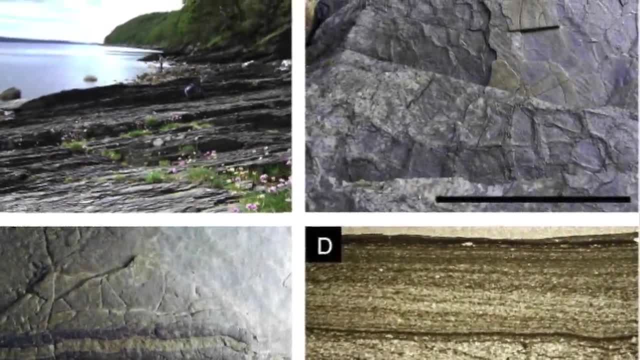 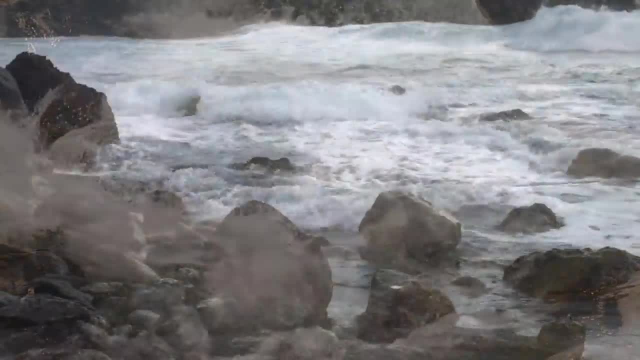 woven fabric. As the delta streams shift or storm surges dump new sediment on top, these tufts and wrinkles are locked in place and the unique chemistry of these aqueous environments tips the balance of petrification. This is the end of this video. 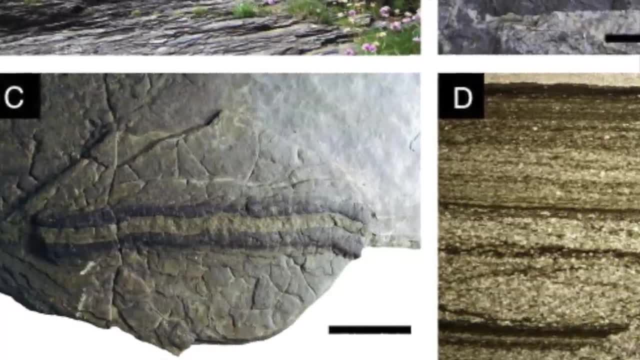 Thank you for watching. Please subscribe and like this video. You can also leave a comment below, And if you want to see more of my videos, then be sure to hit that subscribe button And I'll see you in the next video. Bye. 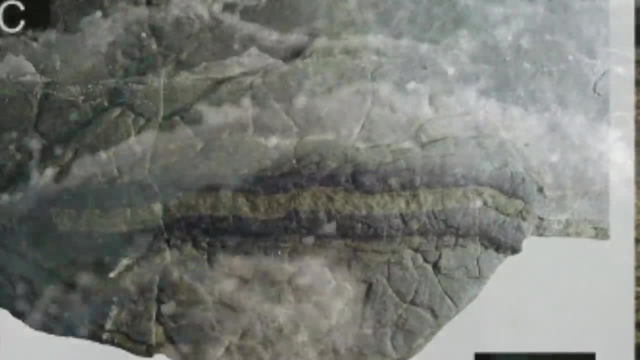 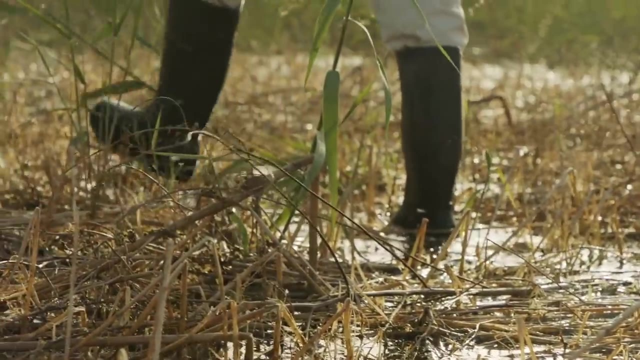 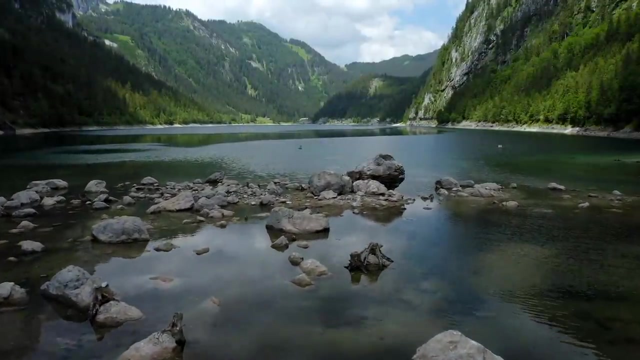 Today, pre-Cambrian paleontologists scour the top and lower surfaces of rocks for these shadowy hints of wrinkled biomats. Searching at sunset when the sun is low, reveals intricate patterns formed by sun-hungry biological fabric many hundreds of millions of years ago. 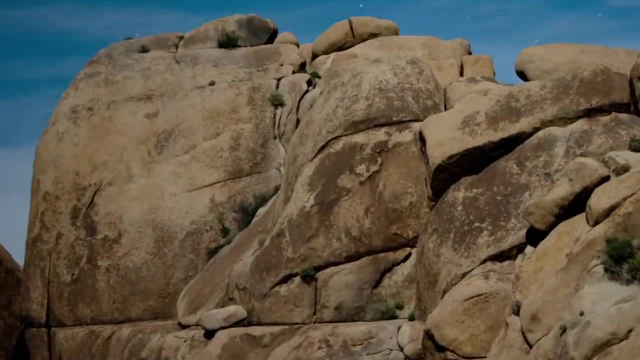 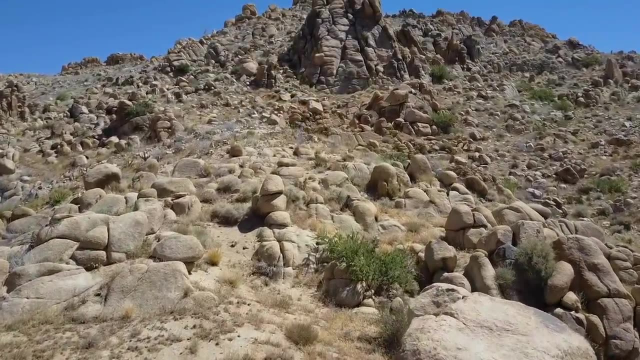 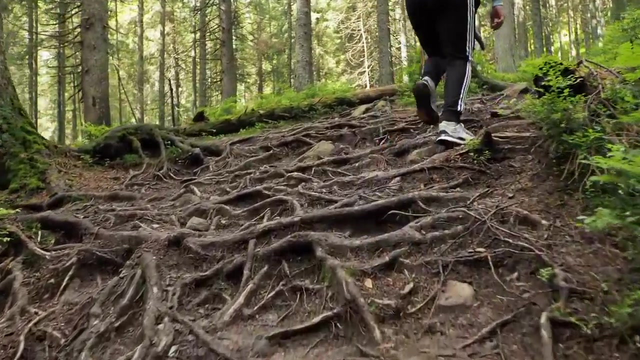 For many paleontologists today, turning over a slab to find its bottom surface decorated with fine tufts and wrinkles formed by ephemeral microscopic organisms is a thrill akin to discovering a dinosaur footprint. It is a brief moment of time miraculously captured for the ages. 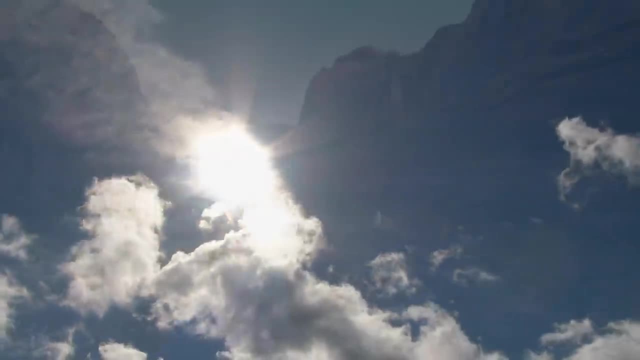 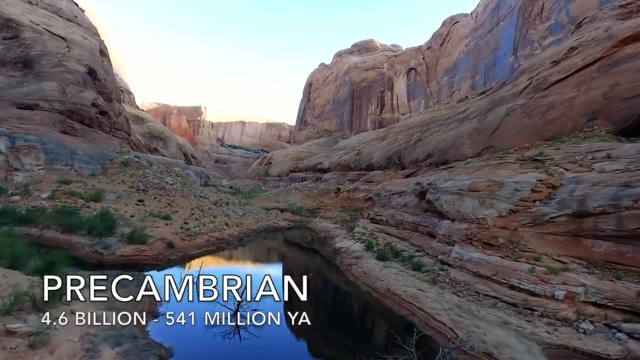 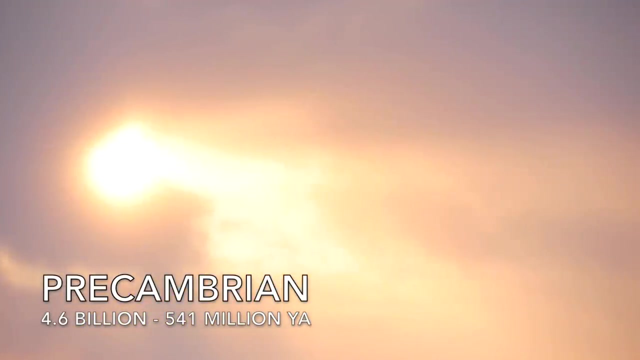 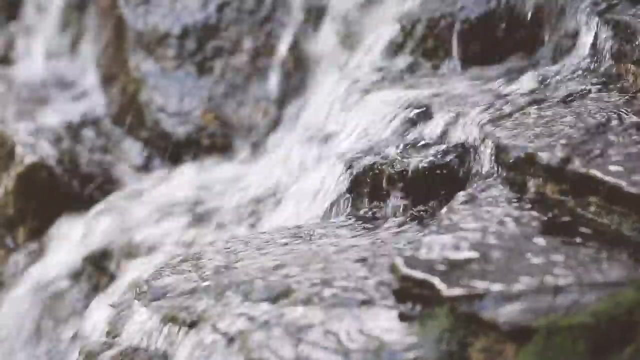 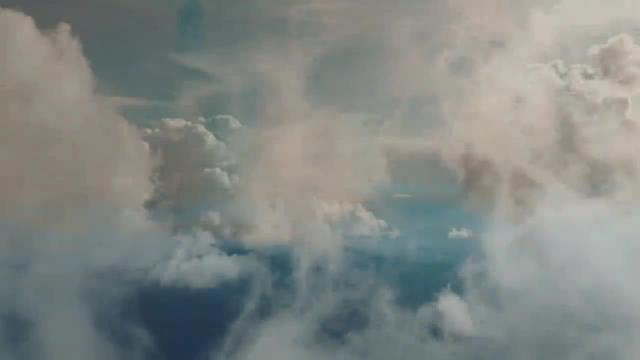 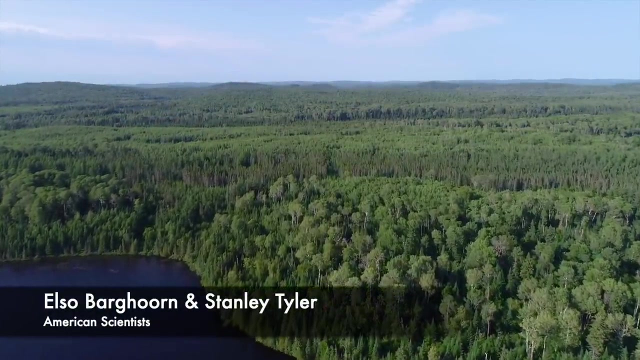 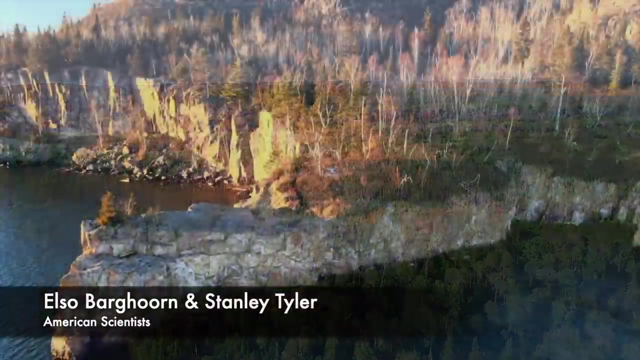 Geologists on the opposite side of the world were uncovering something even stranger. Elso Barghorn and Stanley Tyler investigated curiously carbon-rich rocks from the Gunflint Range of Western Ontario. Layers of coal-like rock contain no fossils, but they hint that life was extremely abundant. 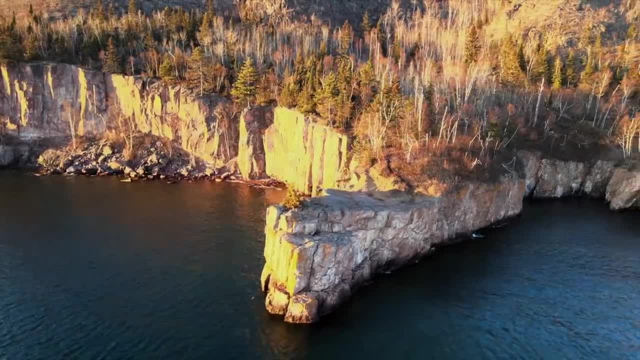 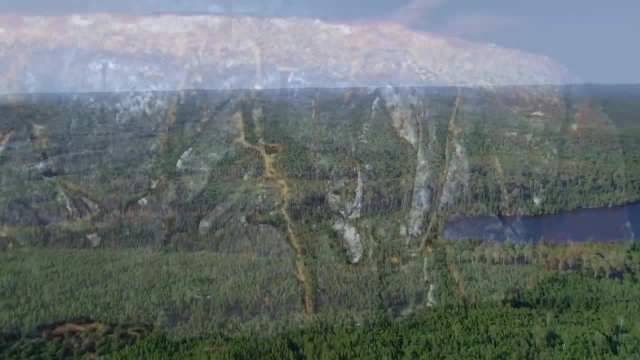 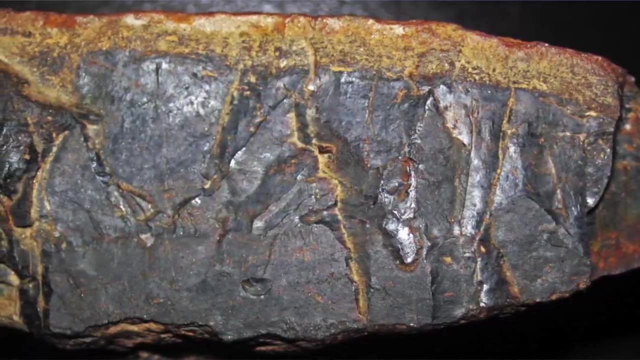 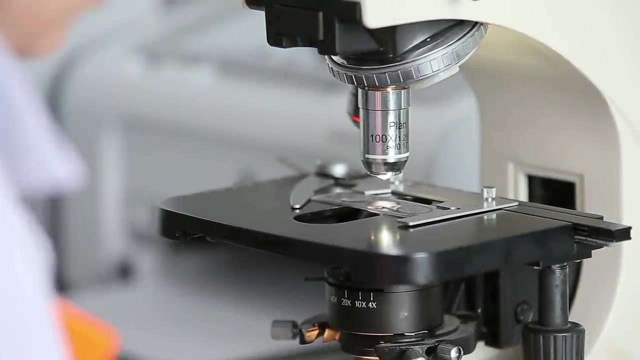 here abundant enough to accumulate carbon within the sediments themselves. Elsewhere, among the Gunflint rocks, they find dark, glassy chert, adding it to their pack for analysis when they return to the lab. Standard geological analysis often involves slicing paper-thin sections of a rock making. 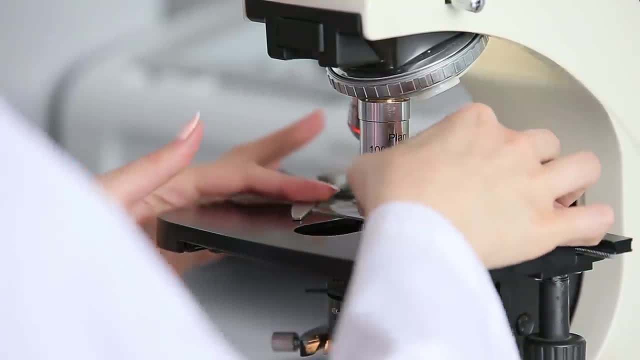 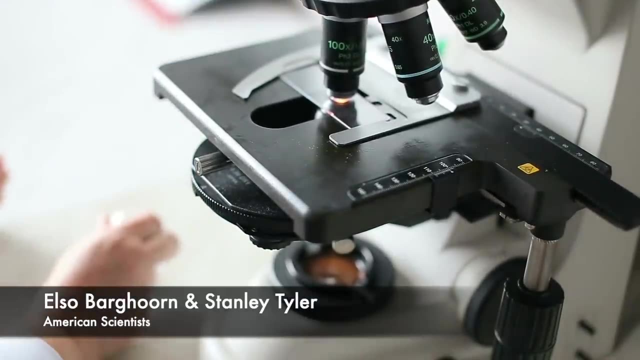 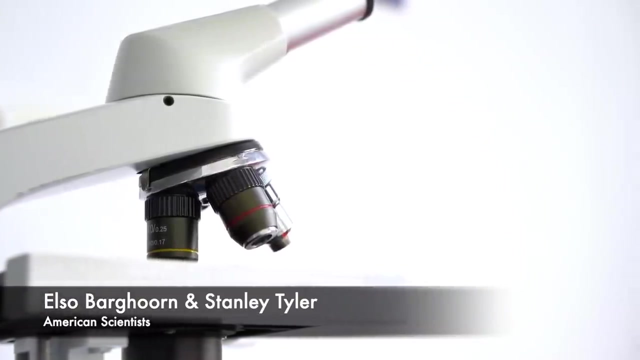 it thin enough so light can pass through it And experts can identify the minerals by their microscopic characteristics. But when Tyler and Barghorn discovered the Eucalyptus rock, they were surprised. They found something they didn't expect. Speckled all throughout the fine crystals of silicon dioxide. there are tiny grains. 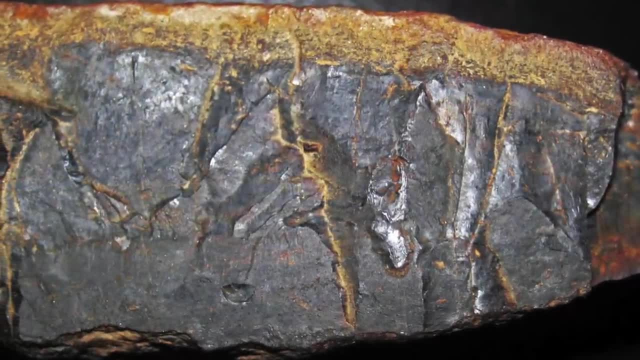 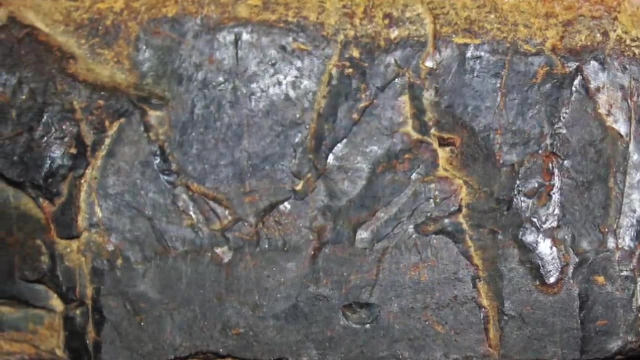 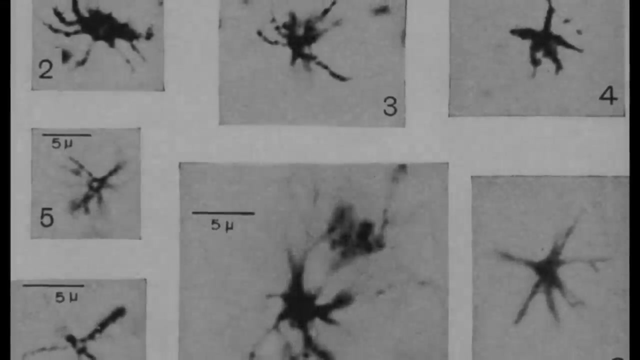 of carbon. It's this that is responsible for the chert's black colour. But in places these specks are gathered together in three-dimensional spheres, filaments and star-shaped groupings, each no more than around 10 microns or 100 microns. 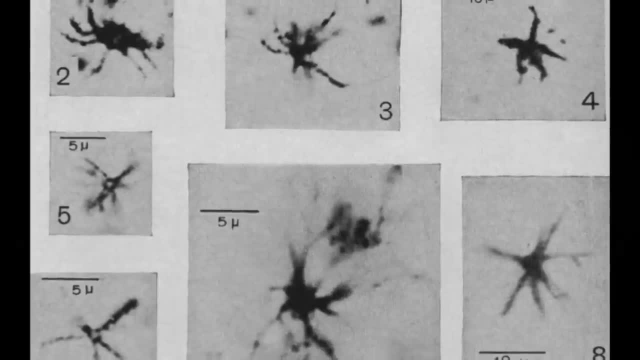 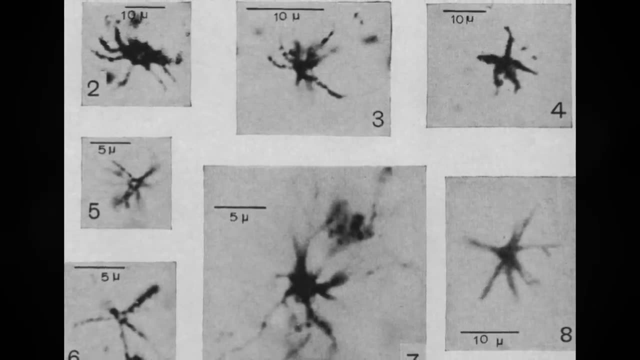 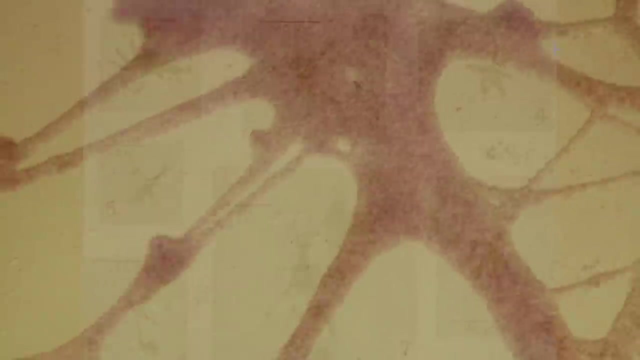 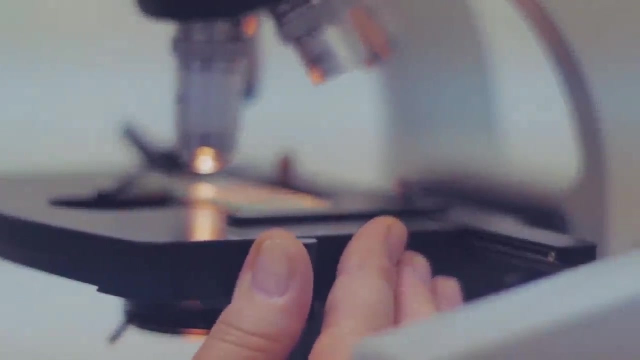 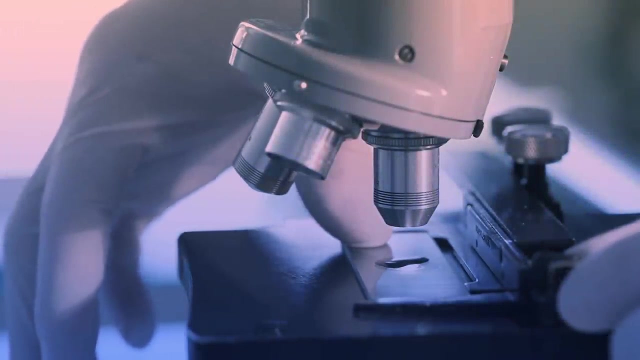 In both shape and size they resemble living microbes, But they are nearly 2,000 million years old. Could they really be biological in origin, Such delicate forms preserved for so long? For the last 70 years, since this incredible gunflint discovery, scientists have found: 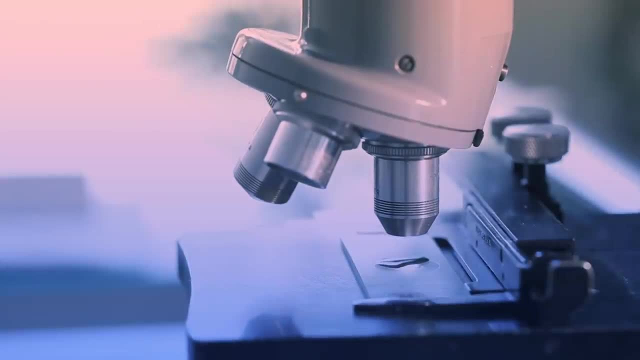 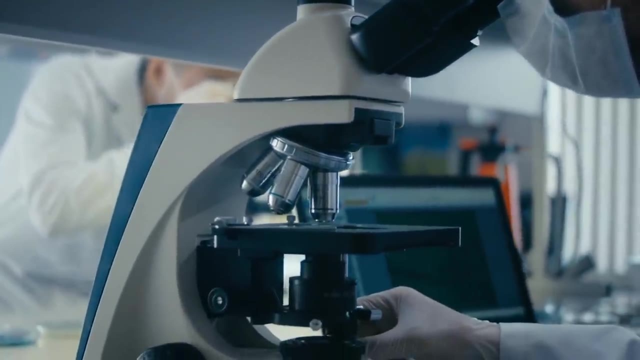 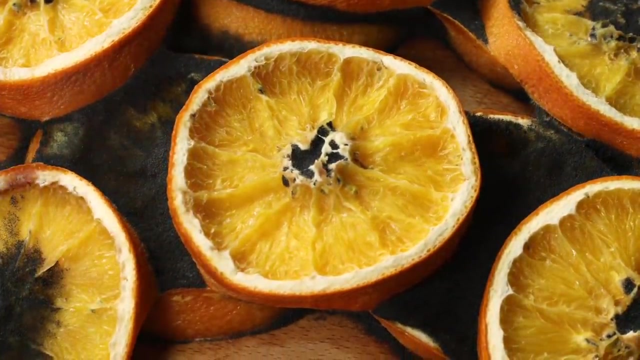 chemical and petrological justification for how such impossible fossils could come to exist. Remembering that fossilisation is a race between degradation and preservation, for the most delicate of organic structures to be preserved, then that preservation needs to happen at an unprecedented rate. 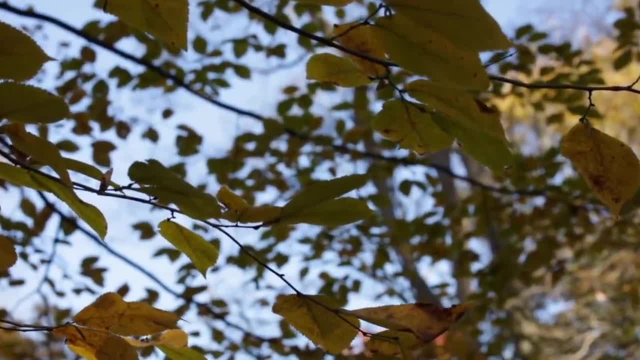 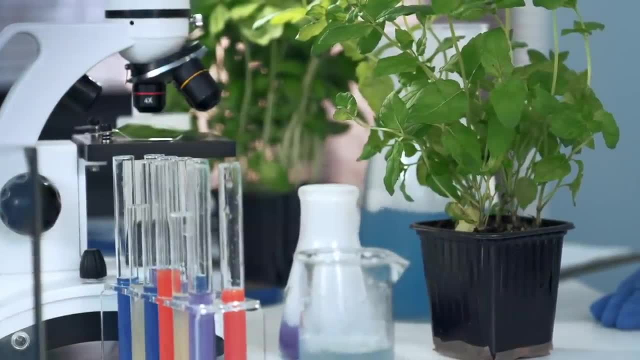 Indeed, the petrification of the fossil is the most delicate of organic structures to be preserved. The petrification process must begin while these cells are still alive. Certain quirks of chemistry more common in the exotic and undisturbed seas and lakes. 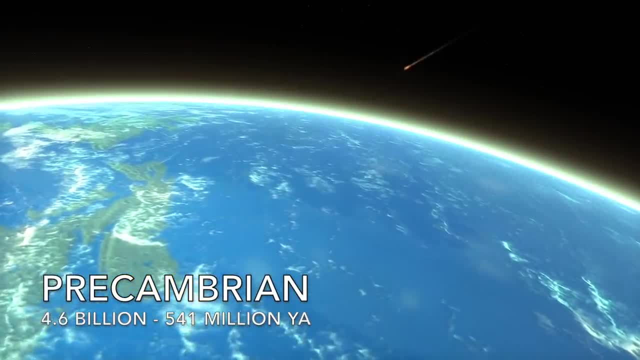 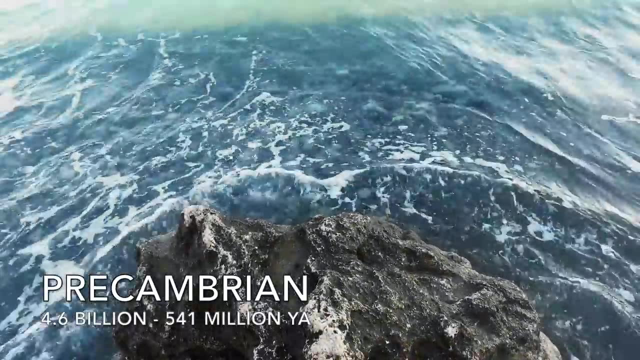 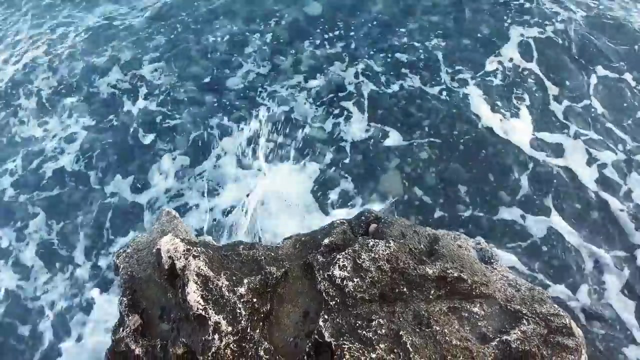 of the Precambrian can see certain mineral fluids become supersaturated in natural waters. Silicon dioxide or phosphate ions build up and are further concentrated by the microbes that inhabit the sea floor As they reach unsustainable levels and a kind of gel begins to precipitate, the luckless 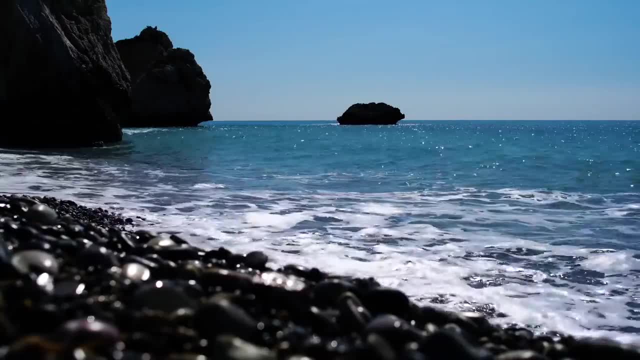 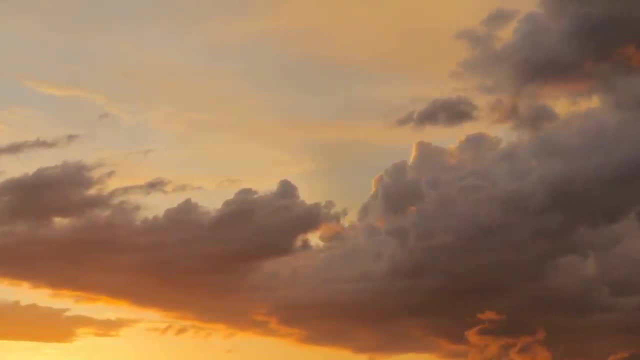 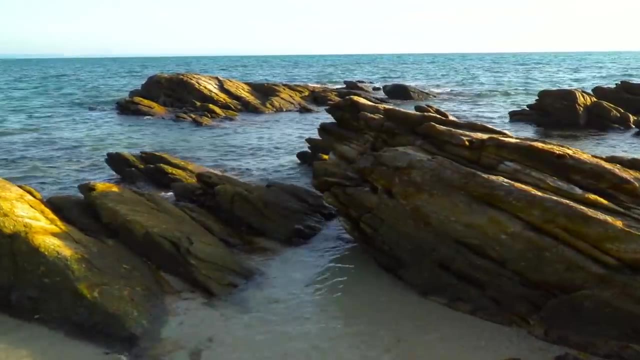 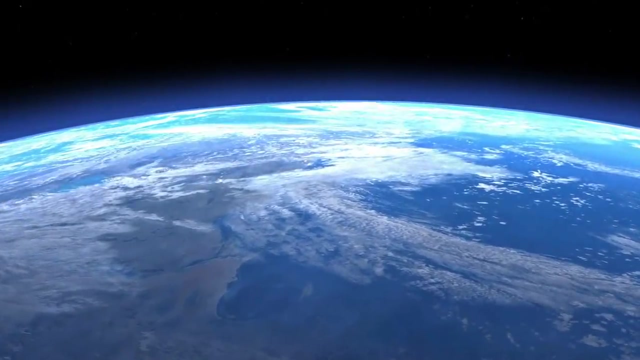 microbes are encased in a mineral tomb from which there is no escape. Deprived of the nutrients they need to survive, the cells die, But they are already beyond the reach of any that might reuse their carbon. As the mineral gel crystallises and hardens, the cells are frozen in their death mask protected. 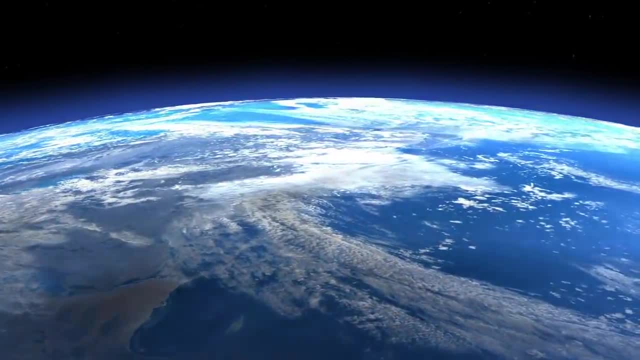 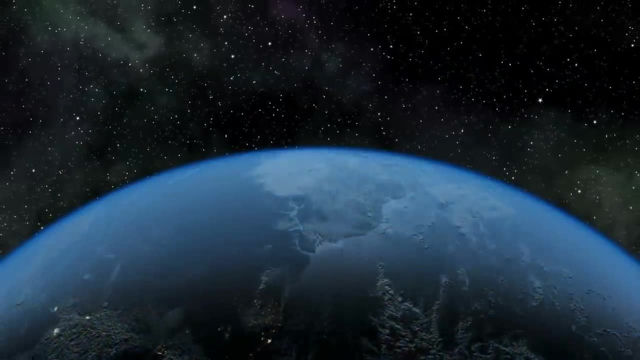 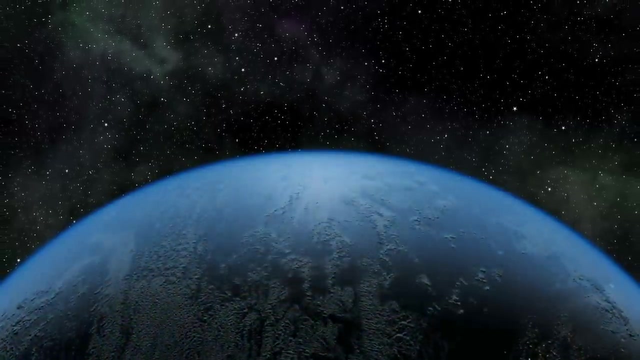 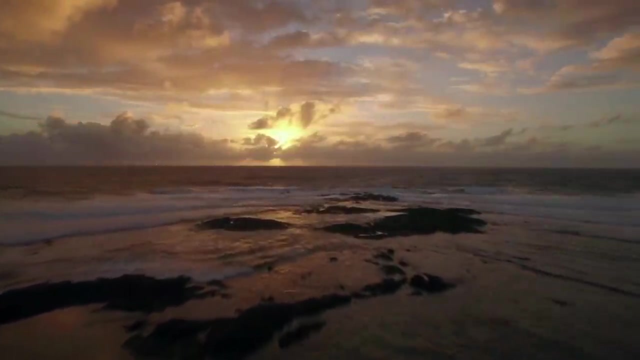 even from the lifeless chemistry that would reduce them to formless blobs. If crystallisation happens fast enough, then the cells are preserved in the three-dimensional positions they inhabited at the moment of their death. If not, and the gel is flattened by sediments deposited on top, then the detail is retained. 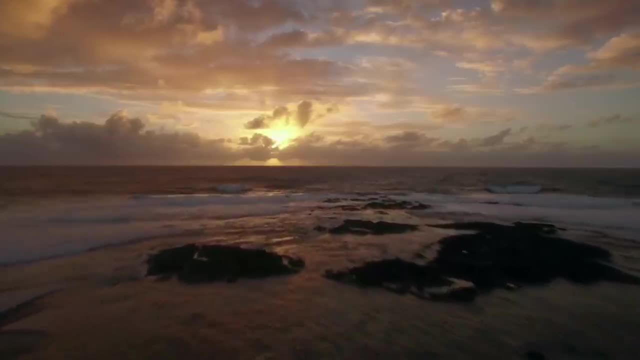 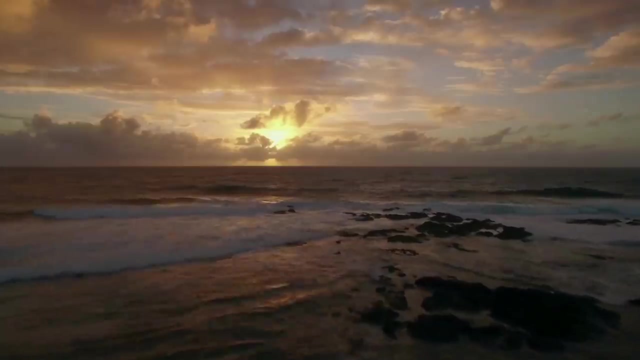 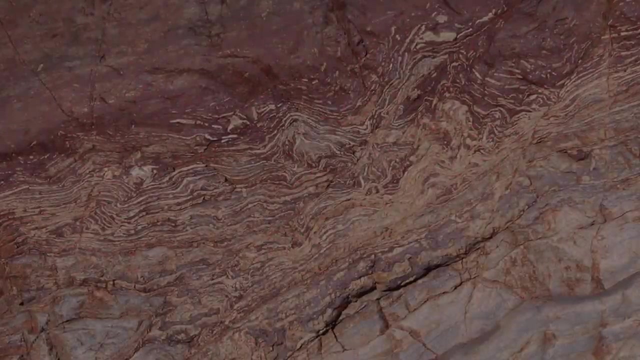 but not their positions. 3D Positions are reduced to two as the delicate fossils are flattened like pressed flowers between layers of mud and sand. This mineral sarcophagus is enough to allow even the most delicate cells to stand the test of time. 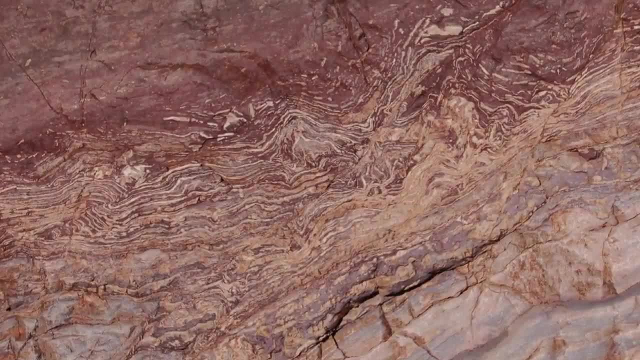 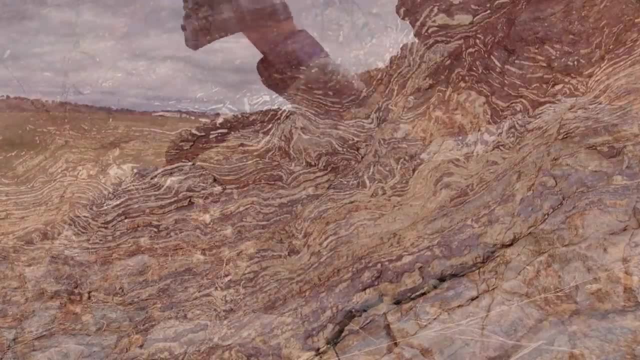 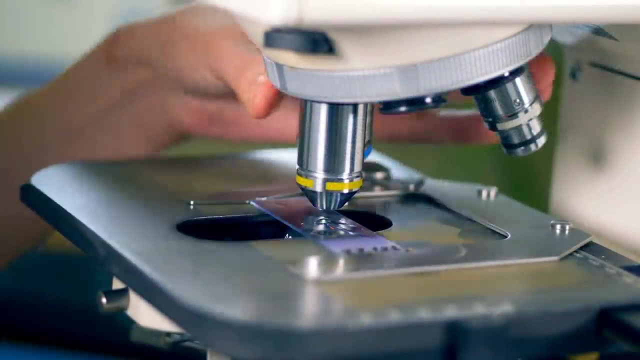 As long as the rocks themselves survive, so does their microfossil treasure. When, hundreds of millions of years later, paleontologists slice those rocks and put them under the microscope…. …or dissolve away the crystalline tombs with acid, they are greeted with delicate 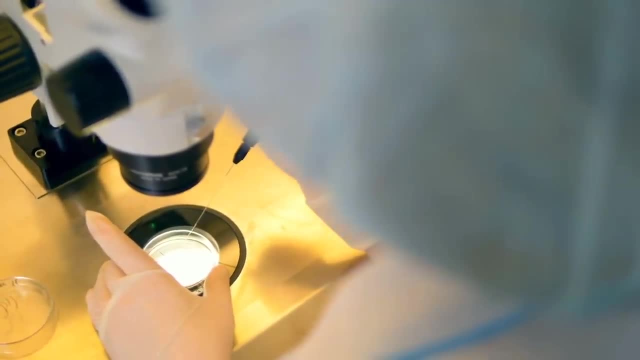 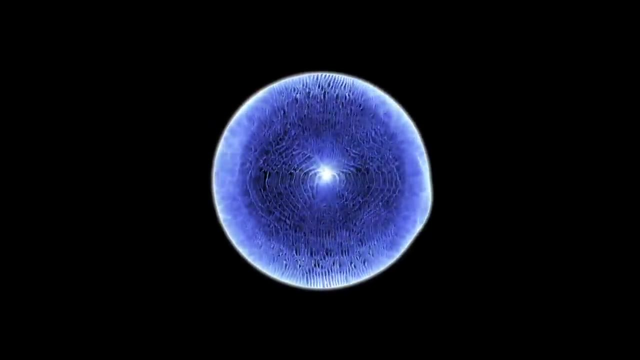 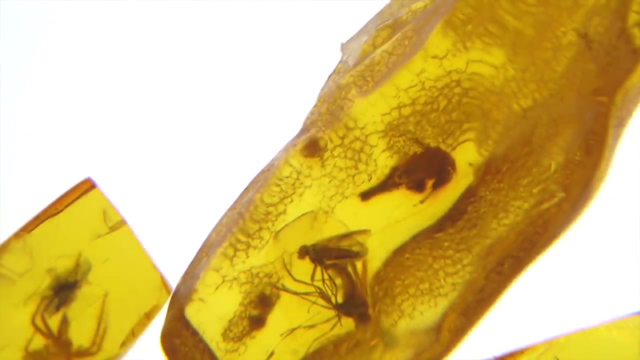 organic walled forms that look remarkably similar to modern cyanobacteria, algae and other single-celled microbes. Just like insects preserved in amber, these appear to be cells that have been frozen in time. Only they are seven times as old And many times stronger. 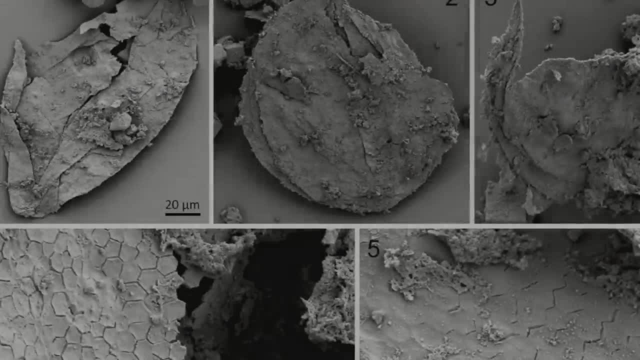 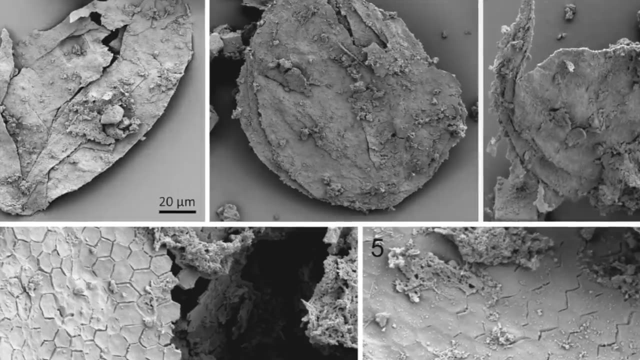 Only they are seven times as old and many times stronger And many times smaller and more flimsy. It seems almost too perfect to be true, And indeed the true nature and antiquity of such exceptionally preserved microfossils has been called into question many times. 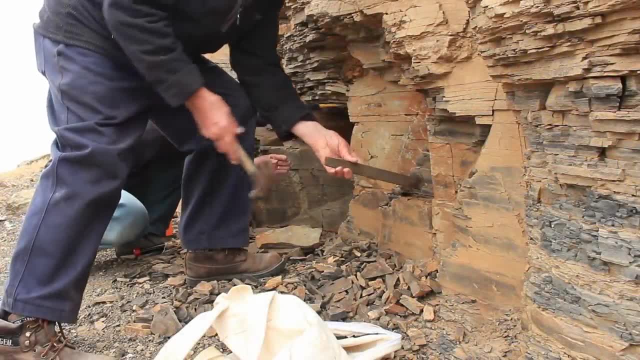 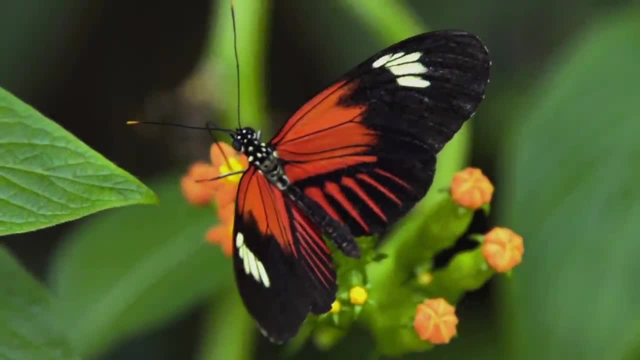 Naturally, the older the rock, the more questionable it is that the microfossil bounty has survived intact, And these are not intricate insects in amber, but forms that are much more simple. Are they really biological cells that have been preserved for centuries? 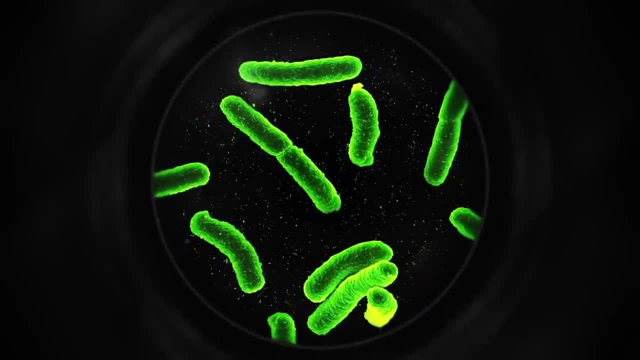 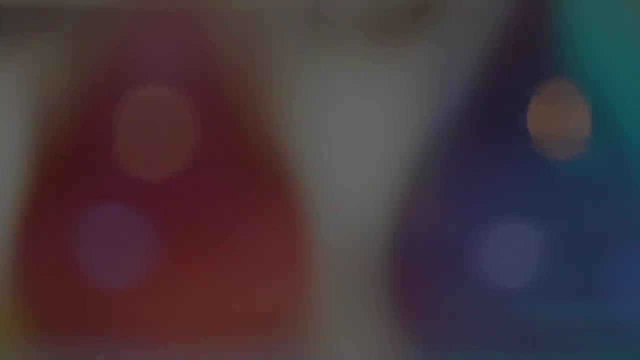 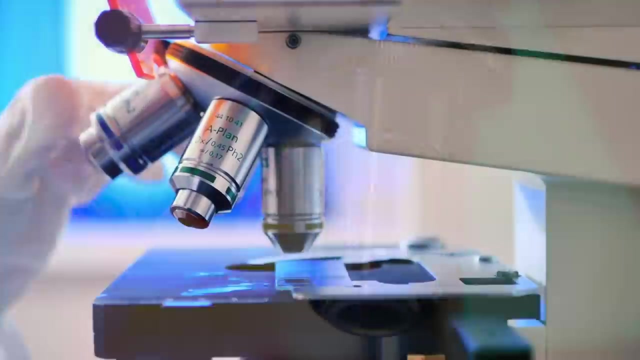 Are they biological cells that are billions of years old Or is it simply wishful thinking? It has been said by pre-Cambrian paleontologists from both camps that extraordinary claims require extraordinary evidence. Impossible fossils that seem to buck the trend of all fossilisation before them must be subjected. 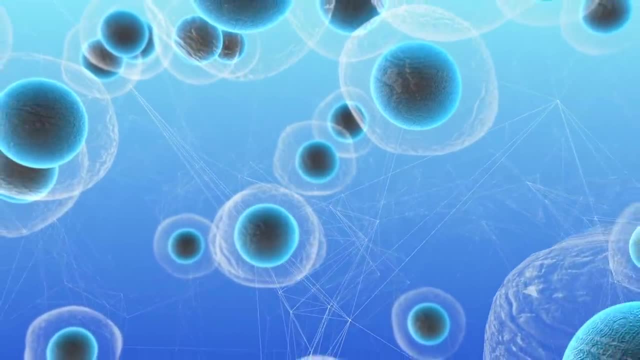 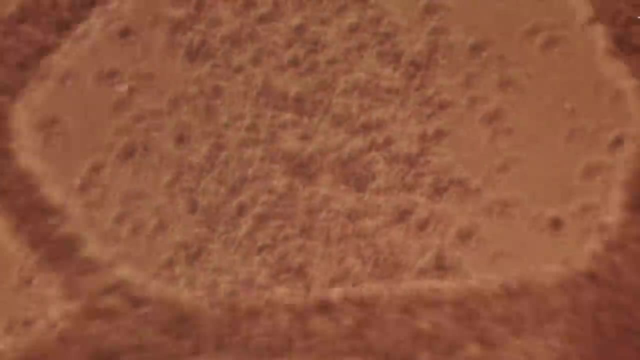 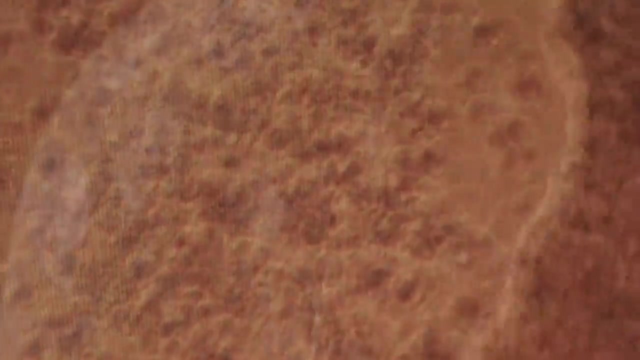 to more rigorous validation than any other. We must prove that they are formed by life. We must prove that they are formed by life And we must prove that they were formed at the same time as the rocks themselves, not introduced later. Luckily, the science of exceptional preservation has matured to the point where such verification 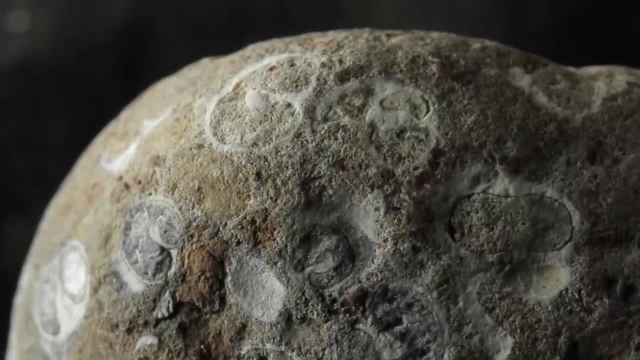 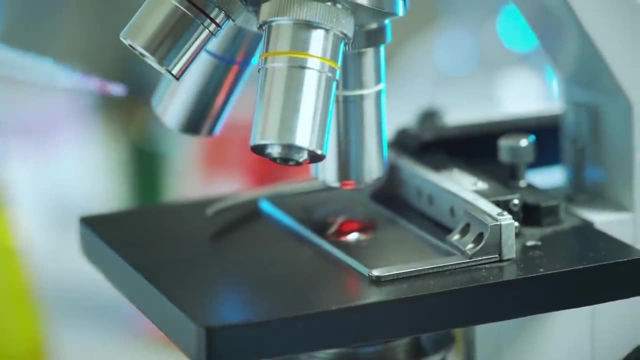 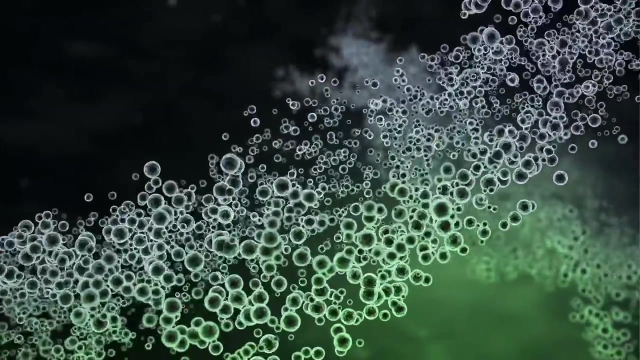 is now routine. Along with documenting the shapes, sizes and associations of microfossils within an ancient rock, experts also look for chemical signals that suggest a biological rather than chemical origin. They look for certain complexity in structure which can't be achieved by physical processes. 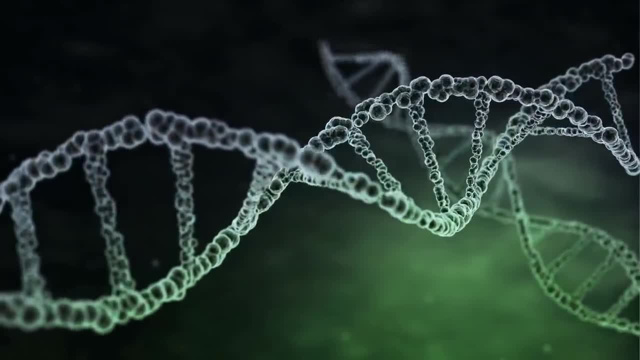 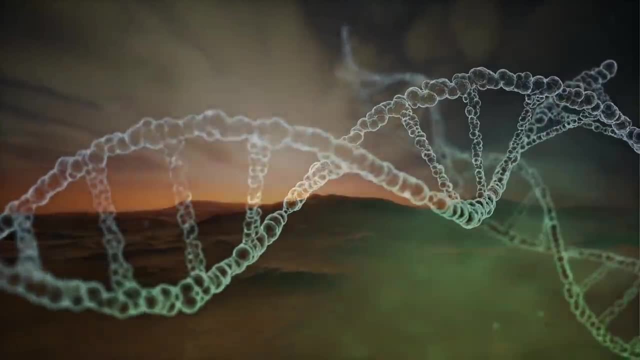 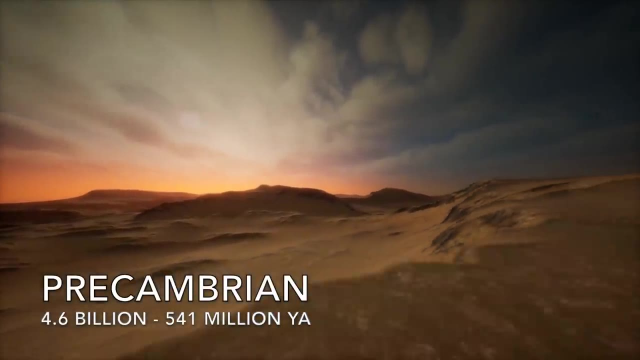 alone, And the surrounding rocks are analysed in minute and microscopic detail to calm any fears that the microbes could have been introduced after the minerals had formed. Now, organic walled microfossils from the pre-Cambrian are no longer impossible, But an important part of our paleontological inventiveness remains. 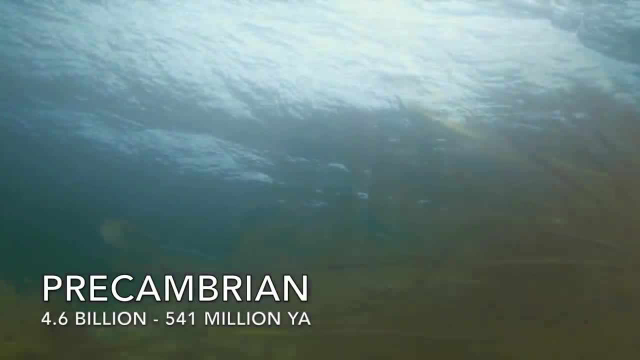 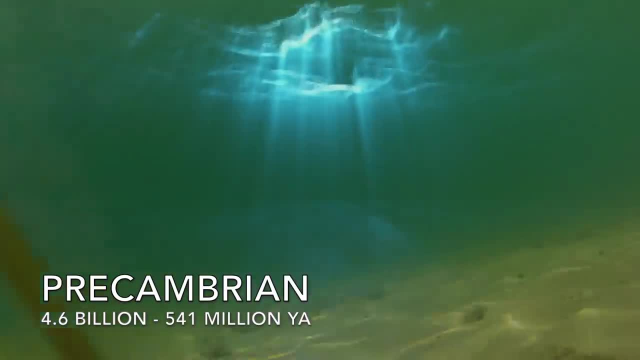 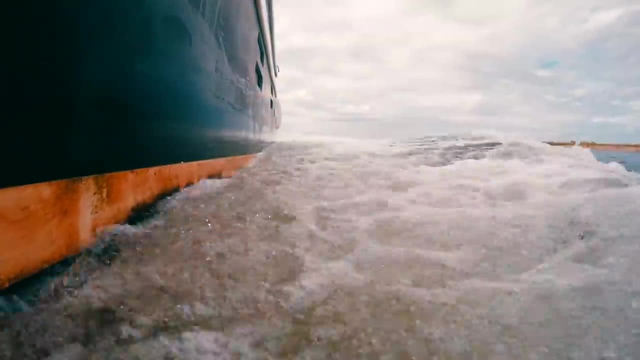 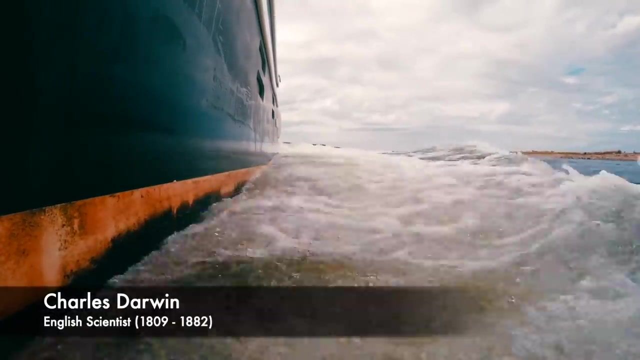 country stretching back at least two and a half billion years. The world is a more complex and interdisciplinary world than Charles Darwin ever hoped to have. but we may not be a full picture, But some two centuries after his birth, it is a better picture than Charles Darwin ever. 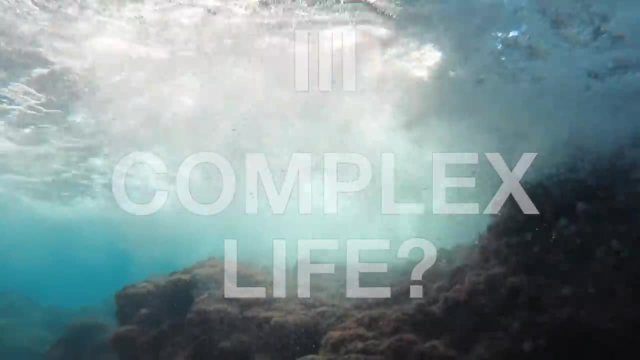 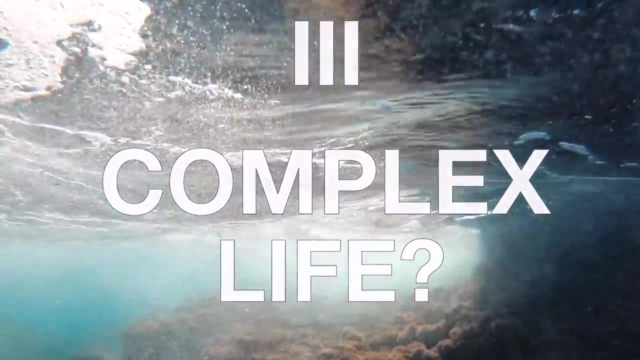 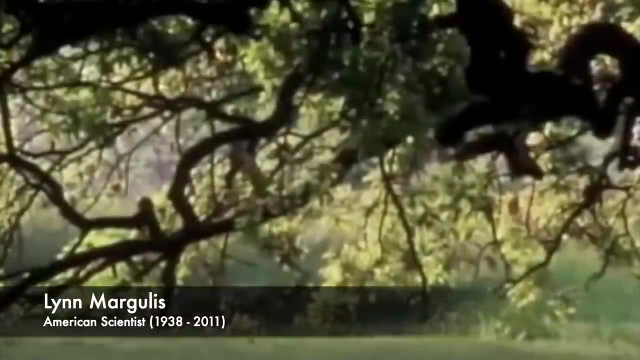 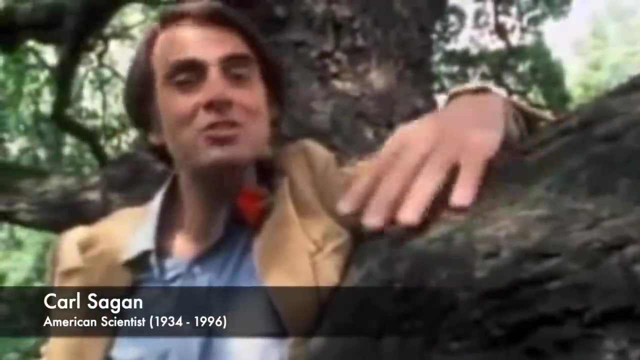 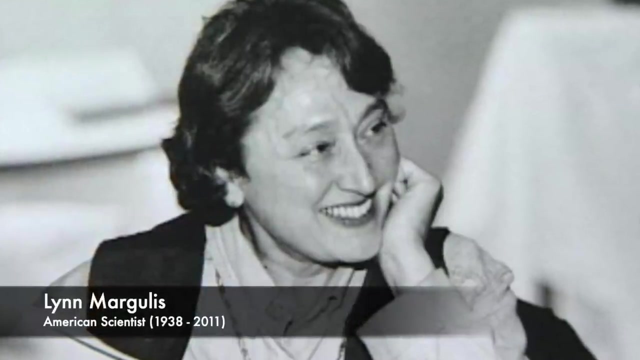 hoped to have, And we now begin the more challenging task of interpreting exactly what it is that picture shows. Lynn Margulis was not your traditional scientist. Once married to the famous cosmologist Carl Sagan, she looked at the world of evolutionary biology in her own unique holistic way. 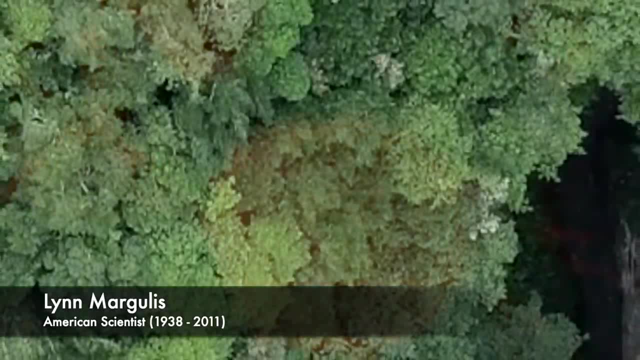 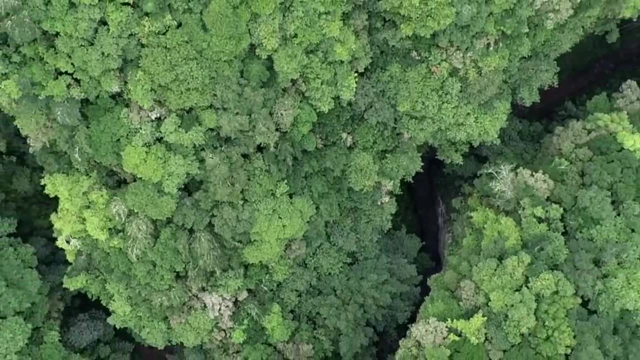 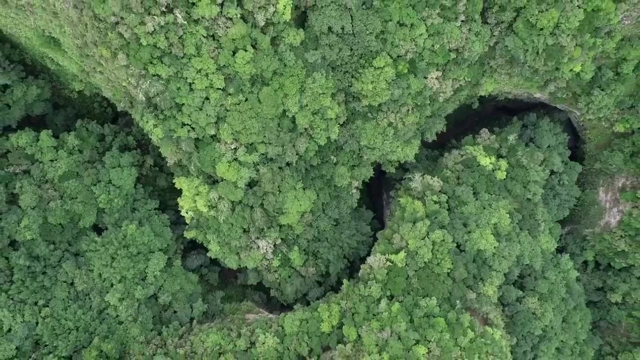 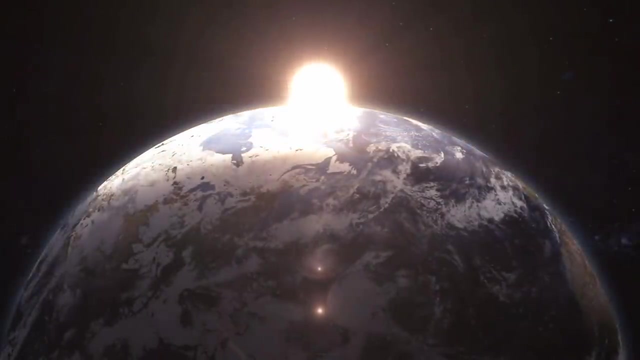 She wasn't interested in how one organism functioned, but pioneered considering the links between even the most disparate creatures. She didn't consider individual habitats as their own isolated environments, but rather looked at the entire Earth system as a vast, interconnected and self-regulating super-organism. 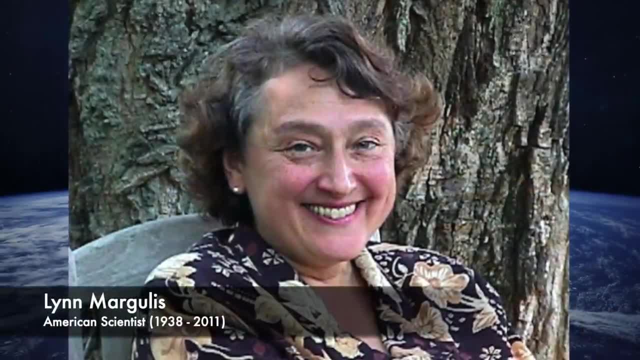 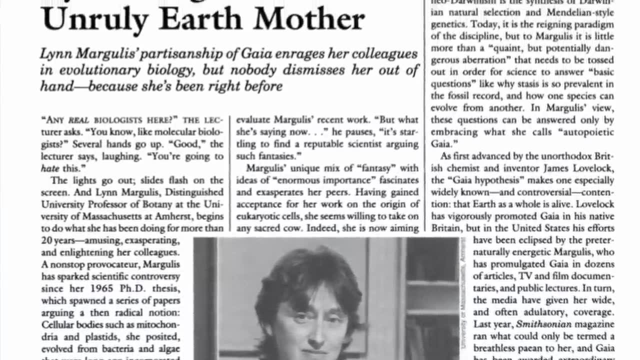 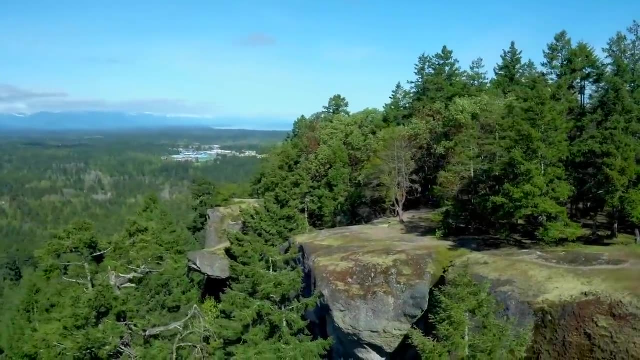 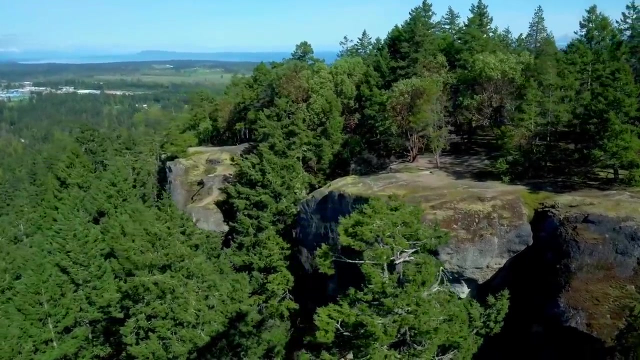 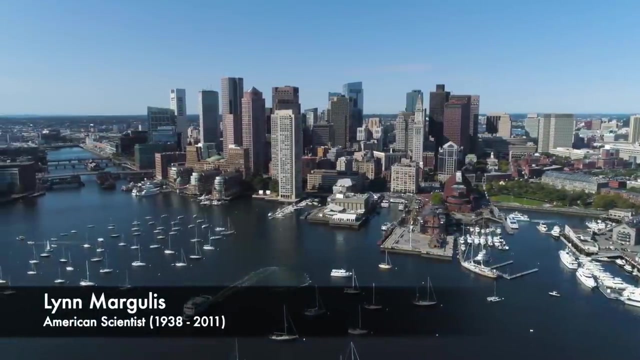 Her theories were wild and unconstrained By popular opinion, earning her the title Science's Unruly Earth Mother. One such theory took shape in her mind in 1966 as she took up her post teaching biology at Boston University. She posited that the more complex eukaryotic cells, from which all higher multicellular 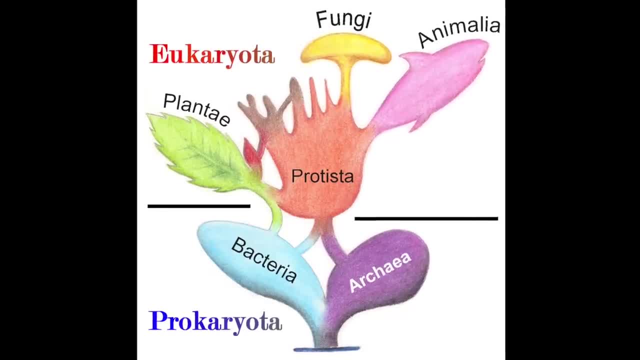 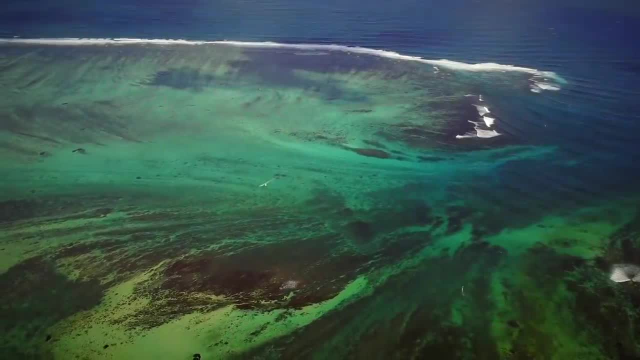 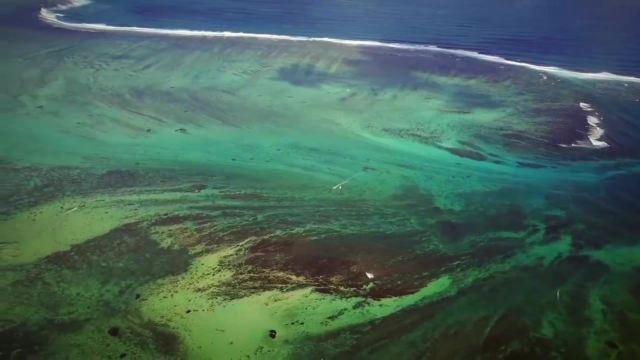 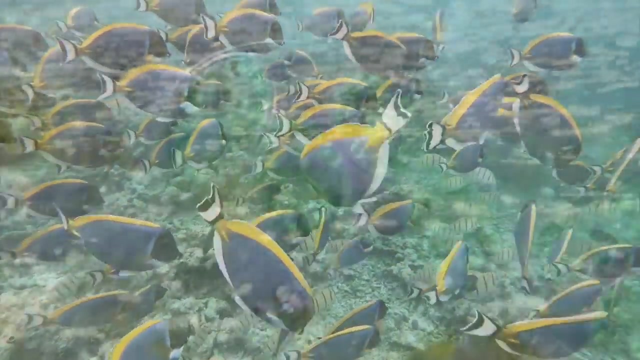 organisms are built came about not from competition but by cooperation. Normally evolution by natural selection brings about changes in living things by favouring certain traits within a species' naturally occurring variation under competitive conditions where resources are scarce. But Margulis suggested that in the case of eukaryotes things happened a little differently. 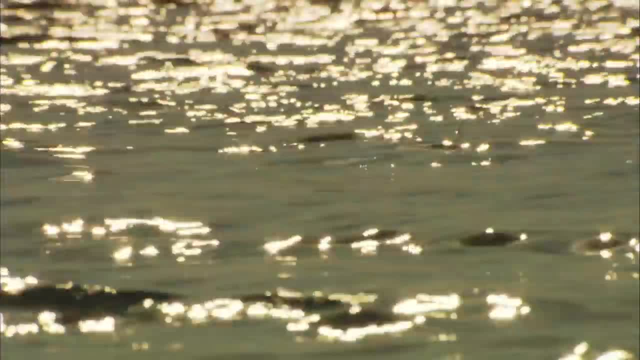 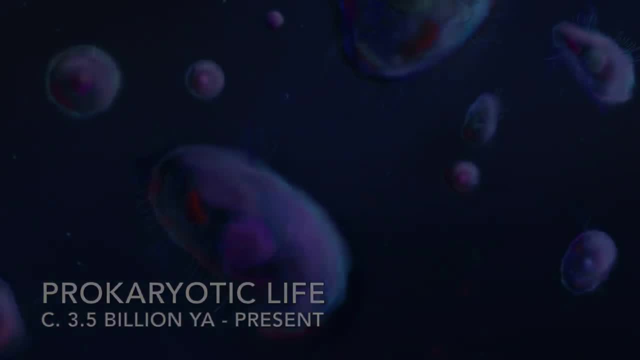 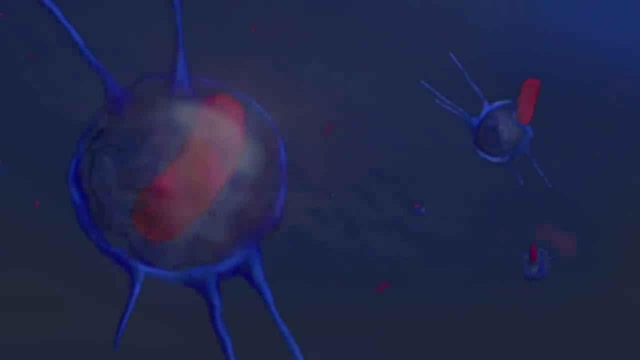 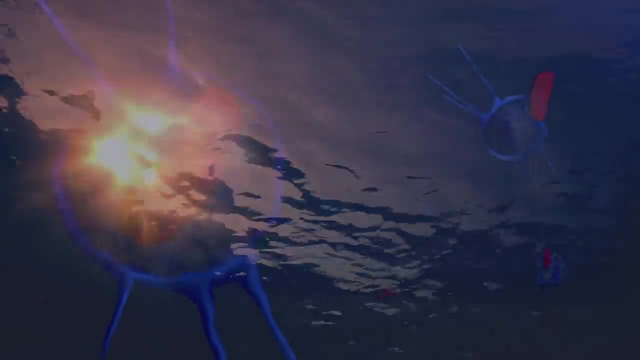 When nutrients ran short in the ancestral prokaryotic world, different bacterial cells contrived to work together to increase both of their survival chances. This pact, or symbiosis, was secured by a physical association. One type of prokaryote would physically come to live inside another and reproduce alongside. 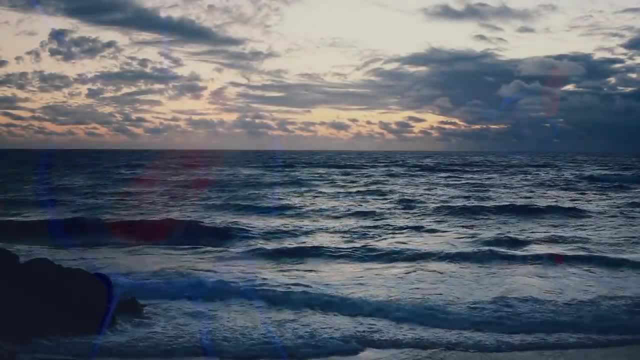 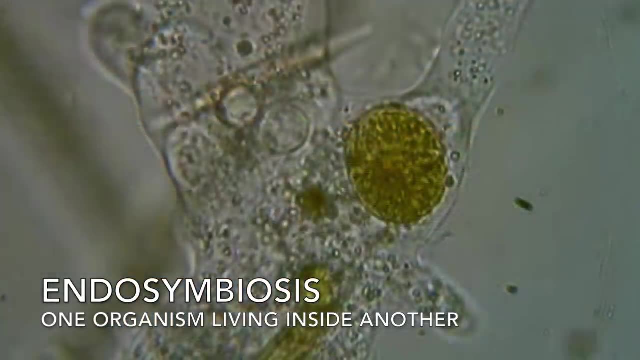 it, And thus Margulis's theory came to fruition. In the late 19th century, the eukaryotes were considered to be the most important species. Margulis's theory of endosymbiosis took shape. It seems like a strange assertion, and indeed it was too strange, too unsupported by actual 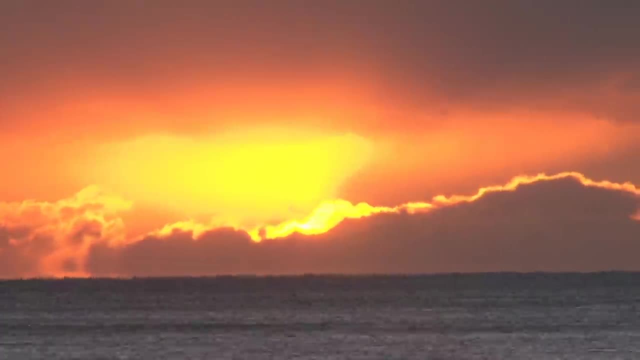 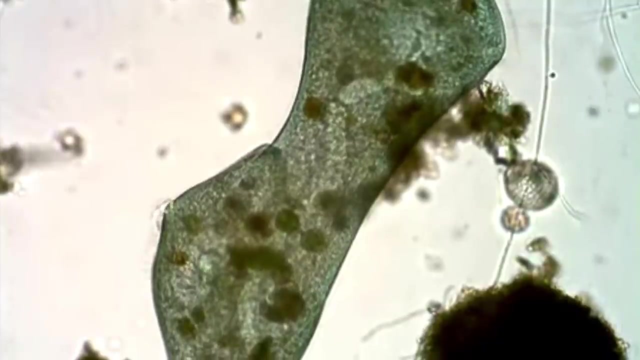 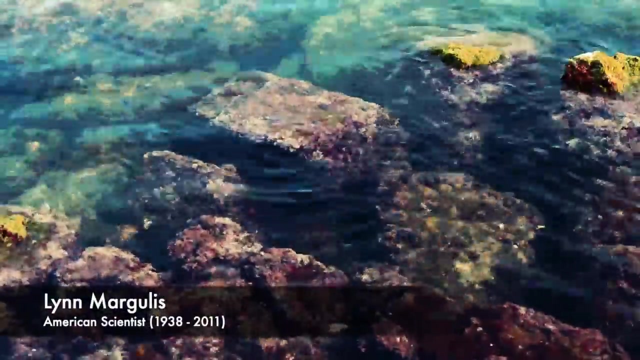 evidence for many to accept it straight away. Margulis submitted her paper to about fifteen scientific journals before one, the Journal of Theoretical Biology, finally agreed to publish it. She spoke about the theory everywhere she went: At scientific seminars, conferences, workshops and even among friends. 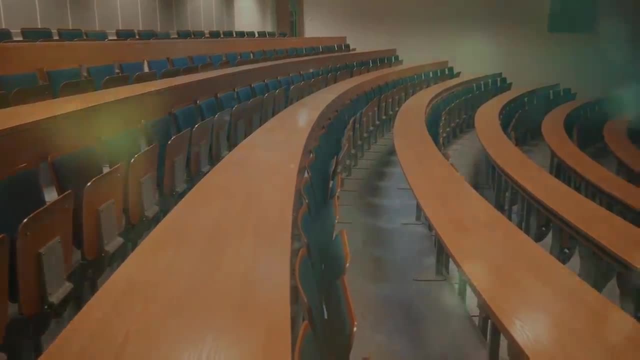 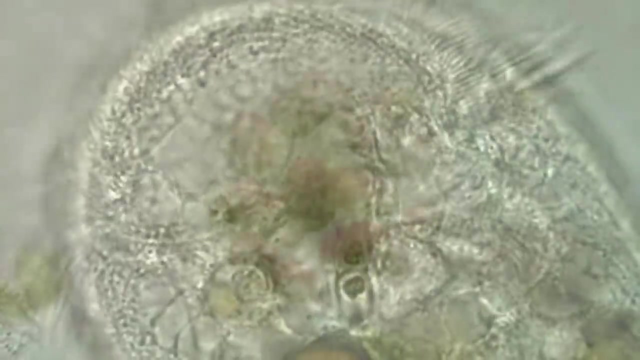 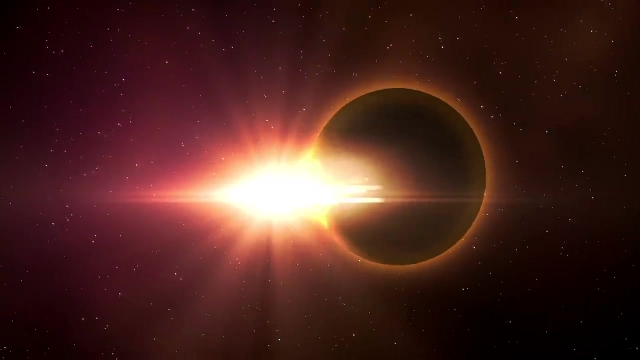 But for a long time the idea of bacterial cooperation was just too much for many to countenance. For about fifteen years Lynn's ideas were considered fringe science and perhaps never taken completely seriously. But by the 1980s a new analytical technique gave the endosymbiosis a new meaning. 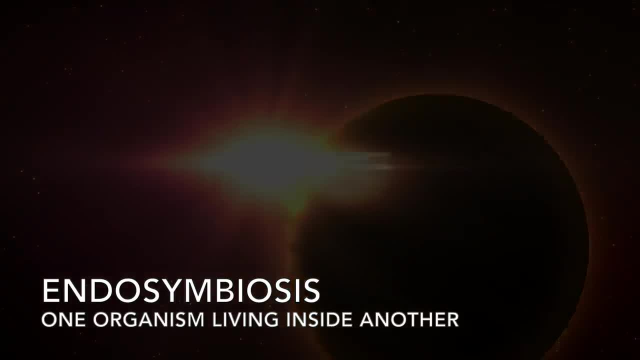 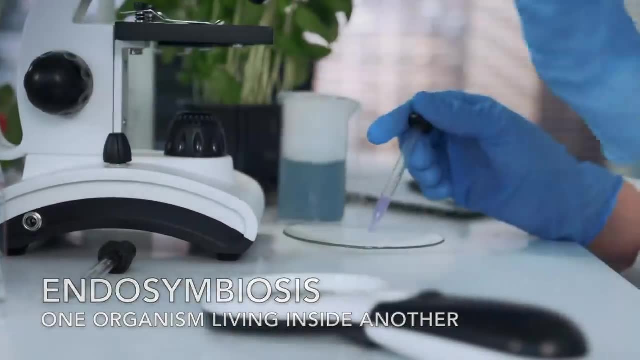 The endosymbiosis was the first scientific theory to have been developed in the early 19th century. The endosymbiotic theory, the spark of credibility it needed. It was discovered that mitochondria, the famed powerhouses of the eukaryotic cell, have their 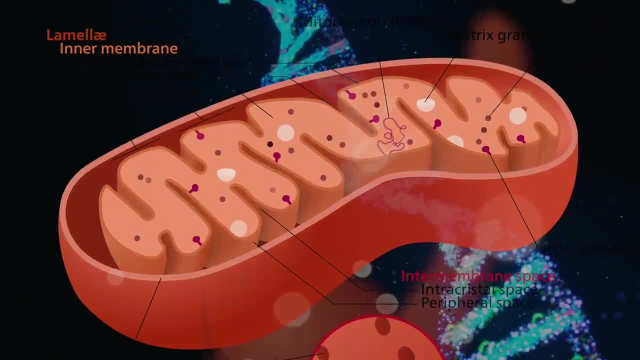 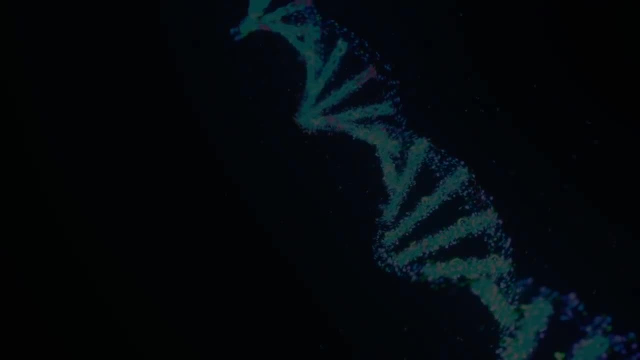 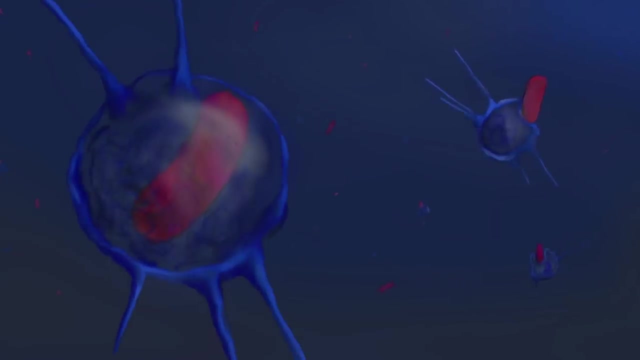 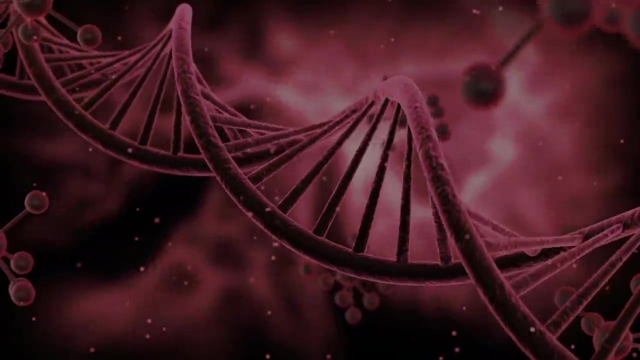 own unique DNA that is unrelated to the DNA of the host. Later, the same was shown to be true for chloroplasts. Margulis had claimed that these structures were once independent organisms, But they were not, And now their genetic signatures were indicating that was true. 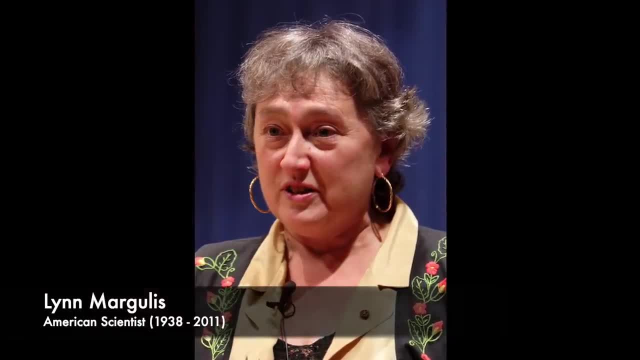 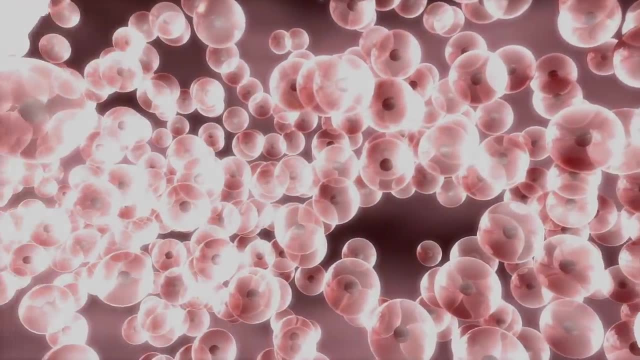 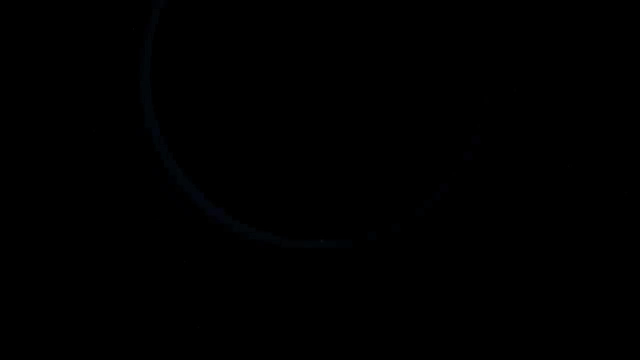 It looked like she had been right all along, Having ridden the endosymbiotic storm from rejection through suspicion and eventually to orthodoxy. Lynn Margulis's unruly approach to science only deepened, and she developed a taste for the controversial. 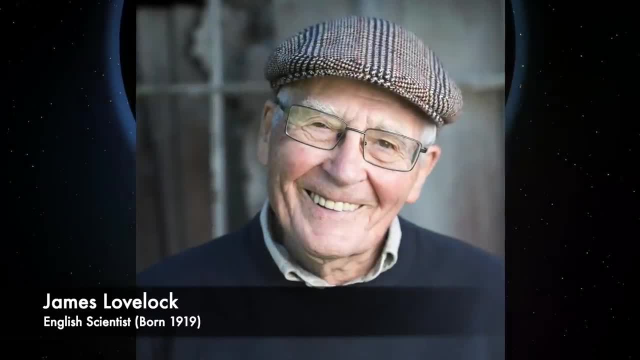 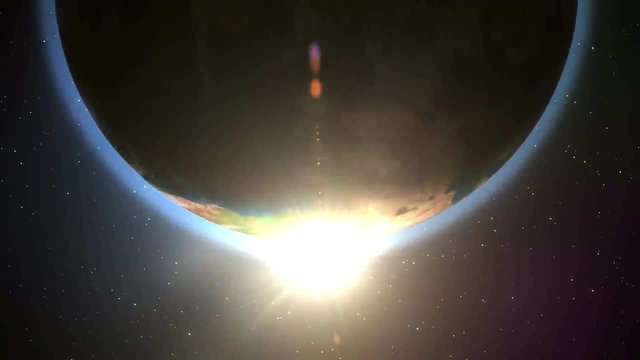 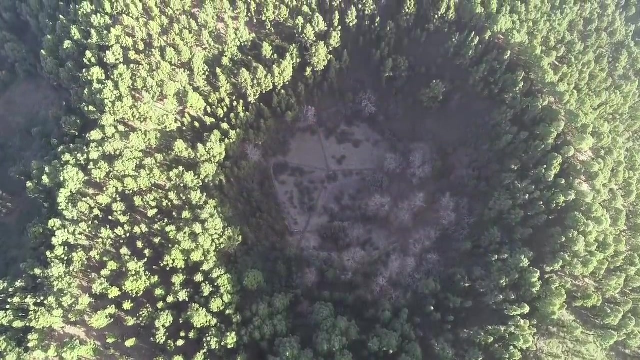 She worked with James Lovelock to give substance to his Gaia theory that the endosymbiosis is a single self-regulating super-organism and fought hard to make her case for five kingdoms of life: animals, plants, fungi, single-celled eukaryotic protists and prokaryotic. 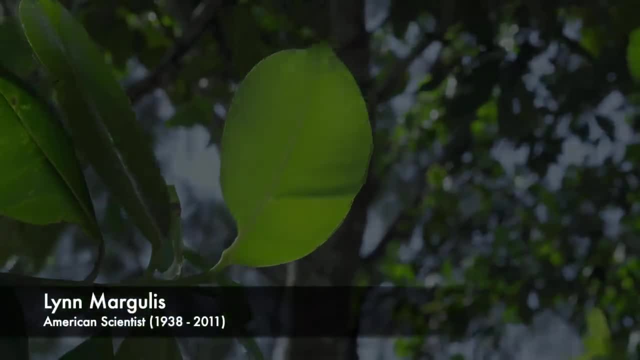 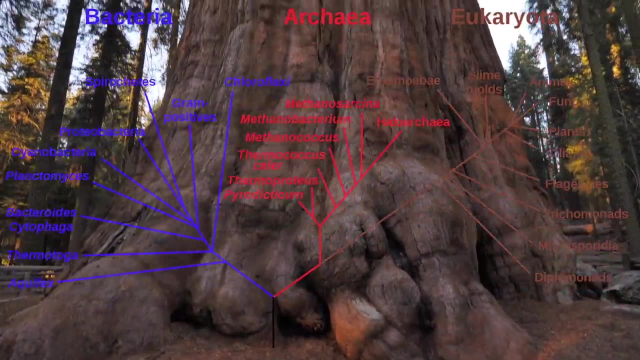 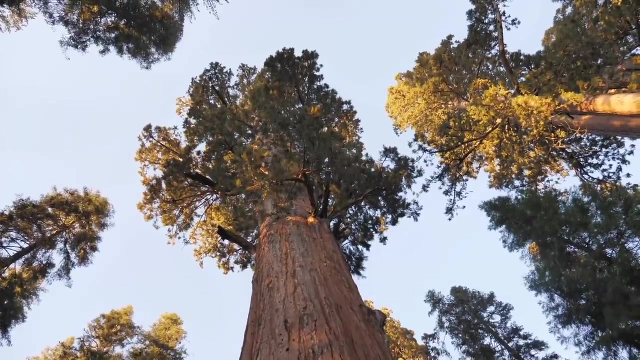 monera. She even went so far as to reject the three domains of life that emerge from genetic analysis of prokaryotes, despite the fact that it was this very genetic analysis that had given substance to endosymbiosis. Nevertheless, as unorthodox as her opinions and approach may have been, there can be no. 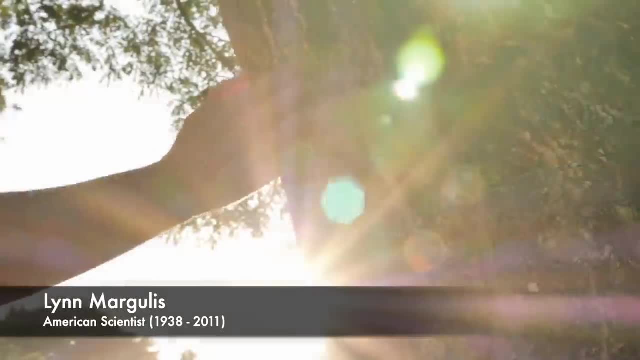 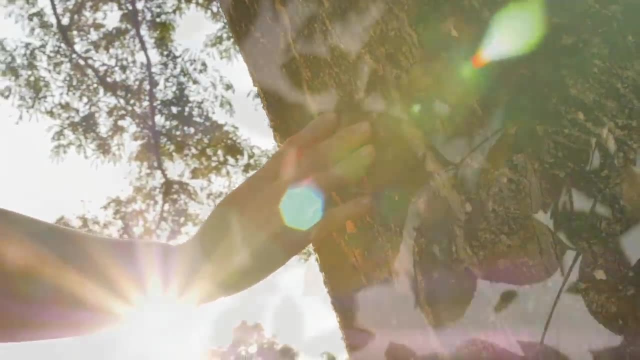 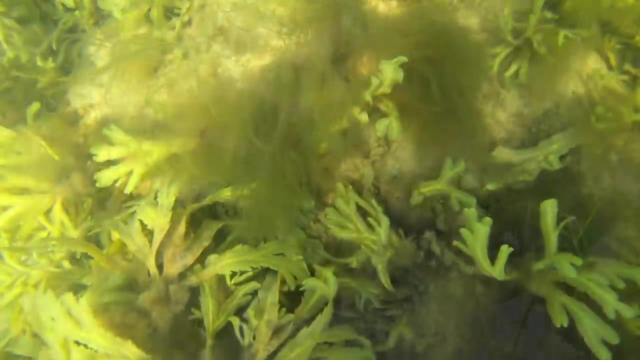 denying Lynn Margulis's uncompromising passion for microscopic life, And she was one of its most vocal advocates right up until her death in 2011.. And, of course, There is No doubt. But anything can happen, and unknowingly, 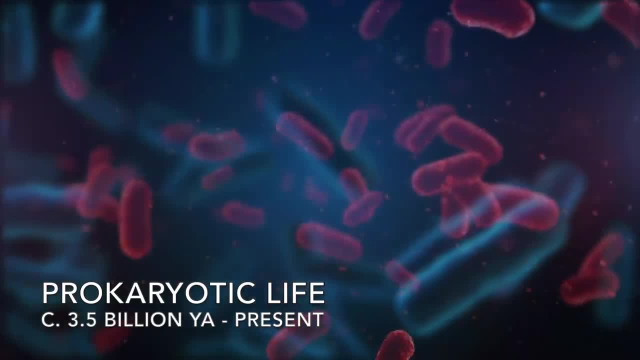 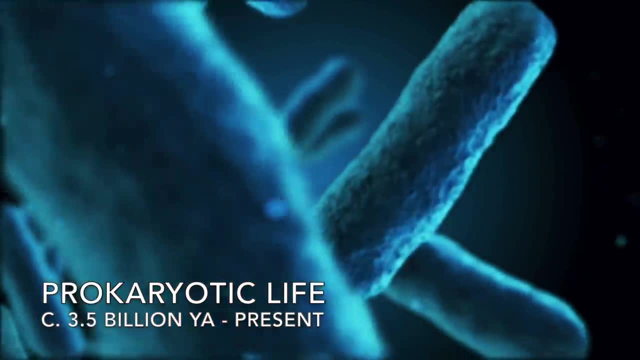 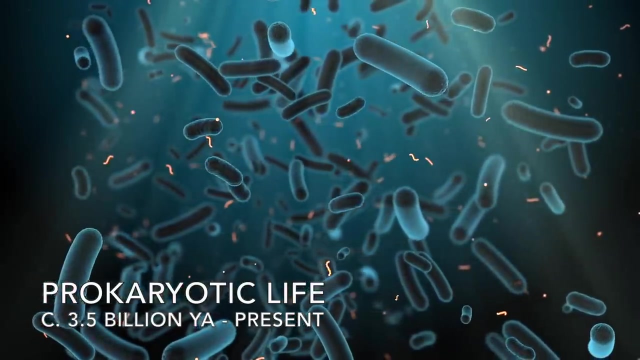 Prokaryotes are most commonly depicted as simple pill-shaped rods, but they can also be spheres, filaments, loose spirals, as well as various bunched and tangled associations of all these. In size, they typically range from less than a tenth of a micron to five microns in length. 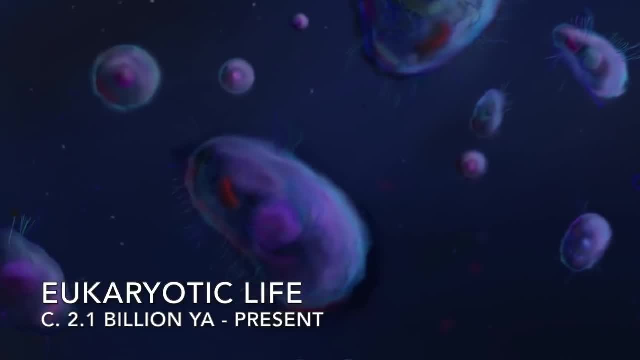 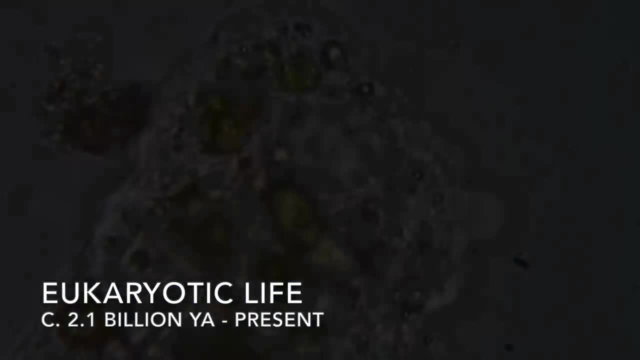 Modern eukaryotes, by contrast, are larger and more complex. Inside their cells, they contain the organelles obtained by an extracorporeal mechanism which is called the pituitary gland, obtained by endosymbiosis, including the mitochondria, chloroplasts and tail-like flagella. 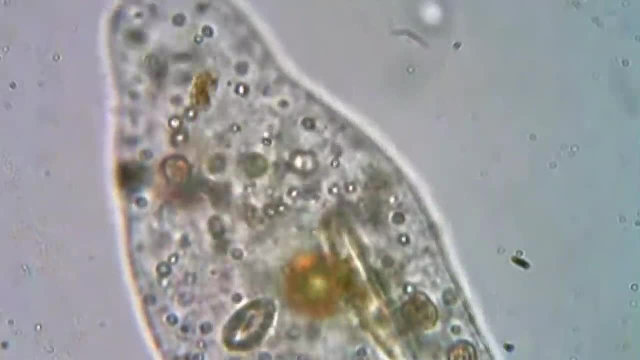 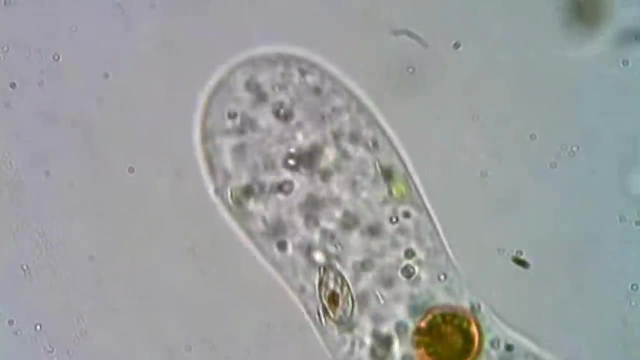 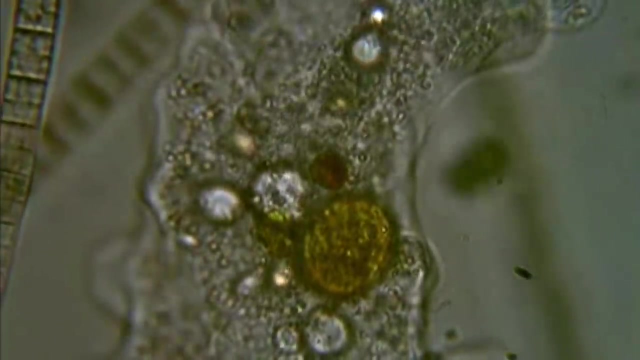 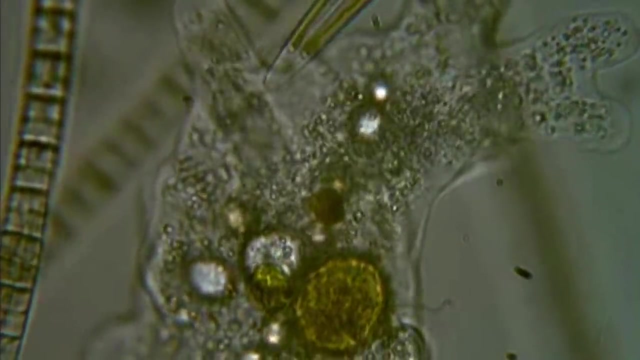 But they are also packed to bursting with other cellular machinery and internal membranes thought to have evolved by more traditional natural selective means. Genetic material doesn't float freely throughout the cell, but is instead contained in a membrane-bound nucleus And there is an ephemeral but highly organised structure to the gel-like cytoplasm which 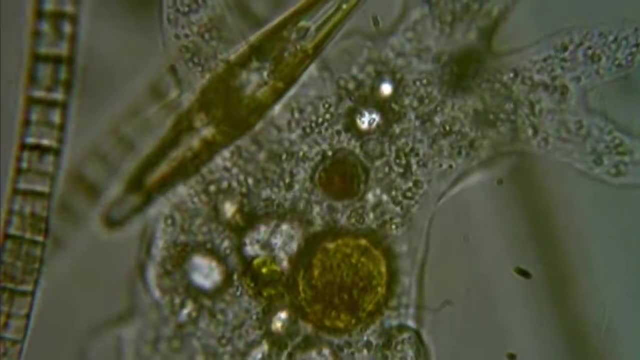 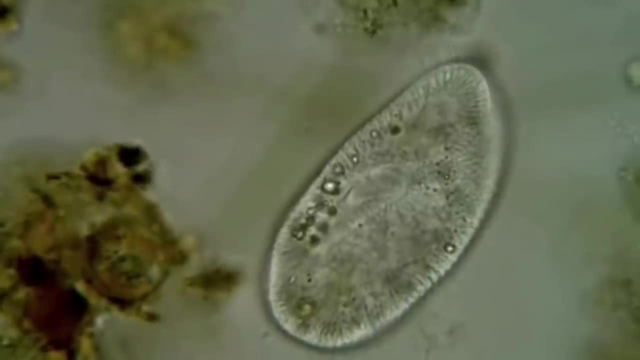 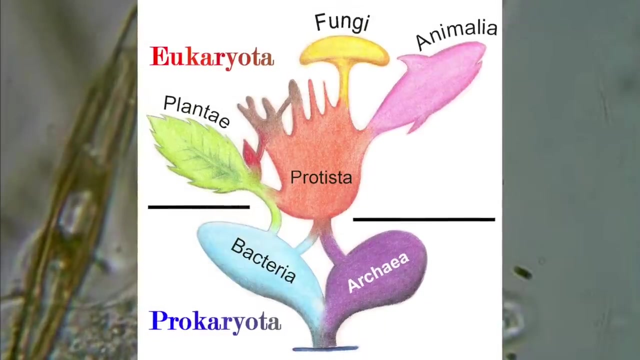 helps coordinate the complex processes of cell splitting and sexual reproduction. It is called a cytoskeleton. It is this internal organisation that allows eukaryotes to become the basis of all higher forms of life, the macroscopic multicellular organisms that evolved much later. 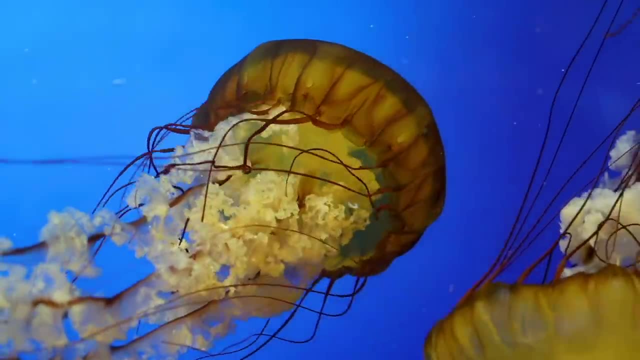 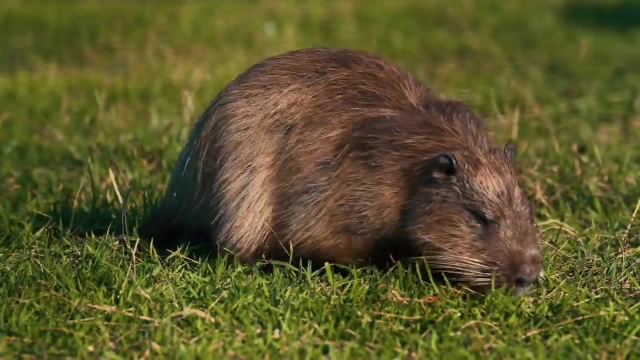 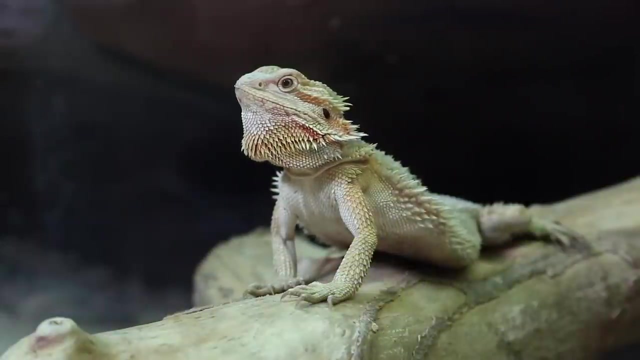 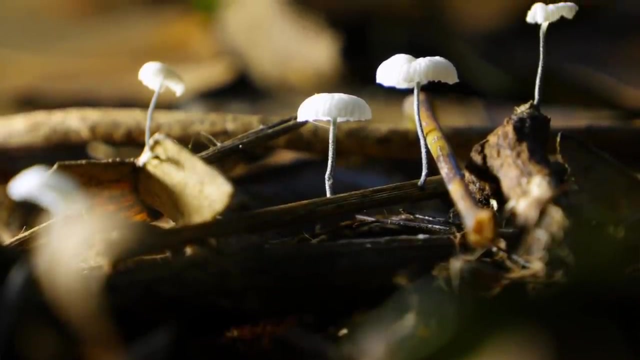 If we are to search for eukaryotes in the Precambrian fossil record, we must take a lesson from Lynn Margulis and think laterally. If the internal features of this more complex life aren't preserved, then instead we must search for features from which we can infer a more complex organisation. 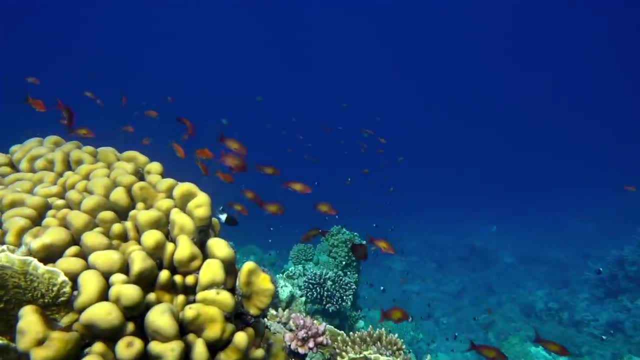 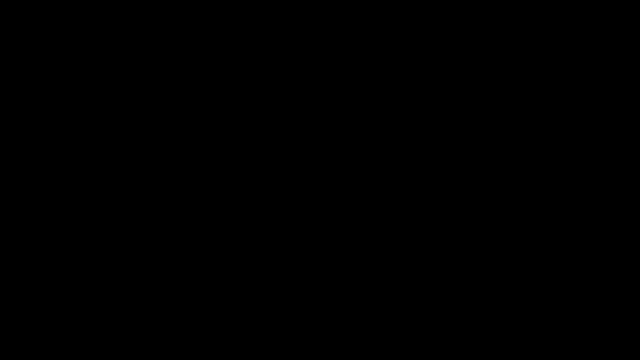 These are things that something only a cell with organelles like a cytoskeleton can accomplish. One such feature is the microfossil's size. In general, prokaryotes tend to be smaller than 5 microns in diameter, and eukaryotes 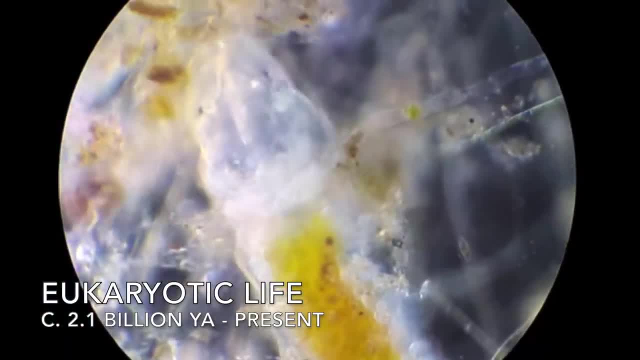 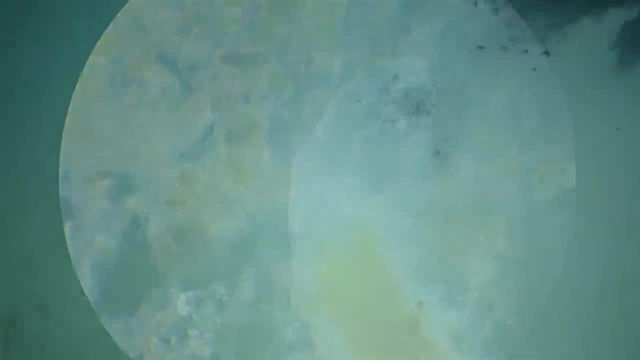 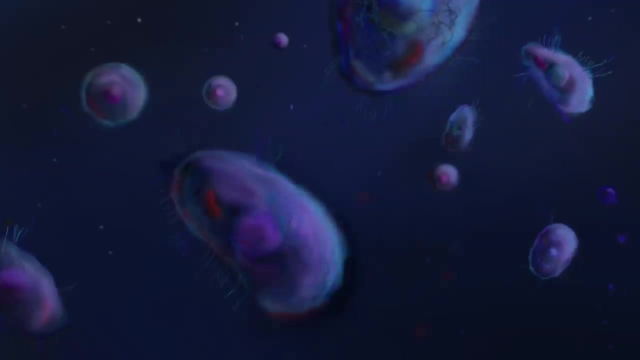 are at least 10 microns across, But even today we see exotic super-sized bacteria or miniature eukaryotes. Encapsulated colonies of bacteria can easily reach a larger size, And once self-digestion occurs, there is no way to tell who the outer case belongs to. 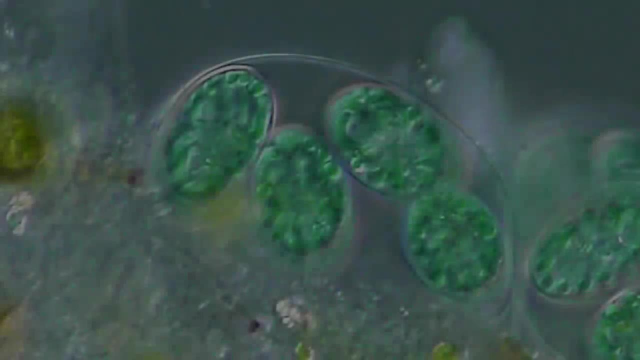 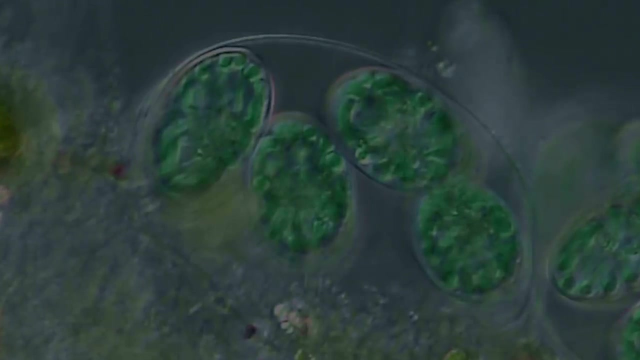 So size is a good first indication but is by no means reliable. A much more reliable indication can be found in the organic walls of the microfossils themselves. A simple cell wall is easy enough to build, but any patterns or embellishments require. 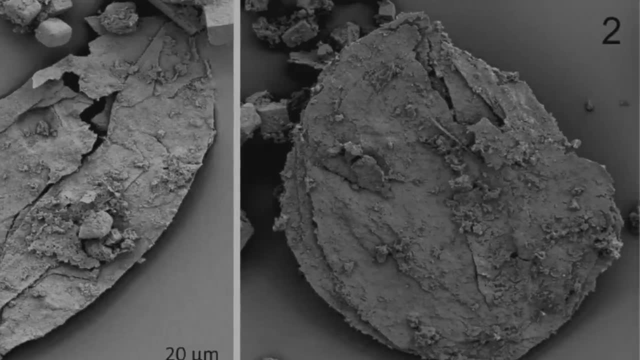 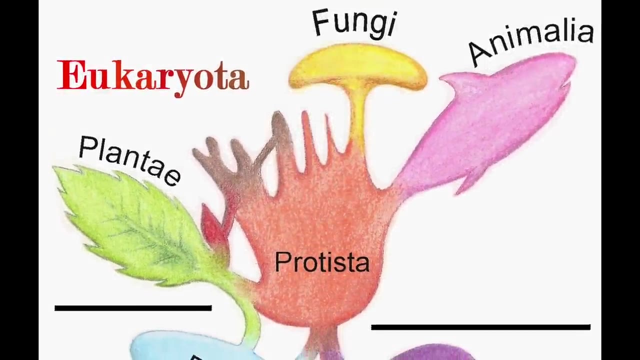 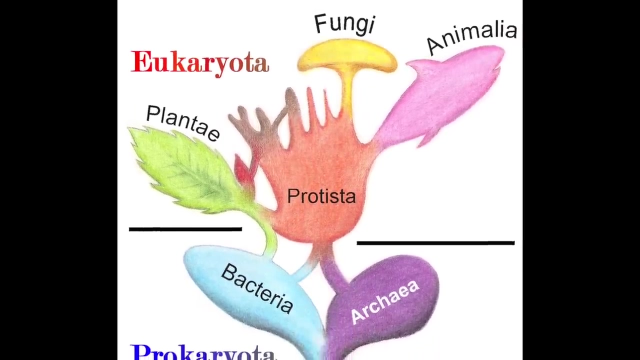 more cellular organisation than a prokaryote can muster. So paleontologists agree that any organic microfossil that is adorned with spines or other external structures and ornamentation must in fact be derived from a more complex eukaryote. 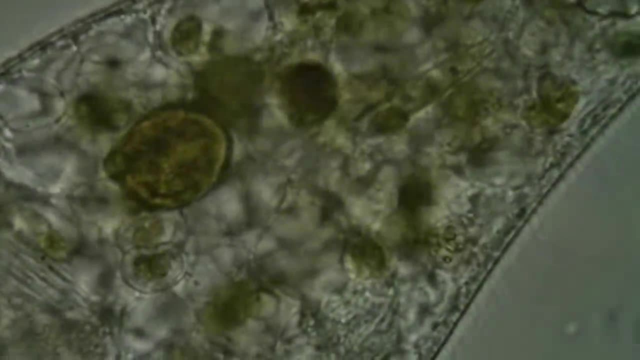 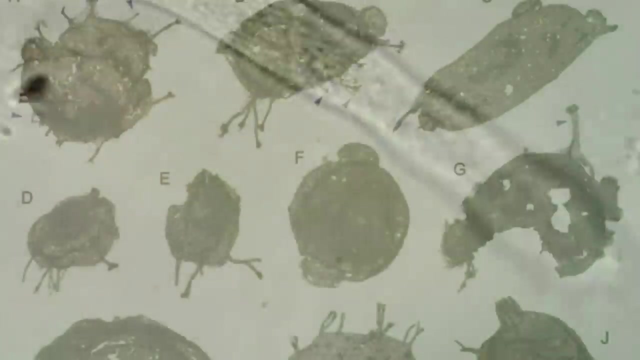 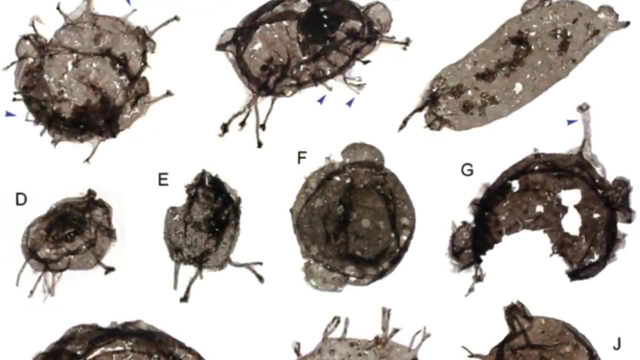 More simple. outer walls and sheaths are more difficult to pin down, but again, some clues can point towards a level of organisation only possible with complex internal machinery. Many modern single-celled eukaryotes are able to survive through periods of environmental stress by encasing themselves in more resistant cysts from which they emerge when conditions. 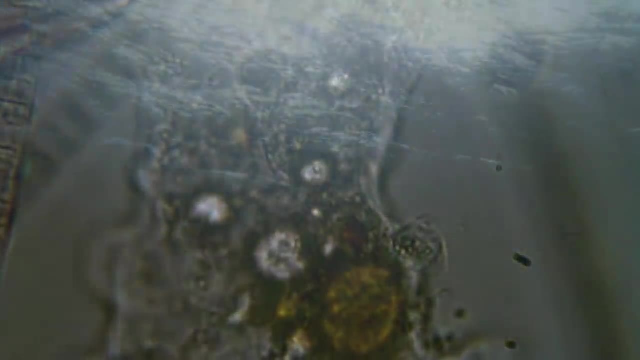 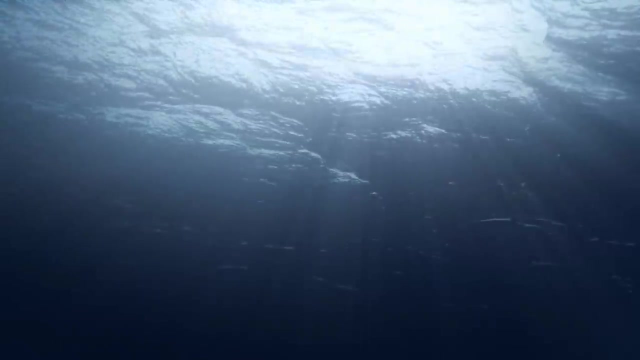 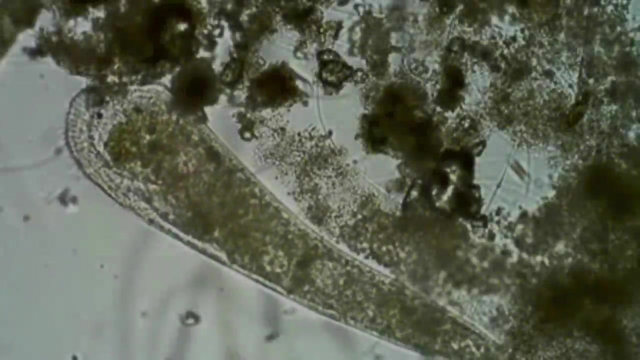 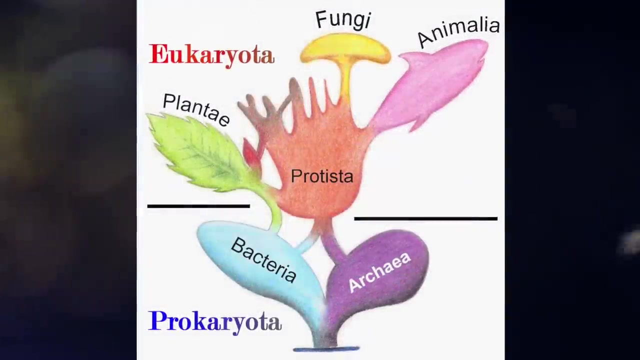 are improved, And nothing is more environmentally stressful than suddenly being encased in mineral gel. So we can expect to find these cysts among the microfossil assemblages. The simple, structureless innards of the average prokaryotic cell could never build a tree. 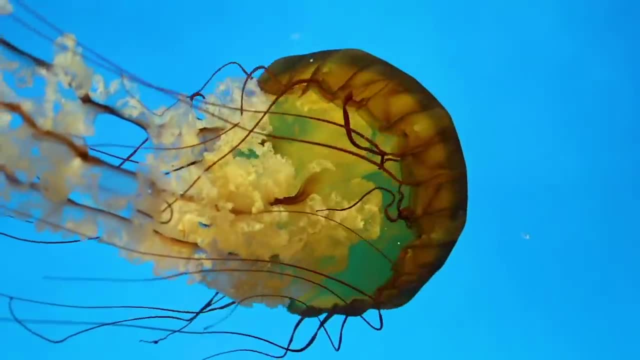 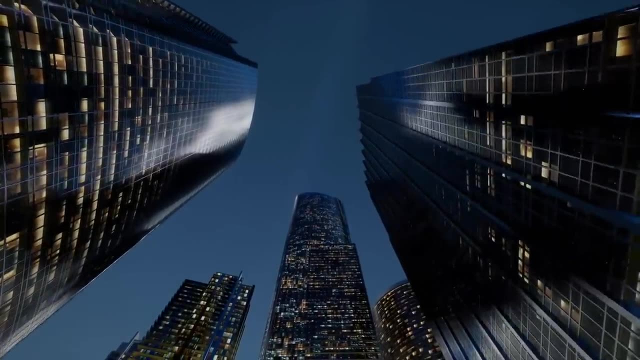 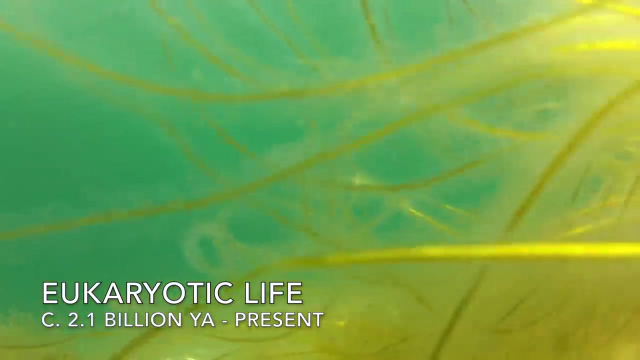 Or a jellyfish, Or a human. It takes the complexity of a eukaryotic cell to make the visible life on Earth as we know it. Of course, such complex machinery takes time to evolve, even with endosymbiosis providing a leap off the starting line. 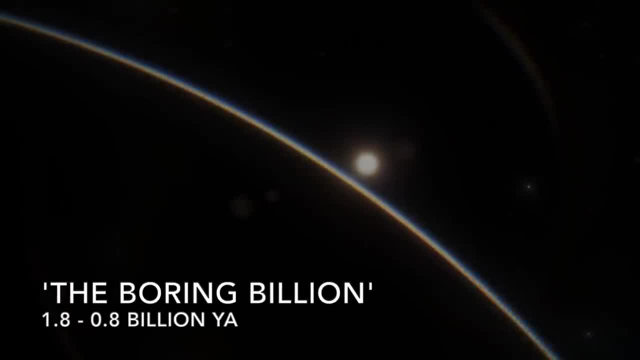 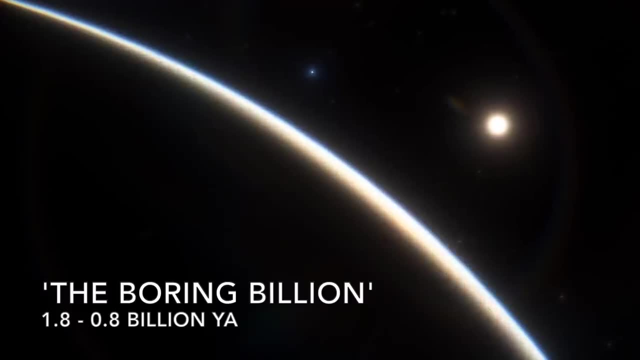 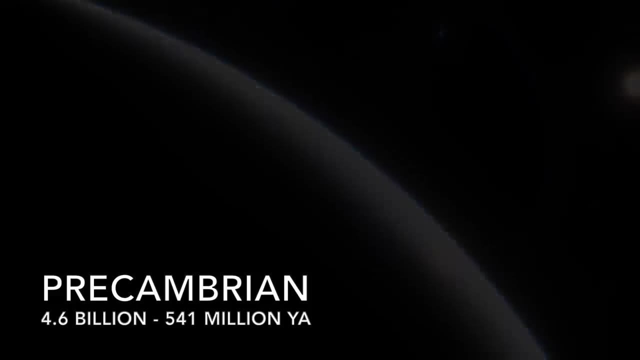 And it's thought that the Boring Billion, the period of unprecedented geological stability between 1.8 and 0.8 billion years ago, provided the perfect conditions to gestate these changes. Now that exceptional preservation throughout the Precambrian is offering us a window on the microscopic life that thrived at this time, 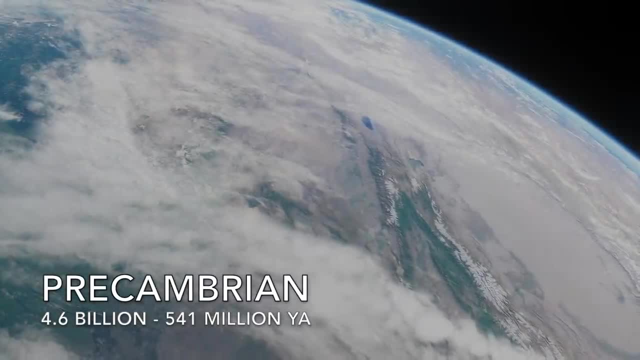 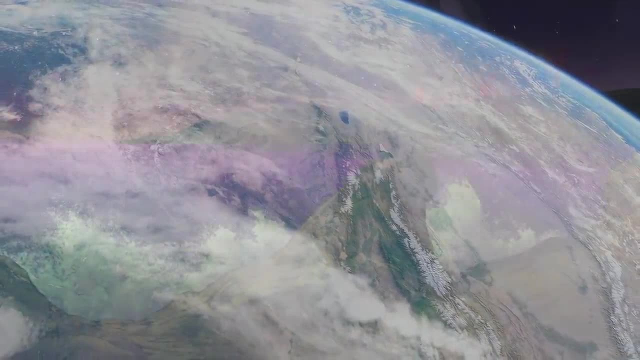 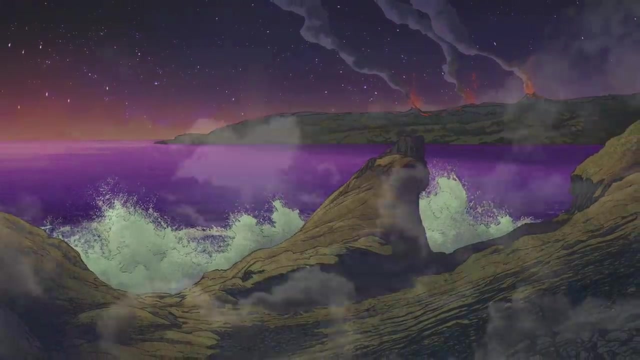 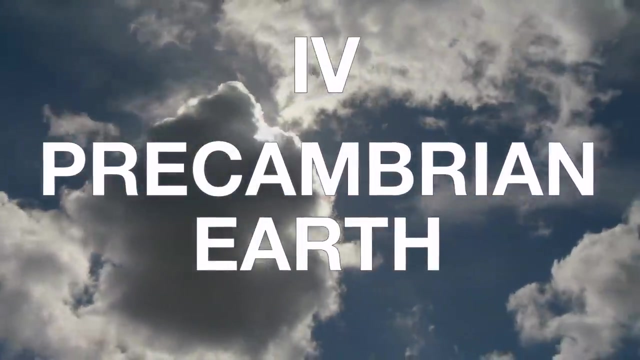 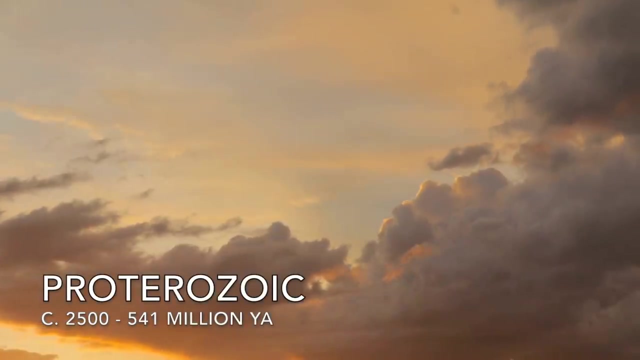 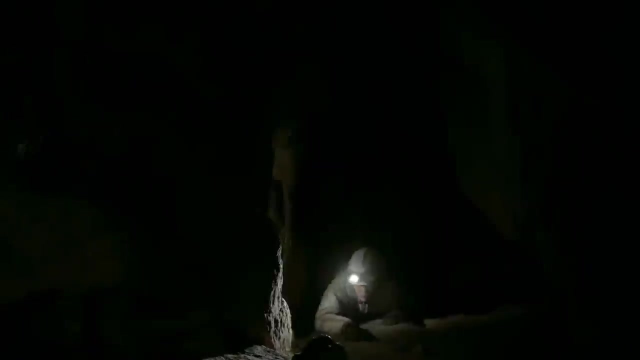 can we find evidence of these monumental evolutionary changes in the fossils themselves And even possibly answer the question: what and when was the first complex eukaryotic life? A protozoic fossil hunter is, unlike any other kind of paleontologist, Walking among ancient rocks. 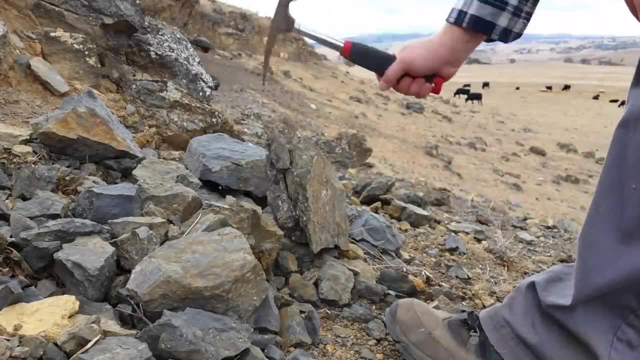 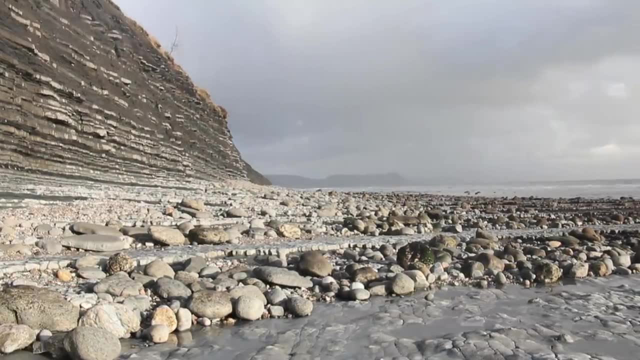 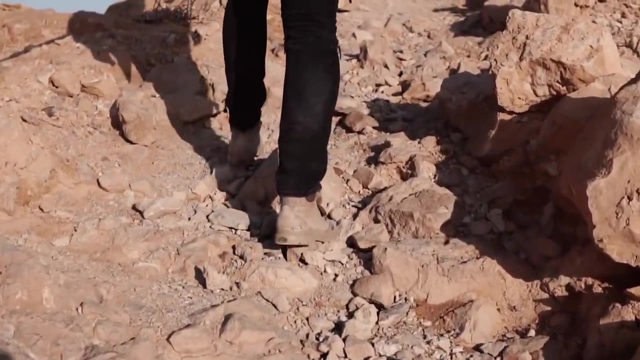 she doesn't hope to find a promising curl or lump producing from a rock's surface, and she would never expect to find her prize washed up among the scree at the base of a cliff. Instead, she is meticulous about documenting every geological detail of the freshness of the world. 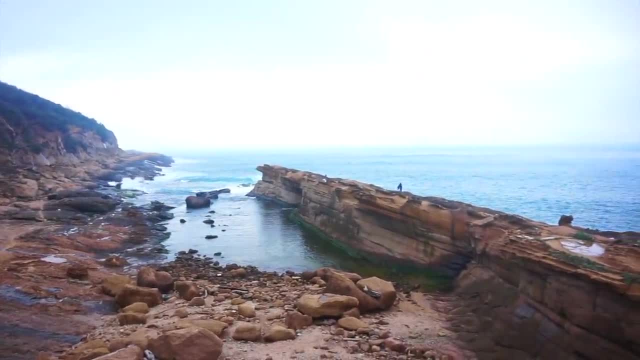 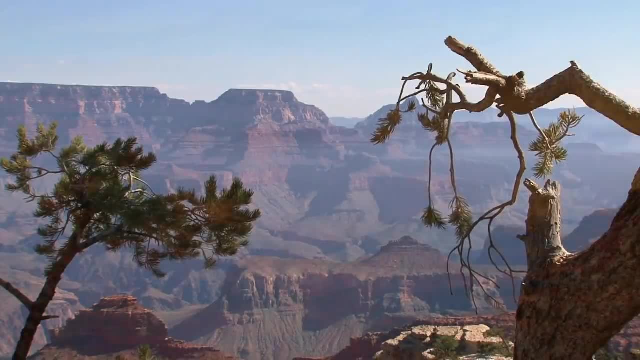 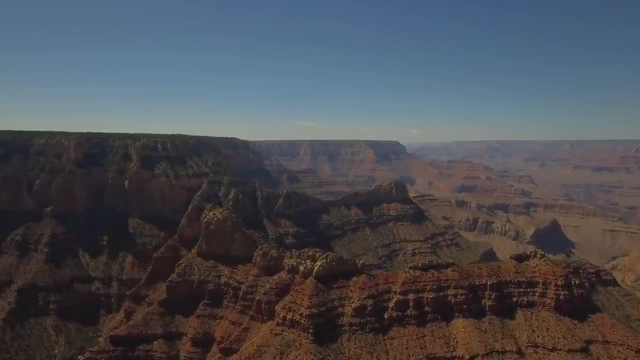 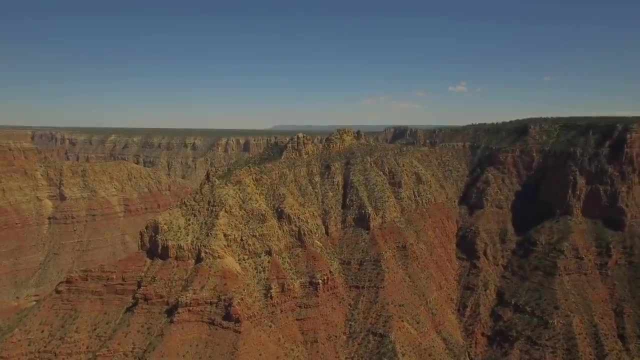 and what geological torture they have endured until now In strata that are sufficiently unaltered. she scours the rock for minute differences in the minerals that make them up, Extracting seemingly uninteresting slivers from within these layers. she labels them carefully, noting their position and orientation. 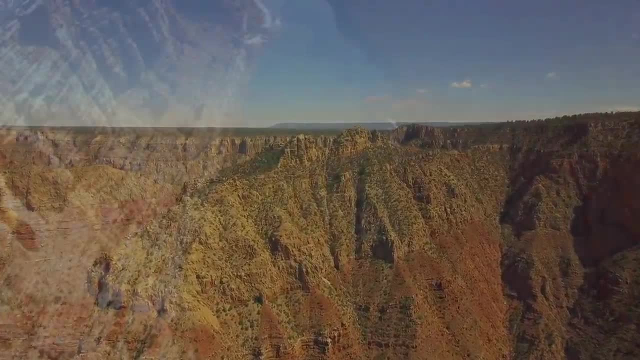 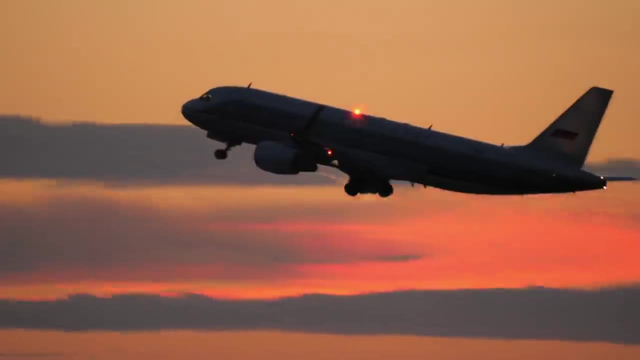 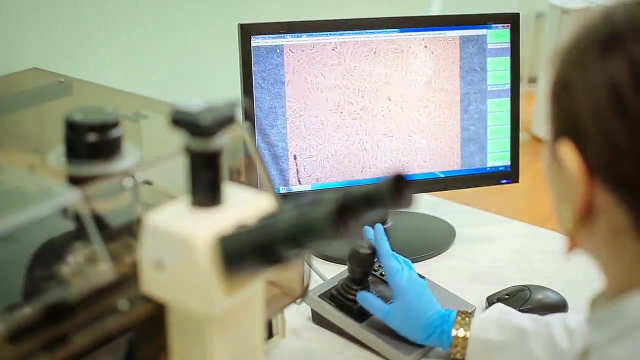 before unceremoniously tossing them into her backpack among tens of others just like them, packing them securely back at the hostel for the flight home. Back at the lab, it's time to process her finds, Some she will cut, exposing fresh surfaces that haven't seen the sun for a billion years. 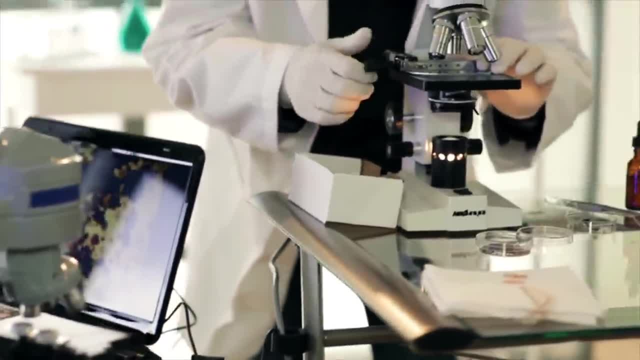 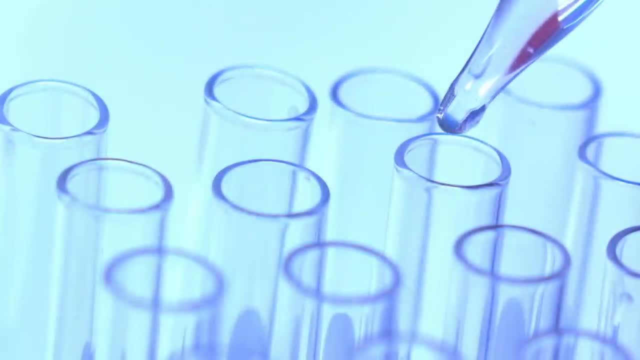 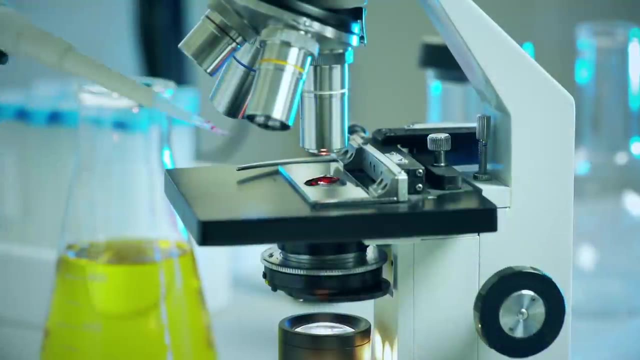 and then mount those surfaces onto glass slides and grind them until they are just a few tens of microns thick. Other samples she will dissolve in hydrofluoric acid, which will melt away all rocks and minerals, leaving only the organic matter behind. This too will be mounted onto glass slides and fixed in place. 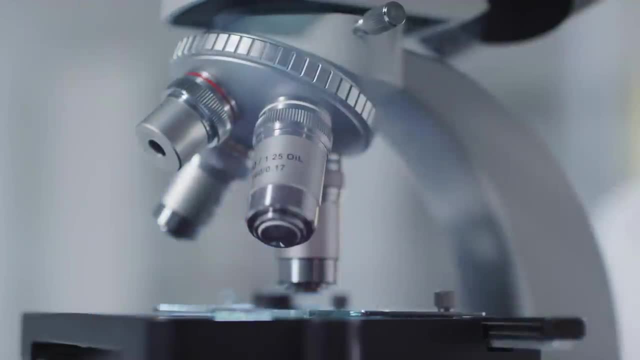 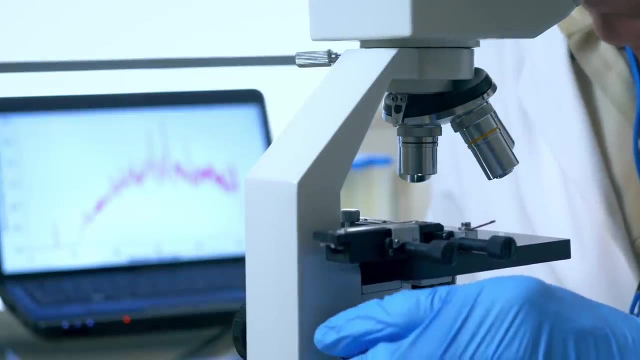 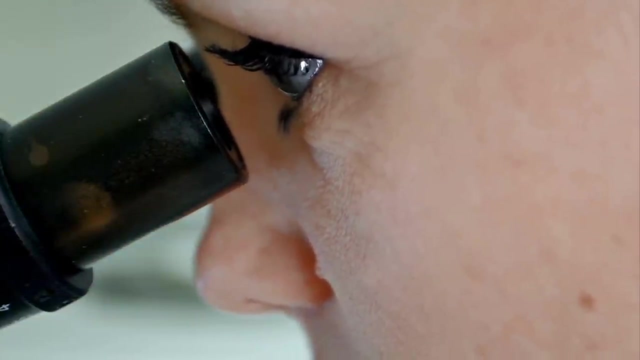 Finally, in a darkened room, thousands of miles from the journey's start, and thousands of hours later, she slips the glass slide beneath her microscope and picks it up. She appears with some trepidation through the eyepiece. Only then will she know whether she has found something or not. 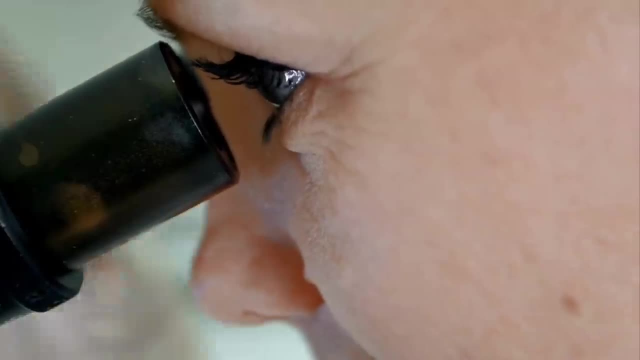 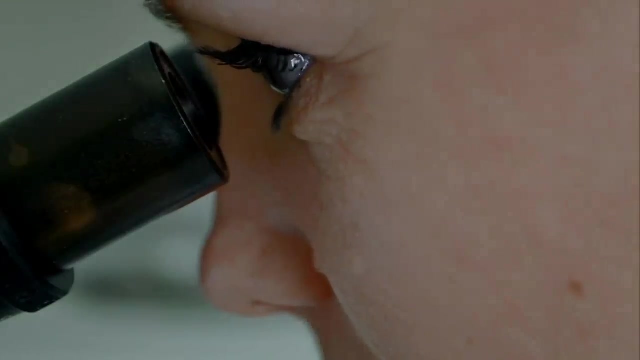 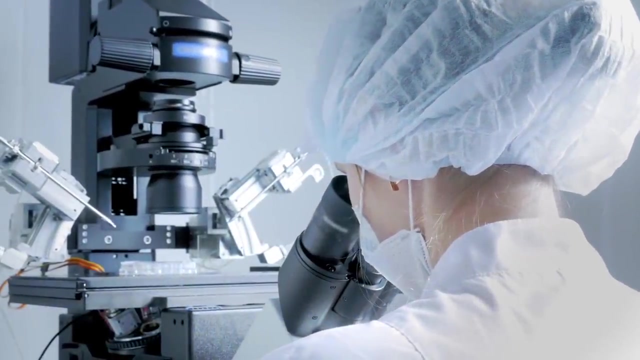 whether her training and geological eye has revealed a treasure of the Proterozoic or if all that work has been for nothing. It is an exhilarating feeling looking through the eyepiece and finding the bounty of the Proterozoic laid out. 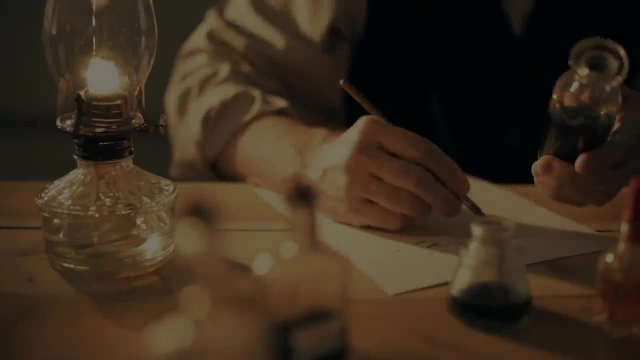 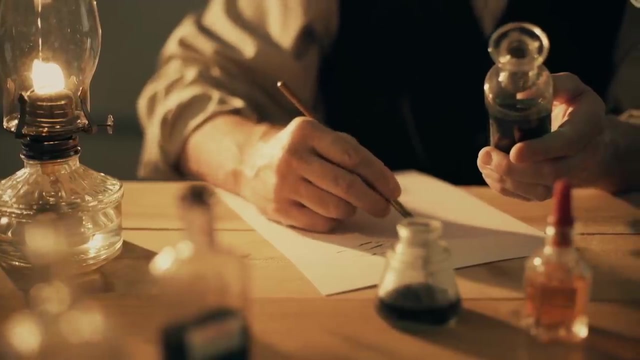 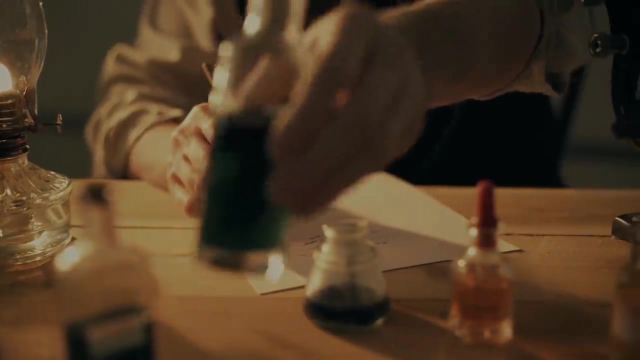 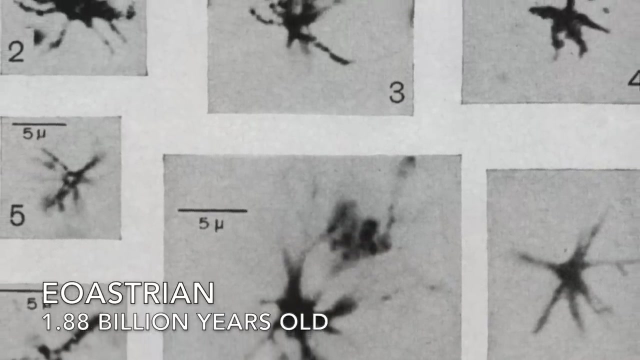 And it's a feeling that many paleontologists have experienced over the years. There have now been countless discoveries of microfossils from Proterozoic rocks all over the world, spanning huge swathes of time, The Gunflint biota, including the curiously star-shaped Eusatrion. 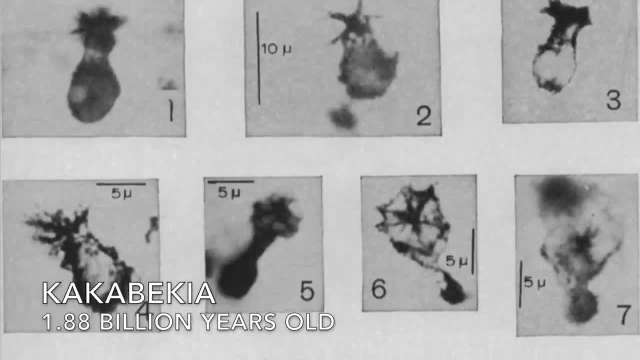 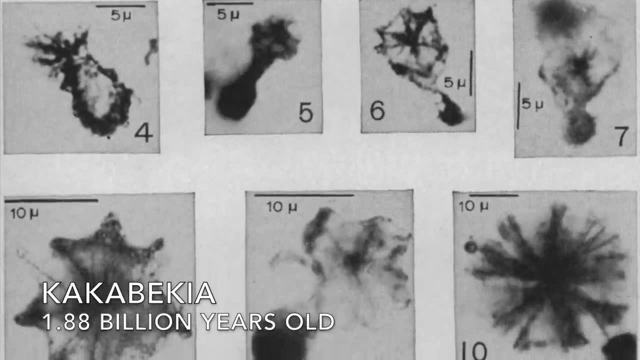 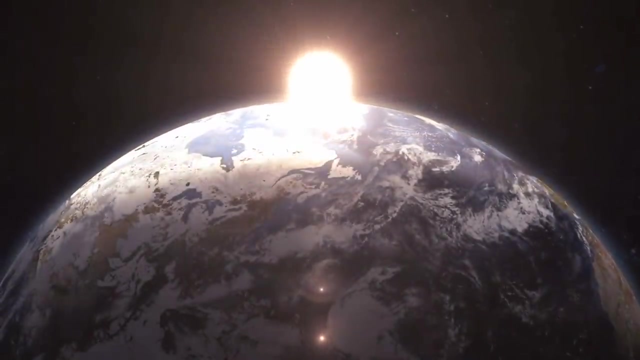 and umbrella-like Cacabecia is found consistently in the Gunflint Chirts of Western Ontario, dating to 1.88 billion years. Other microfossils are found from rocks all over the world, indicating their global dominance within the Mesoproterozoic. 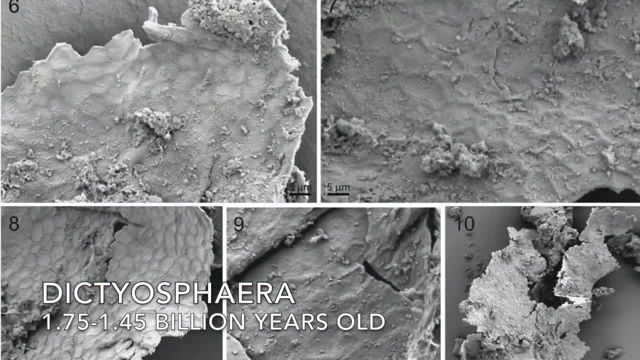 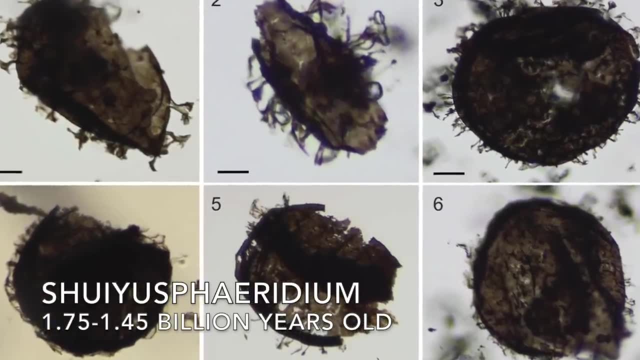 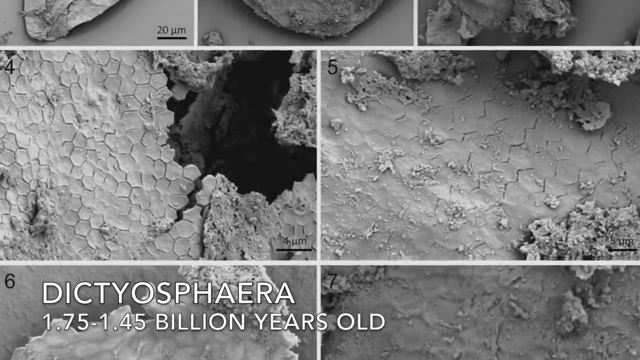 Finely reticulated spheres of Dictyosphera sit alongside Tapania and Shuiu spheridium, with their branching and interlinking spines. All are found in rocks of China and Australia dating between 1.75 and 1.45 billion years old. 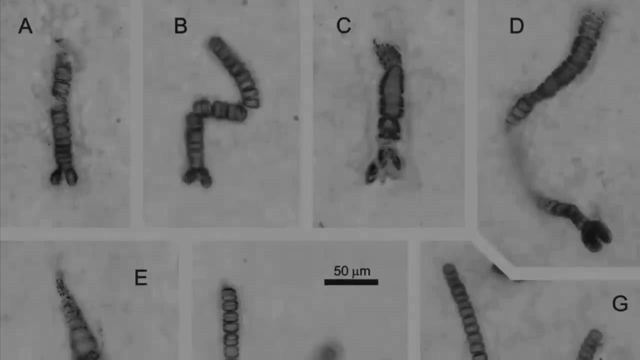 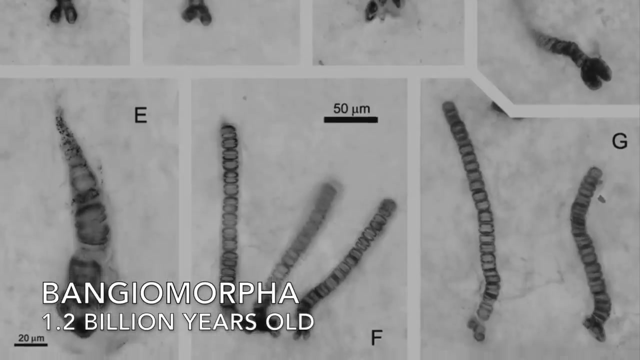 Slightly younger rocks of the Proterozoic dating to 1.2 billion years are found in the Hunting Formation in Canada, and these are host to a curious association of seemingly differentiated cells. Different shapes are confined to different parts of the organised structure. 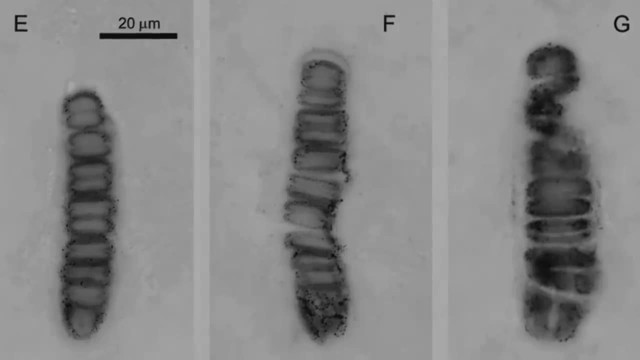 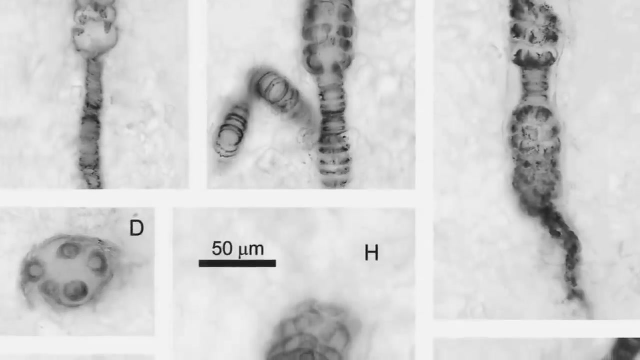 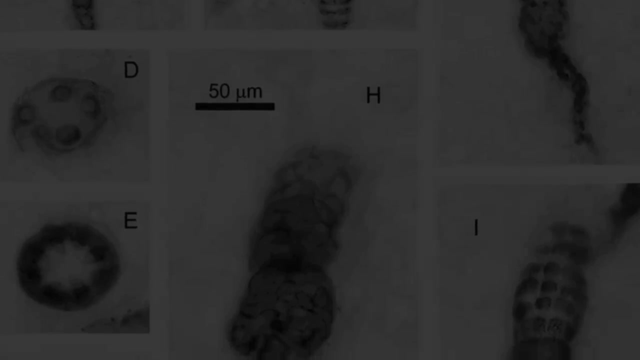 And paleontologists believe this is one of the earliest instances of complex and consistent multicellularity and sexual reproduction. By one billion years ago, eukaryotic cells have even made it out of the oceans and onto land, or at least into the non-marine waters of the Torridon Lakes of modern-day North West Scotland. 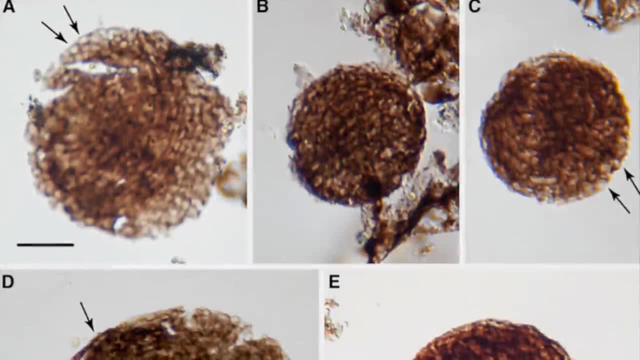 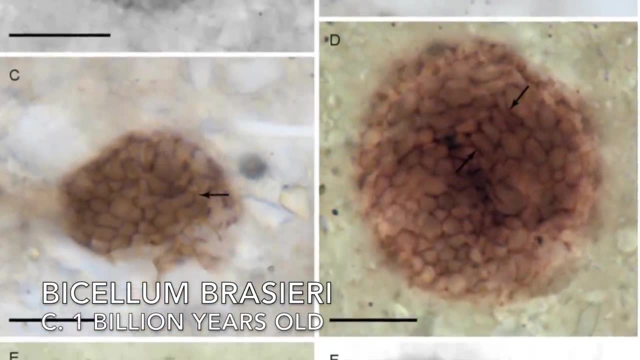 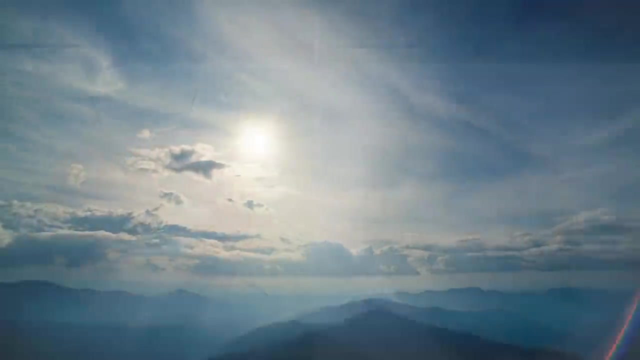 One species native to these ancient lakes is Bicellum brassieri, also featuring differentiated cells. Even before the end of the Boring Billion, it seems that life is already well on its way to complex multicellularity. But what of the deeper history of eukaryotes? 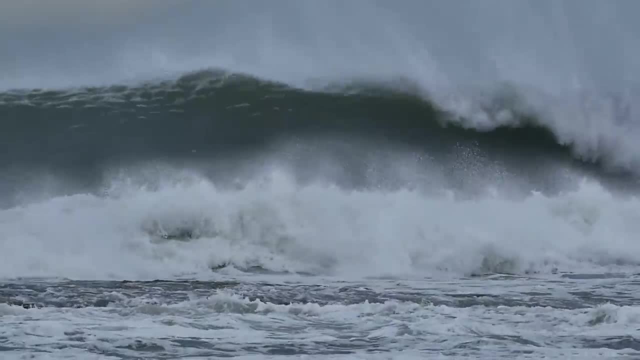 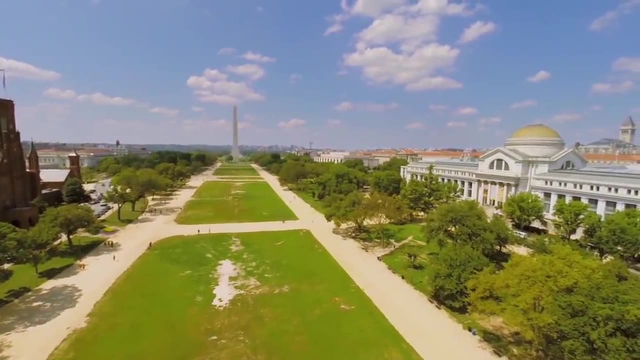 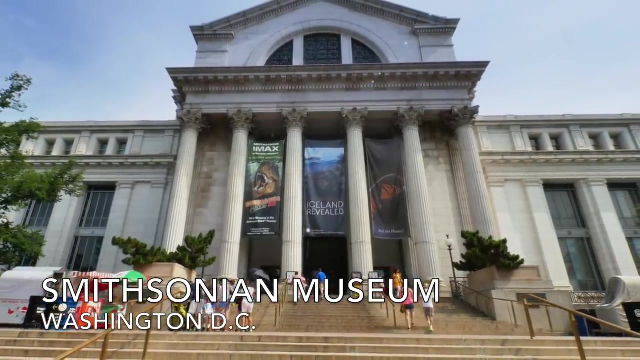 Eukaryotes, Our modern protozoic paleontologists, no longer needs to worry about a paucity of fossils. to study, To compare her finds with ones that have already been documented, she visits the Smithsonian Museum of Natural History. She wastes no time with the exhibits, impressive as they may be. 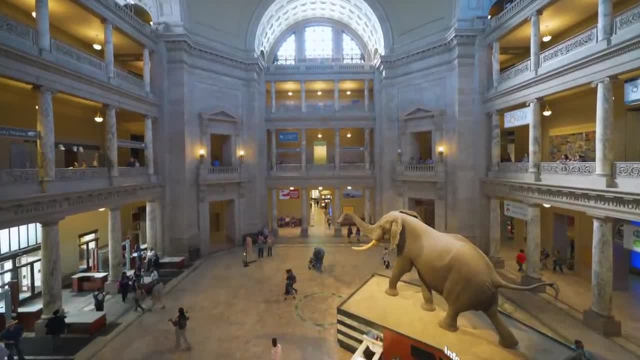 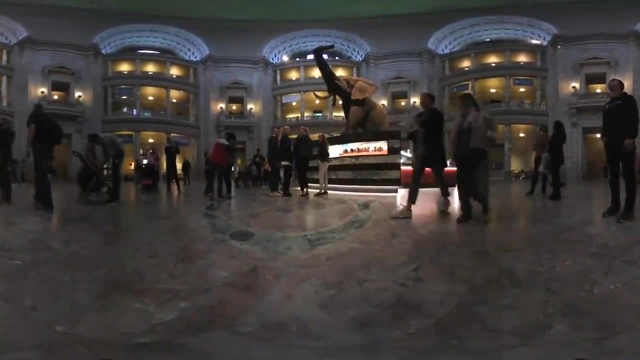 walking past T-Rex skeletons and gigantic fossil stromatolites to a small unmarked door in the corner of one of the halls. She steps through the door and into a different world. She steps through the door and into a different world. 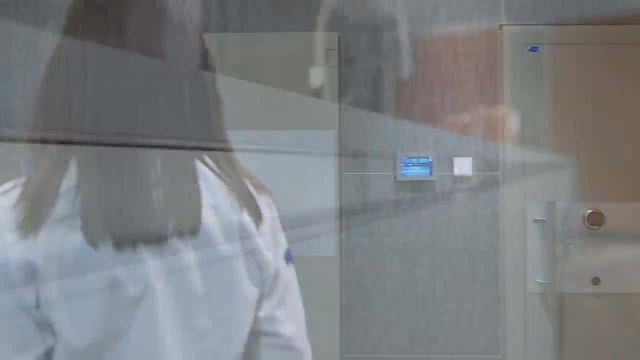 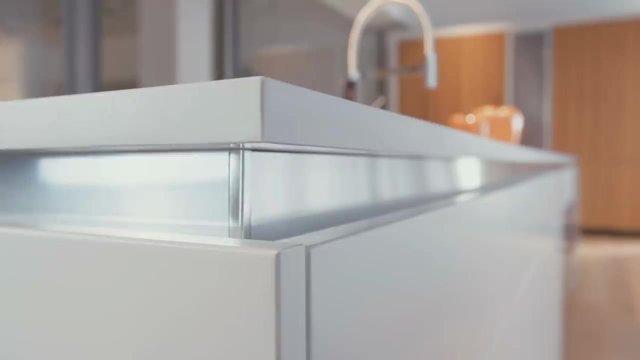 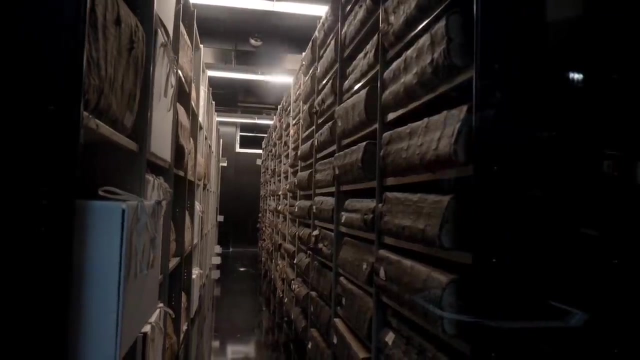 Gone are the information board's creative lighting and screaming children, and she is instead faced with passageways lined with cabinets gathering dust that dulls their already monochrome colour scheme. Navigating this backstage labyrinth, she eventually finds herself in the same room as the fossils she is searching for. 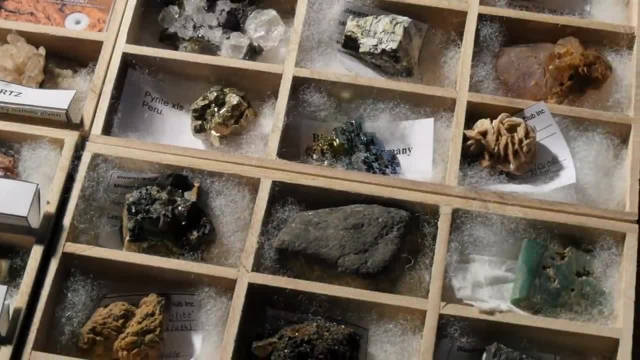 Navigating this backstage labyrinth, she eventually finds herself in the same room as the fossils she is searching for, but she still has to work to find them. The good thing about microfossils is that they don't take up much room. 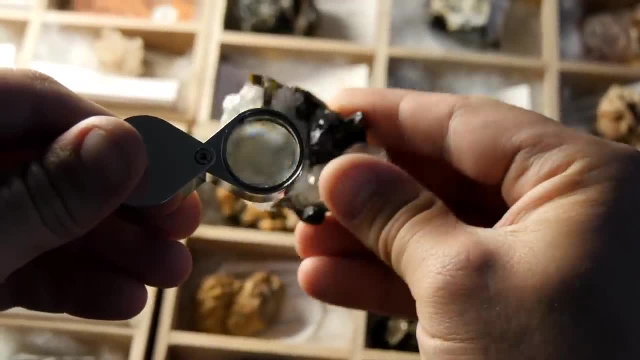 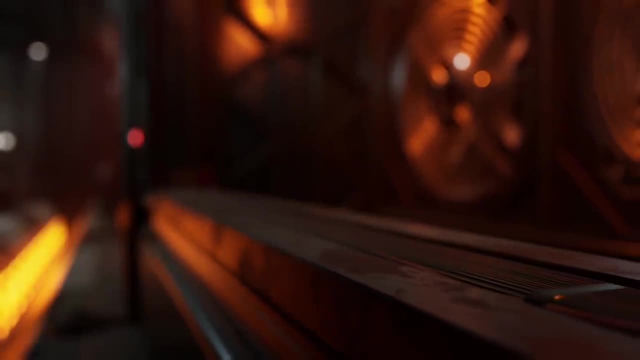 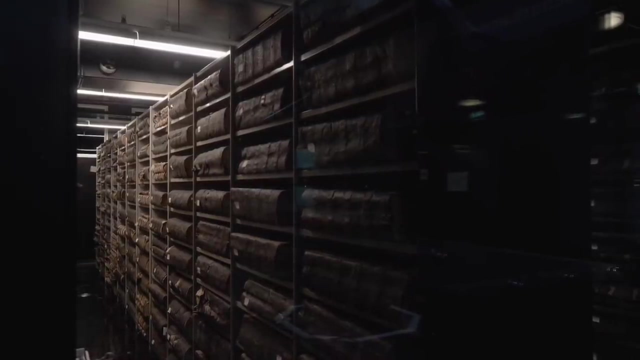 but 70 years of protozoic paleontology has nevertheless accumulated an impressive number of specimens. Cabinets stretch floor to ceiling and are crammed in back to back with scarcely room to slide a piece of paper between them. But these stores are mounted on wheels driven by geared winding handles. 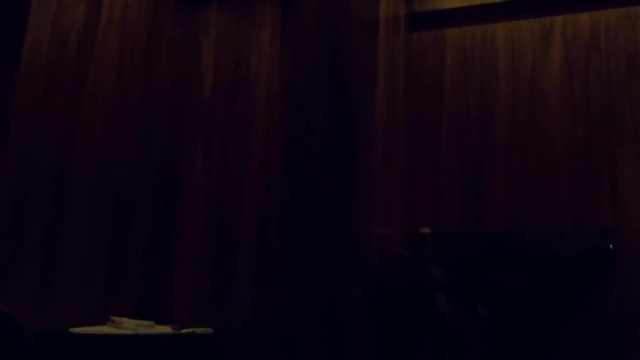 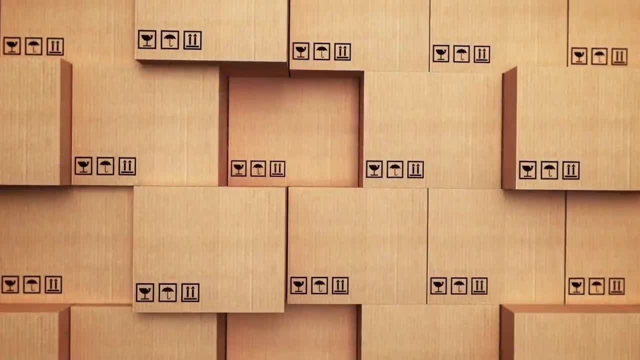 allowing her to walk along the newly created space and commence her search in earnest. allowing her to walk along the newly created space and commence her search in earnest. The store is filled with brown shoeboxes, each full of protozoic treasures, mounted on their glass slides and labelled with a careful hand. 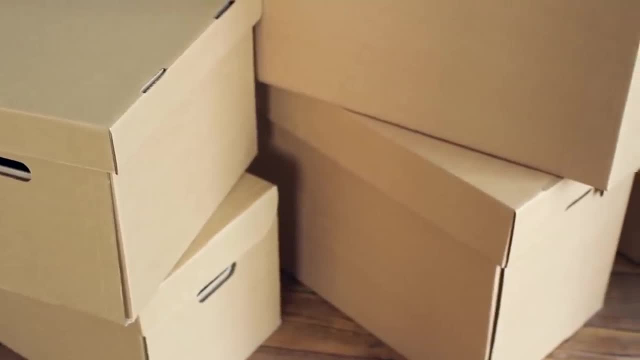 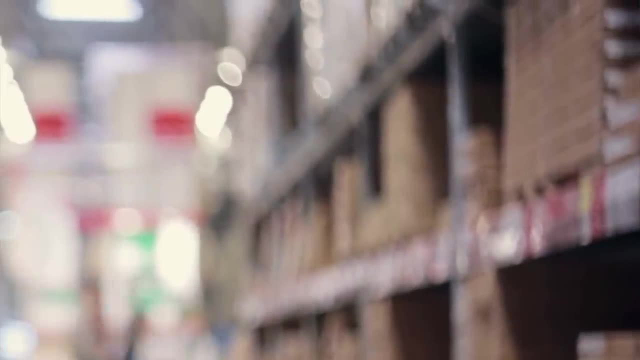 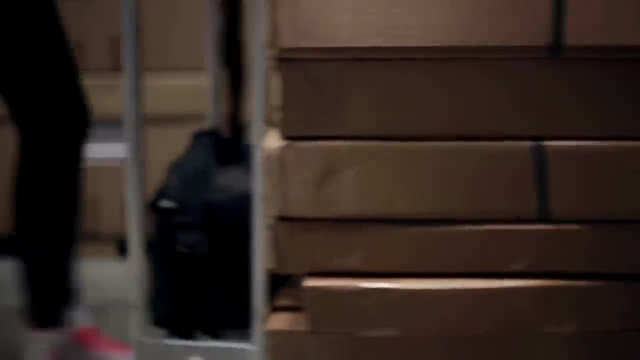 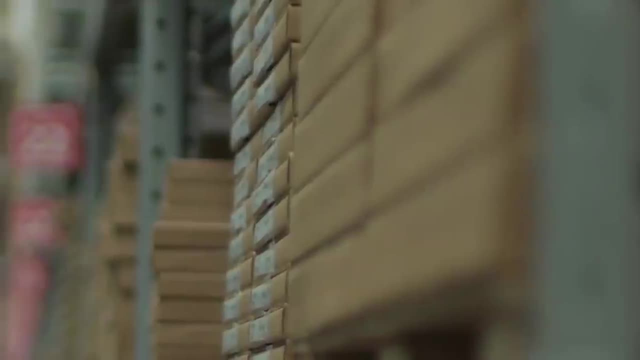 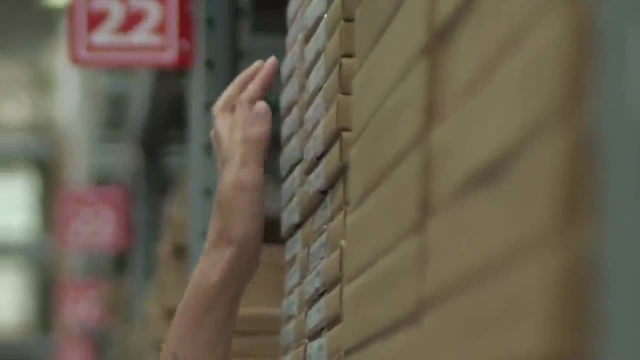 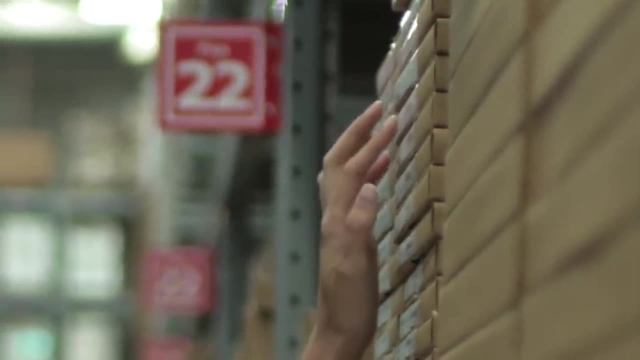 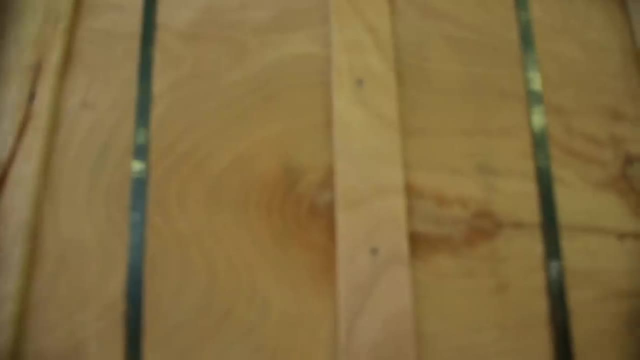 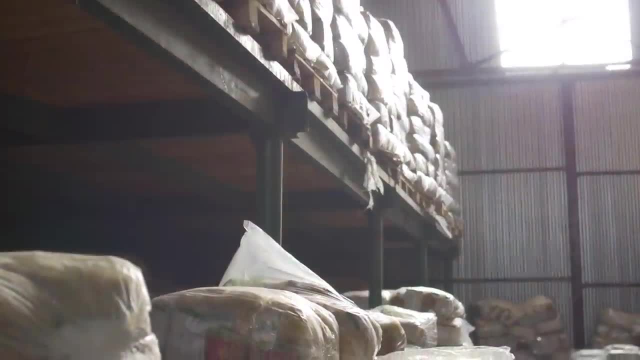 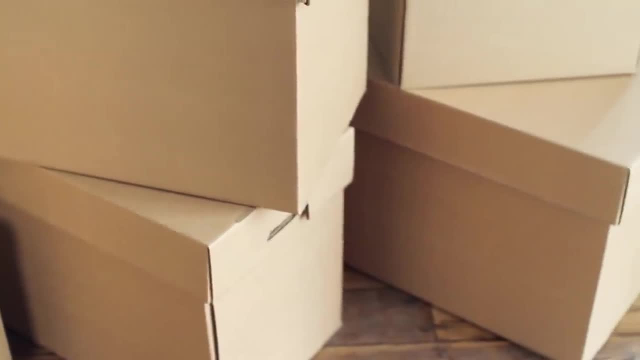 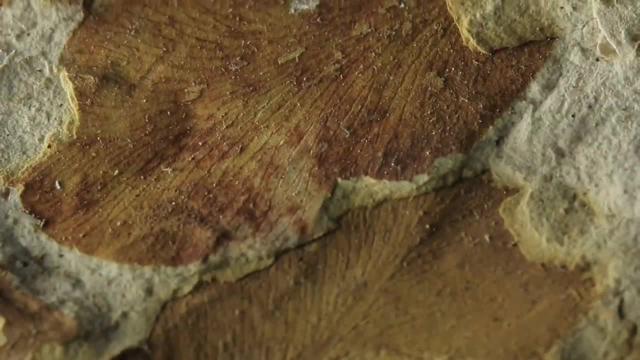 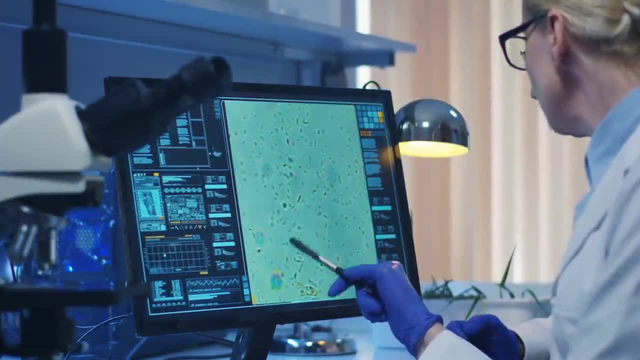 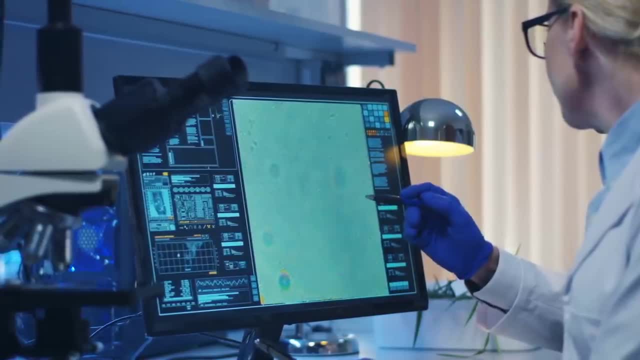 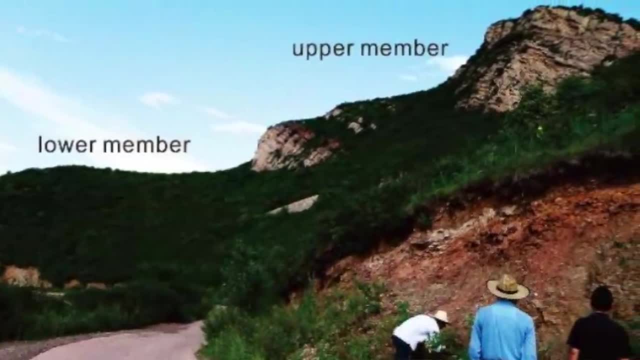 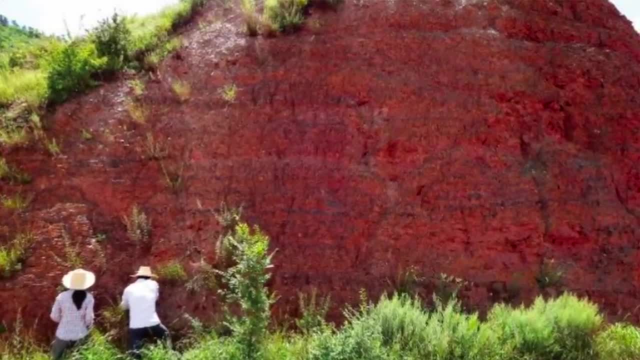 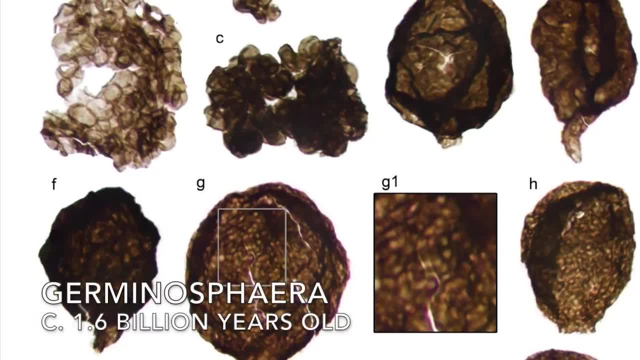 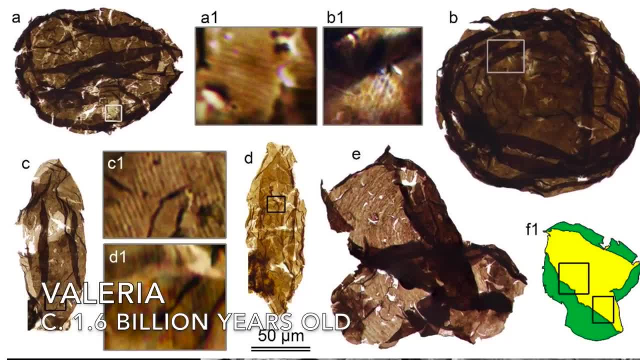 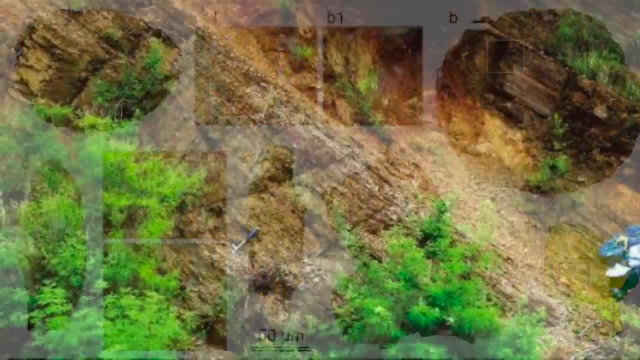 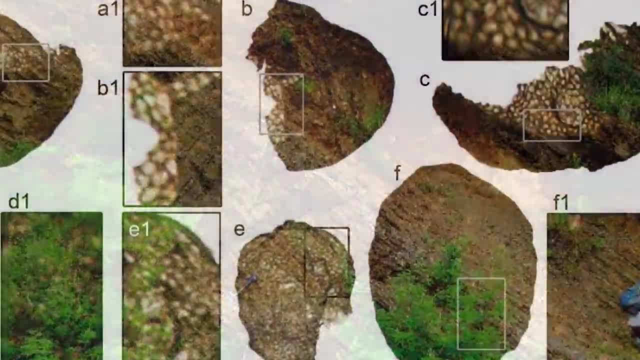 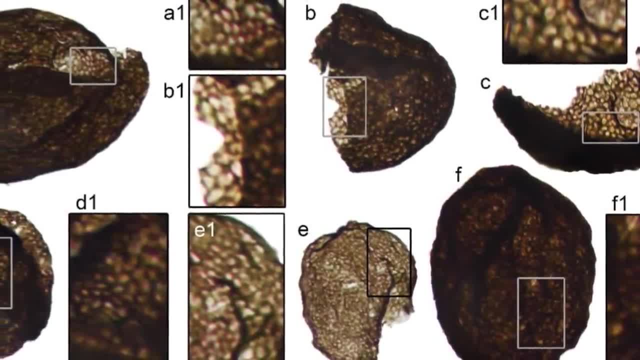 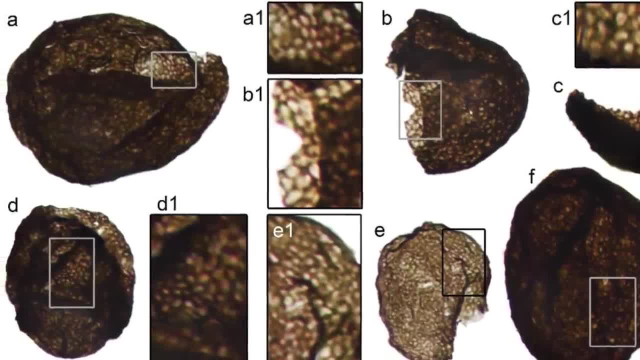 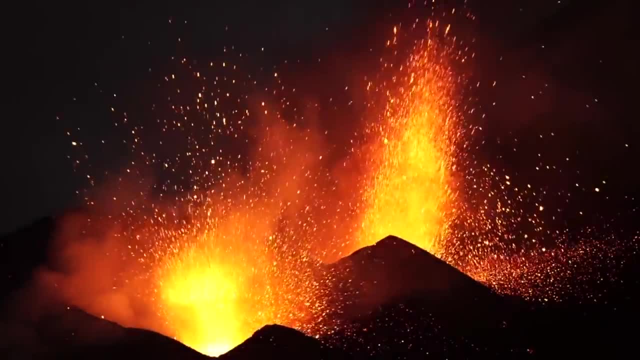 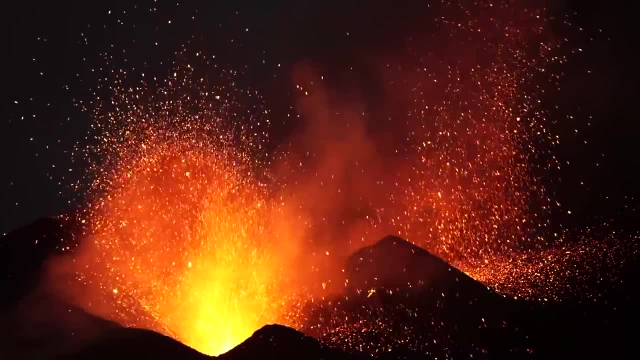 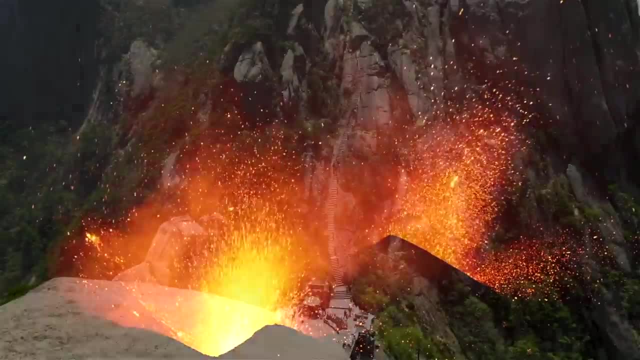 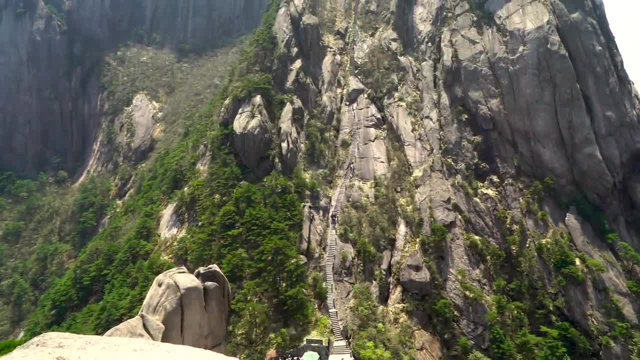 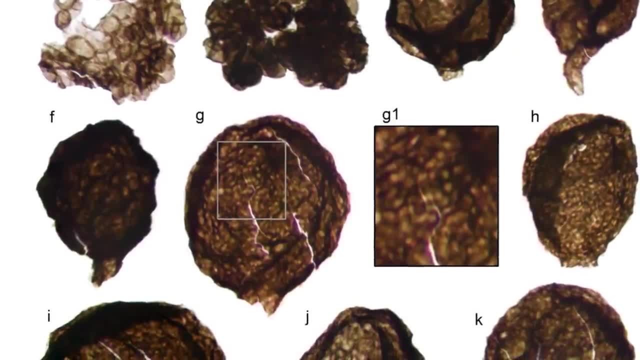 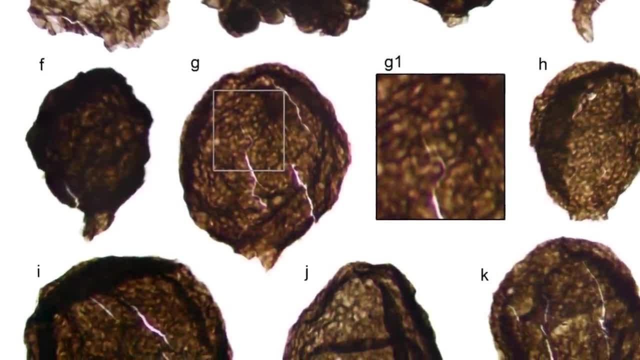 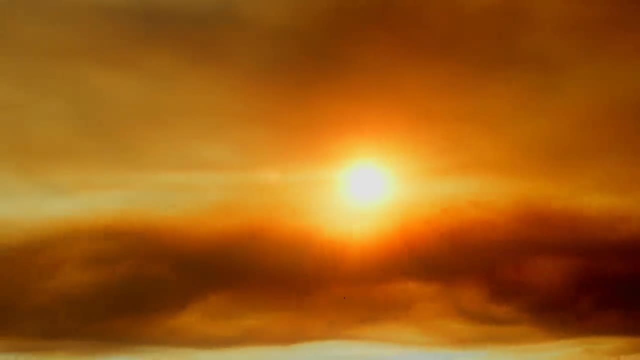 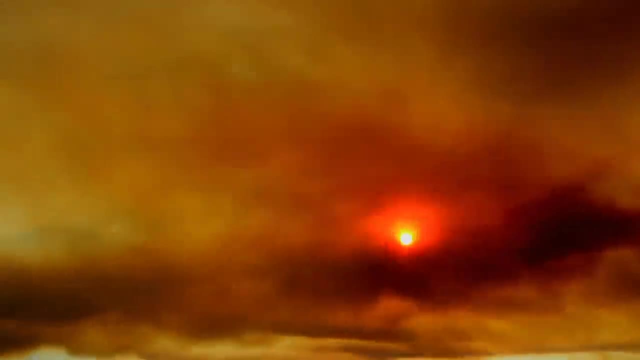 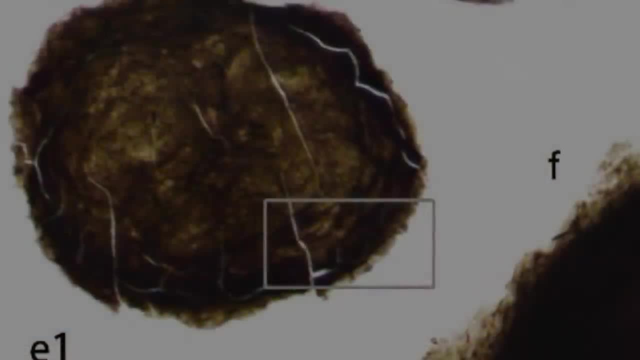 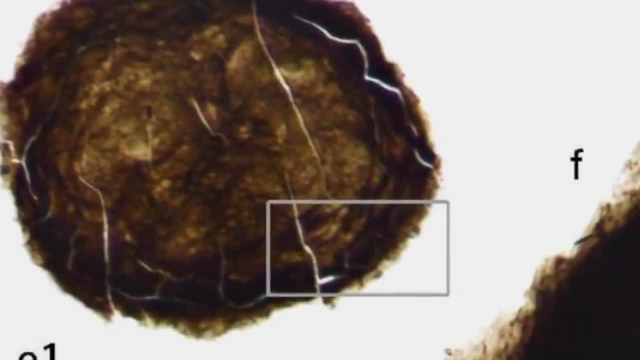 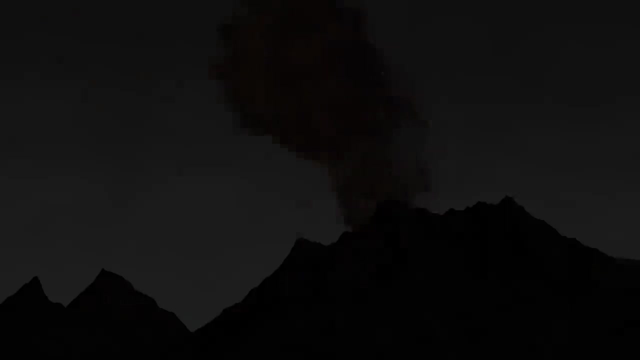 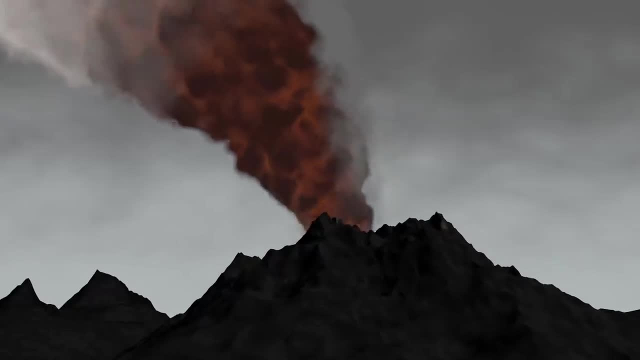 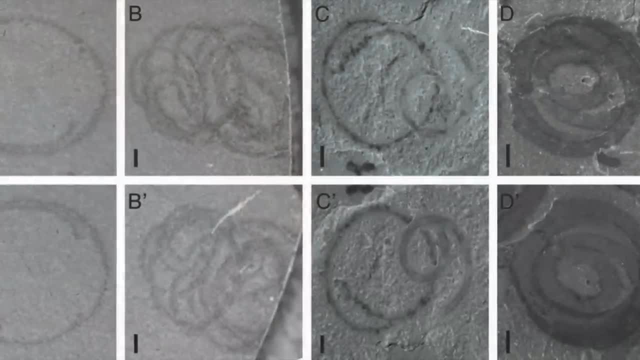 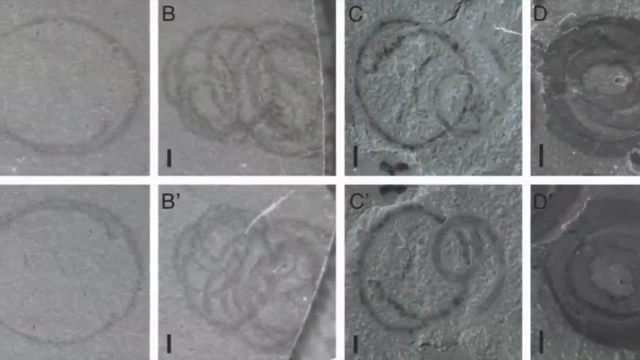 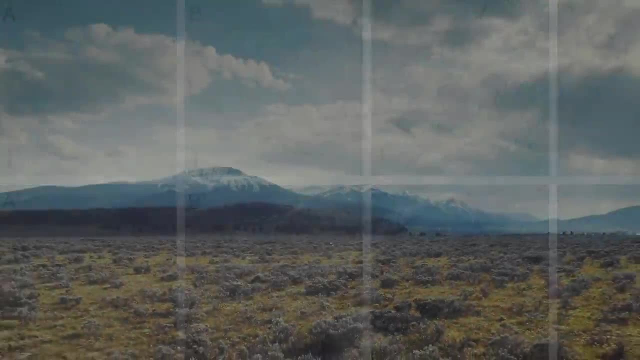 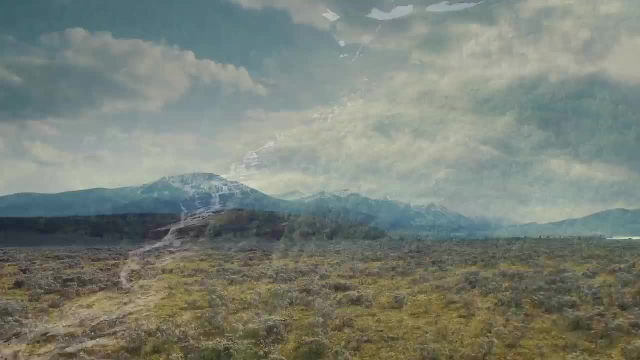 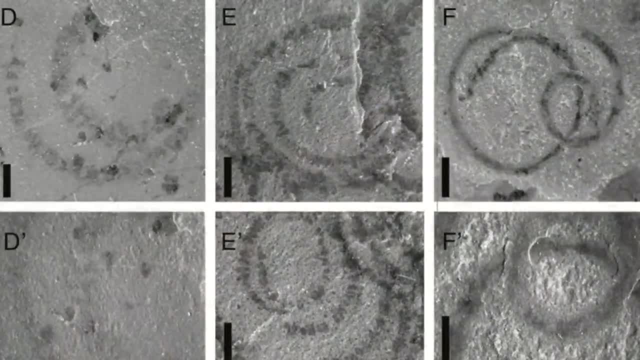 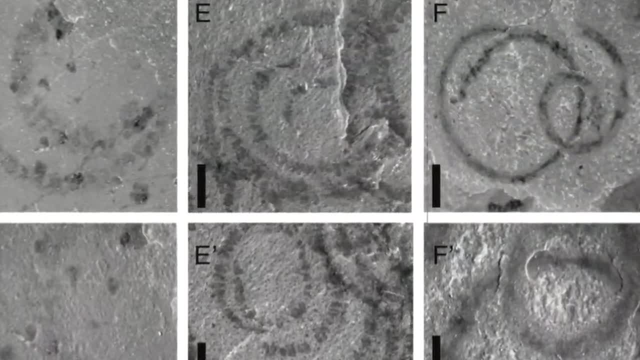 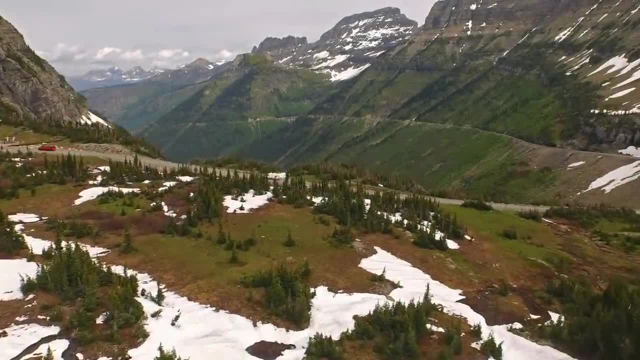 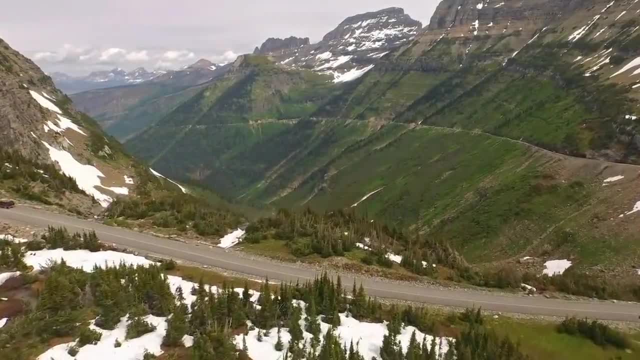 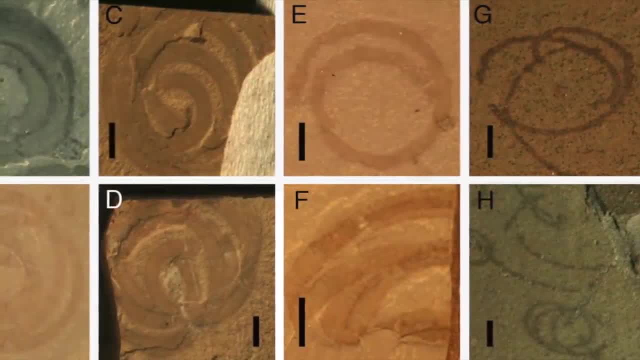 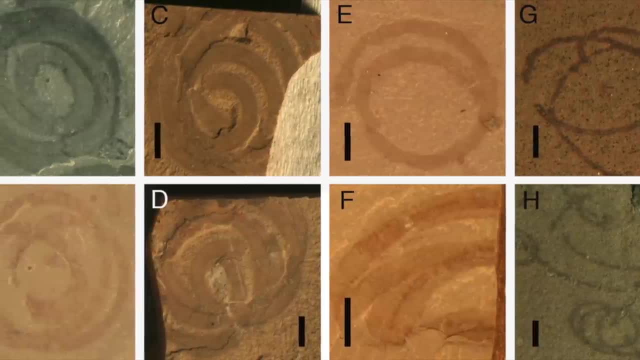 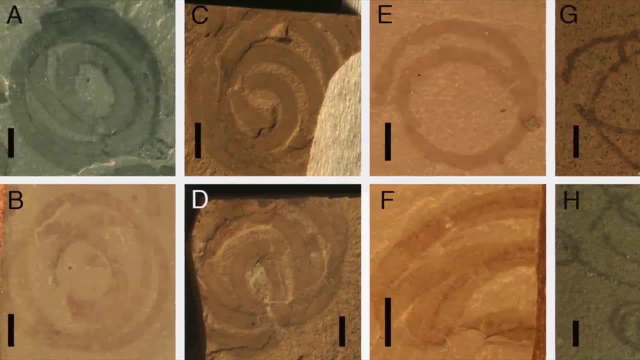 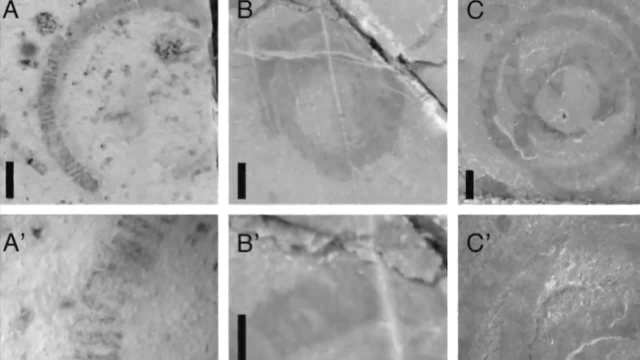 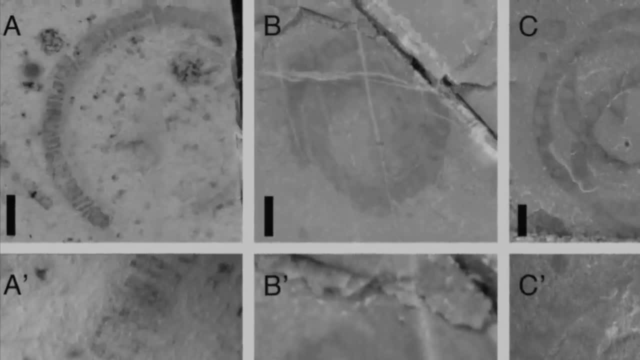 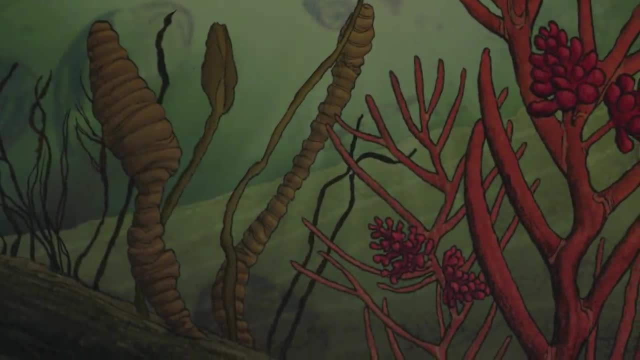 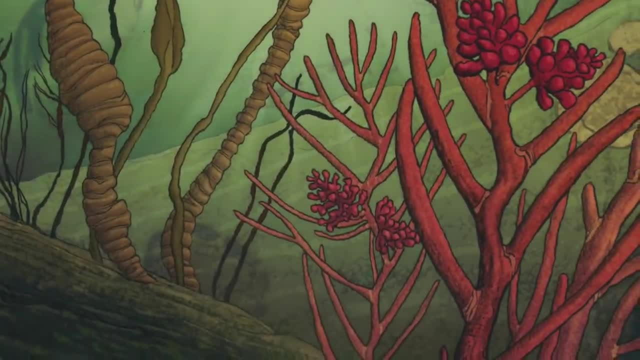 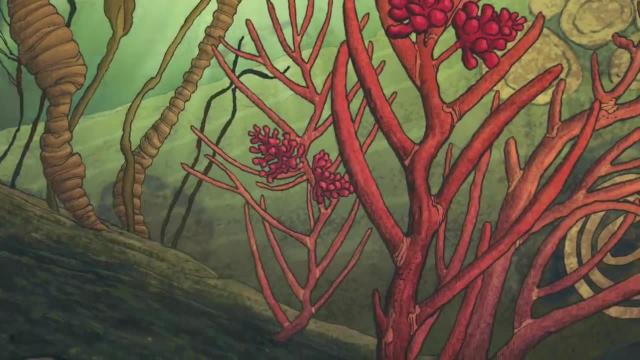 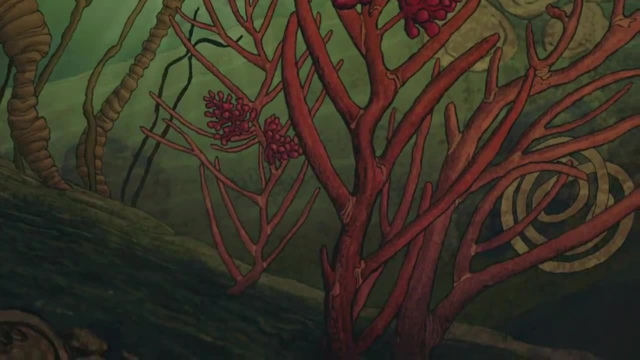 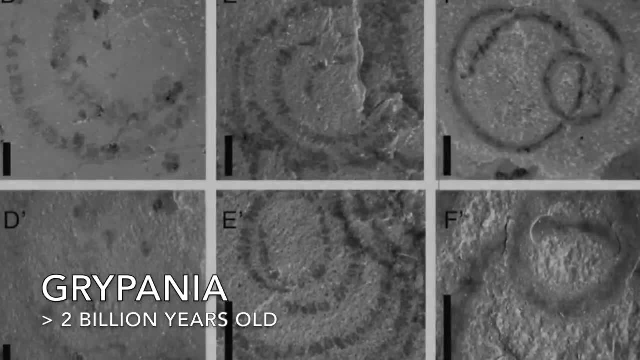 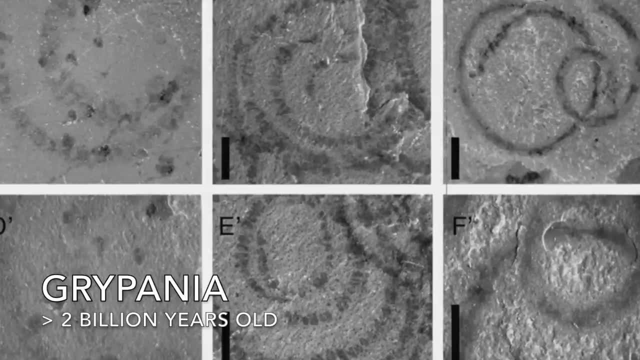 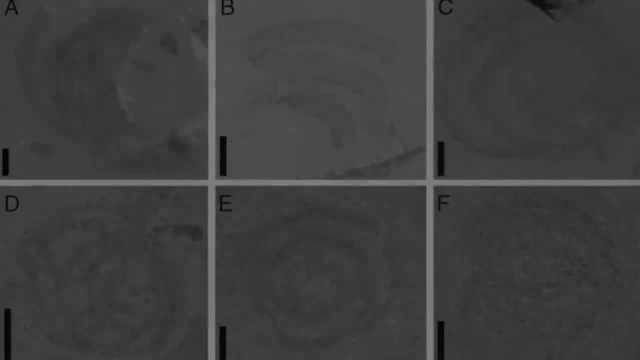 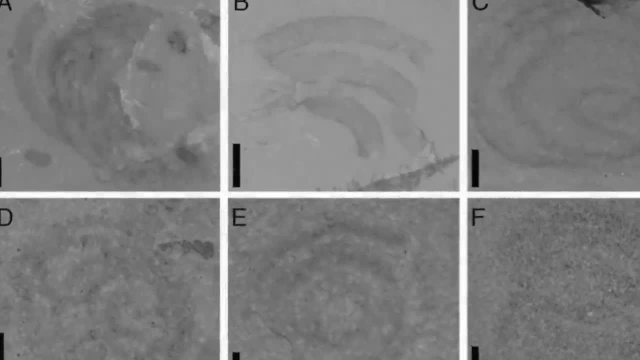 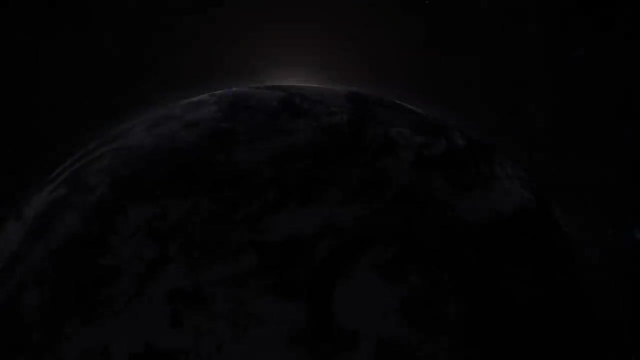 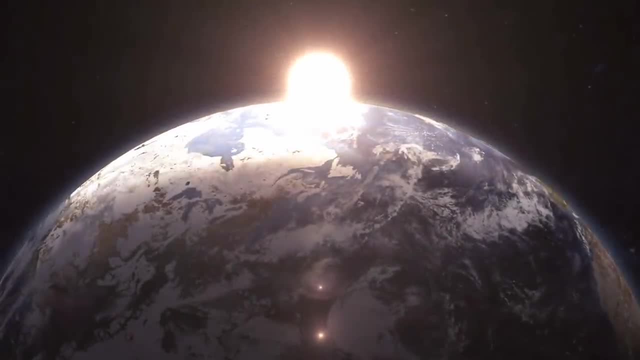 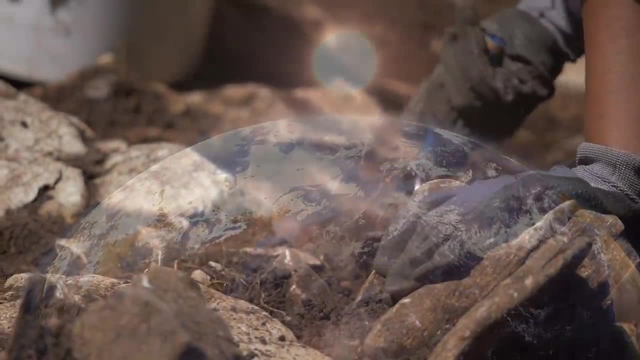 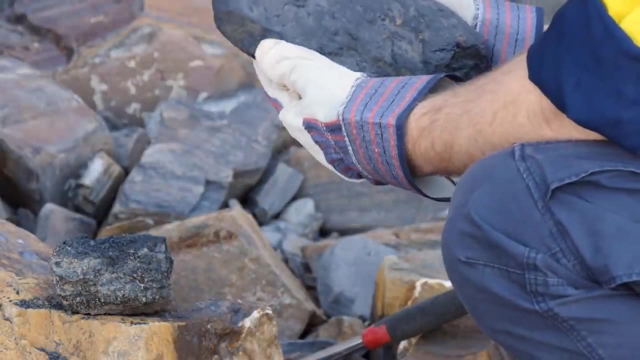 Older carbon-rich fossils have been discovered in fine-grained shales dating to 3.2 billion years old. Some have argued for their eukaryotic nature based on their large size At 300 microns, or three-tenths of a millimetre. they are much smaller than Grippania. 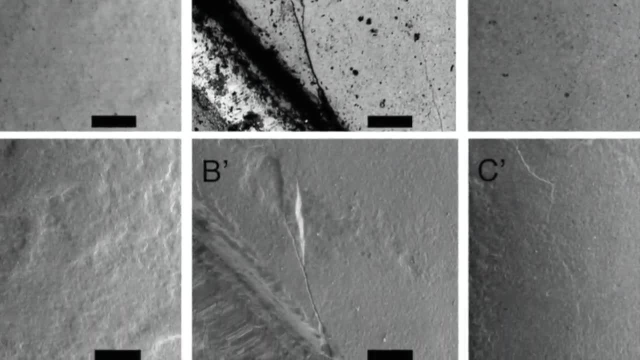 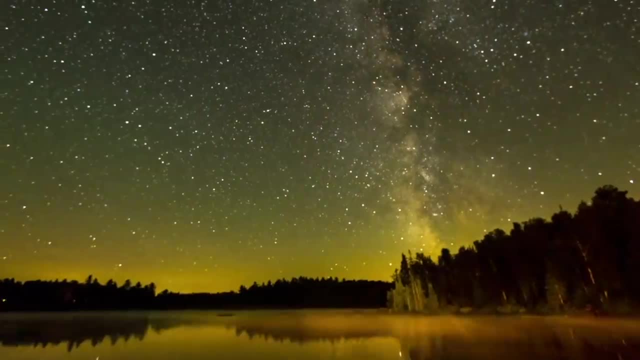 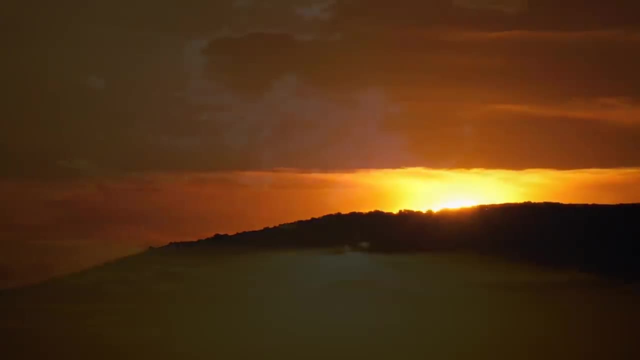 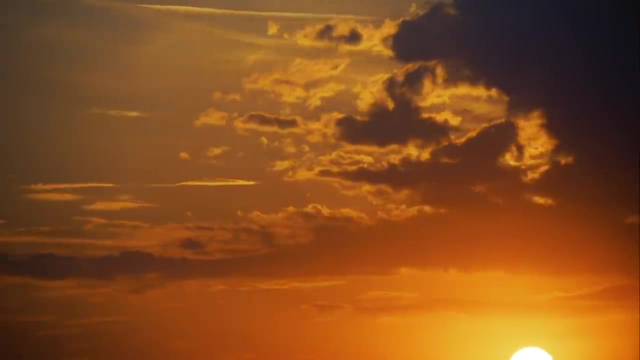 but still larger than most known bacterium. For this extraordinary claim, however, there is no more evidence. Of course, other methods have been devised to try and trace eukaryotes back to their roots through Earth history, Just as the cellular machinery of these more advanced cells can create complicated structures on the outer wall. 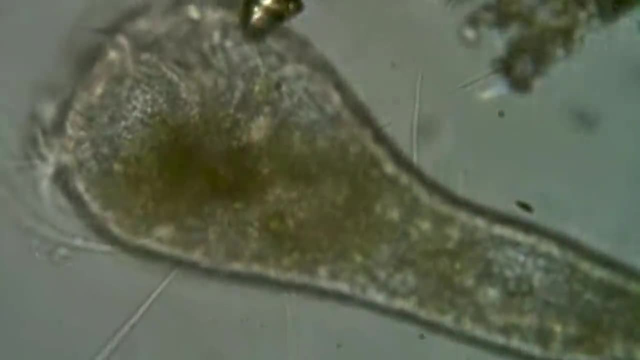 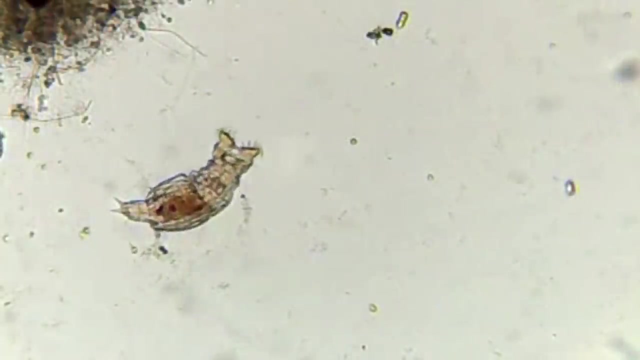 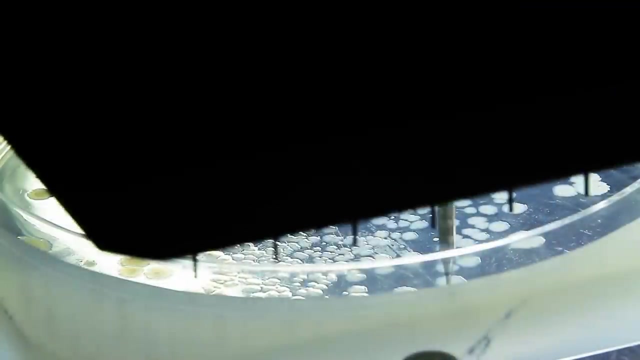 so too can they produce complicated chemistry that no physical or prokaryotic process can replicate, And so there is still no consensus on how to verify the antithesis of eukaryotic chemistry Or the antiquity of a molecule. Other techniques can involve the analysis of genetic change and differences among living eukaryotes. 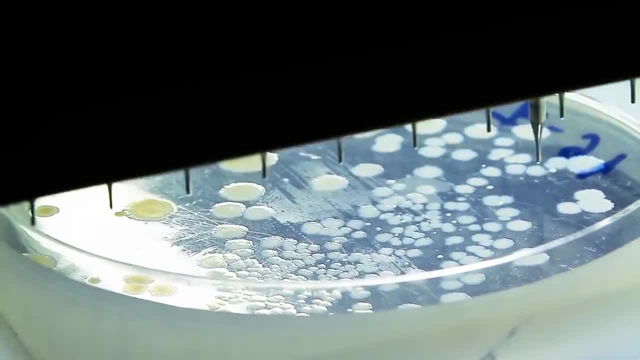 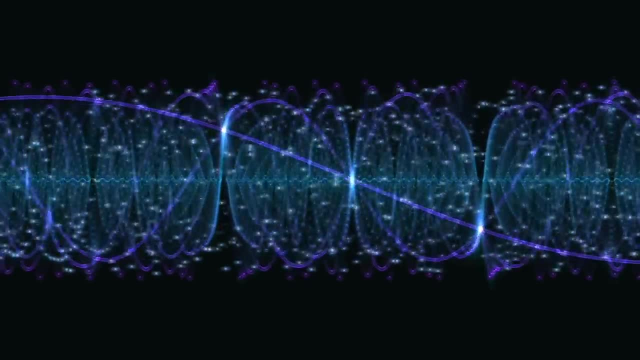 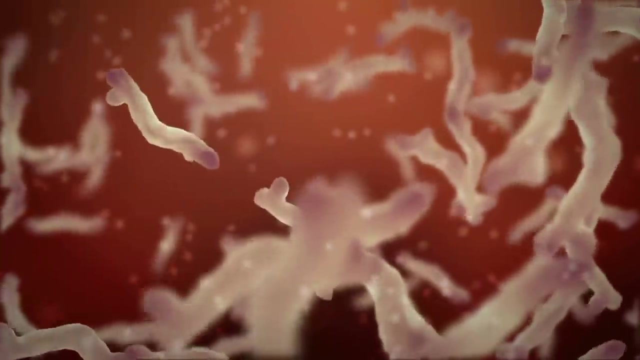 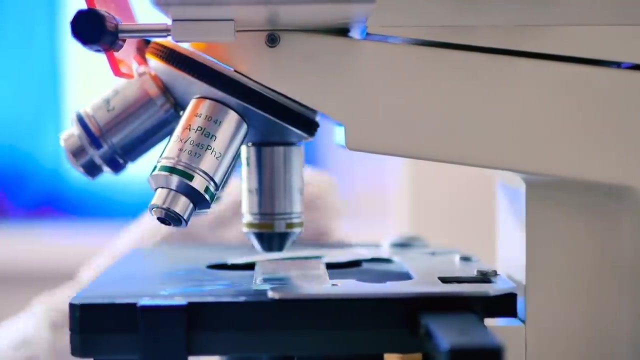 Reconstructing family trees of the eukaryotic kingdoms and tracing those trees back to their roots using an assumed rate of evolutionary change. so-called molecular clocks can put a date on the origin of eukaryotes with no fossils necessary. Some of these analyses also pin the beginning of complex cells to a date of around 2.7 billion years. 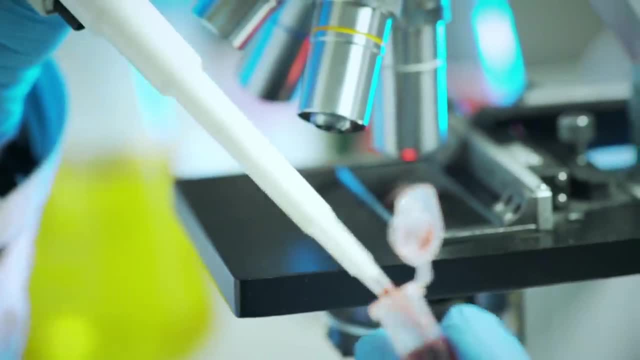 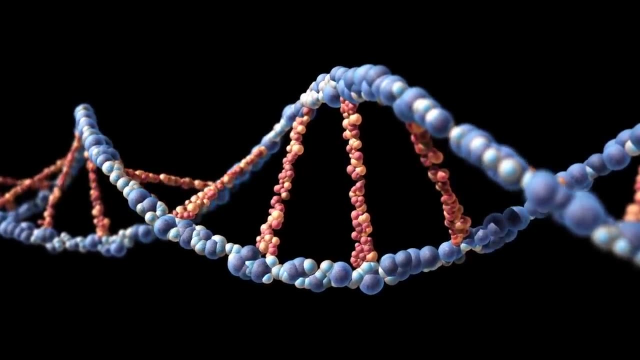 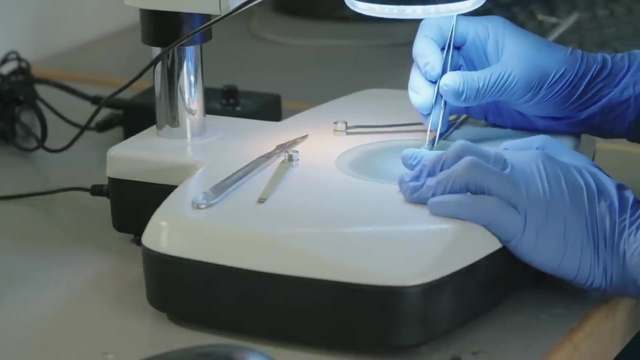 But there is by no means a consensus on the approach used to arrive at that date. There are so many assumptions in the shape of the evolutionary tree and the rate of change over evolutionary time that any proposed dating becomes all but meaningless. Today, the Precambrian fossil record has been revealed to us. 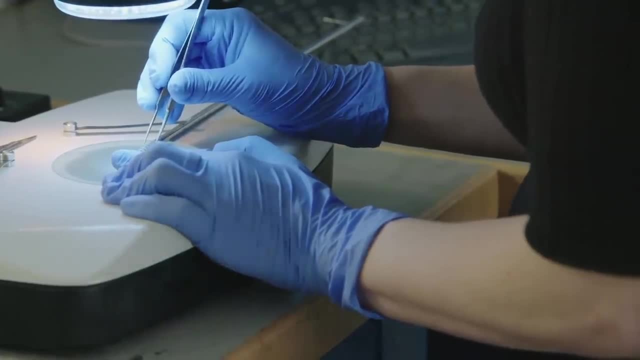 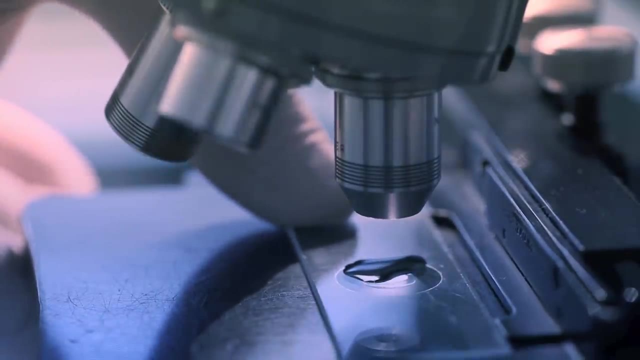 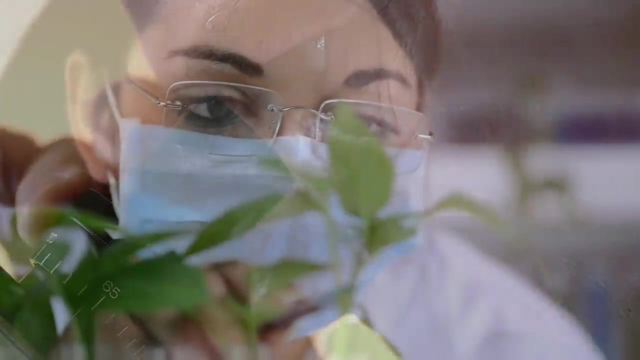 In all its glory. We are pretty certain we know how complex eukaryotic life came about And we have a good and growing history of how it developed in its earliest billion years or so. But finding the very first eukaryote, the basis for all complex life to come, is a much harder task. 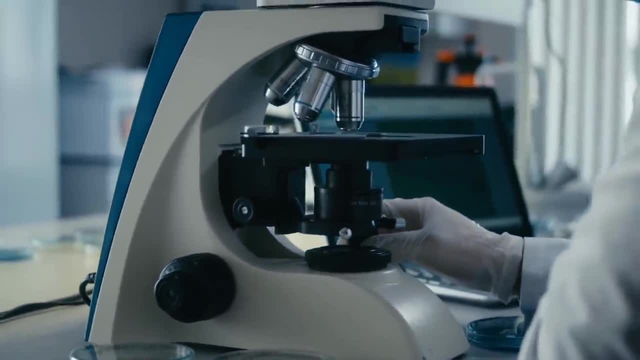 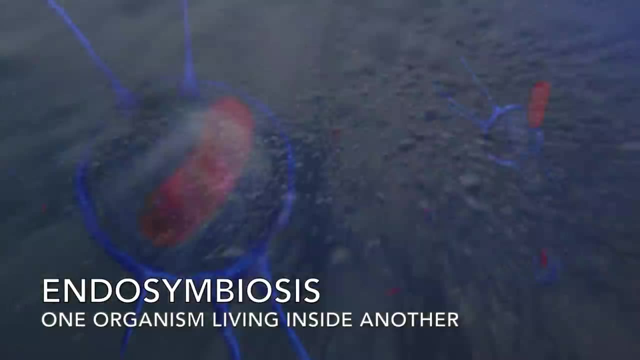 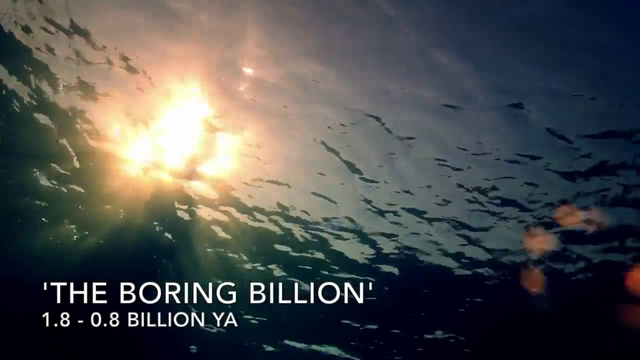 It is likely that eukaryotes as we know them today actually came about gradually, Beginning with the sealing of the endosymbiotic pact and continuing with the iterative development of internal architecture throughout the relative stasis of the boring billion Approaching evolution from the more traditional direction. 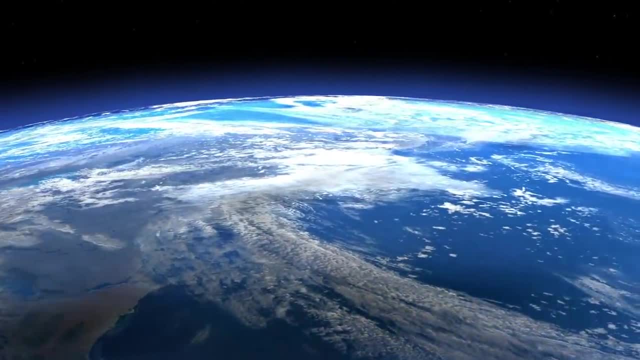 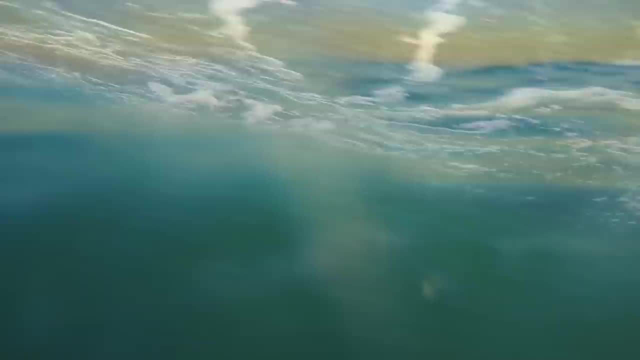 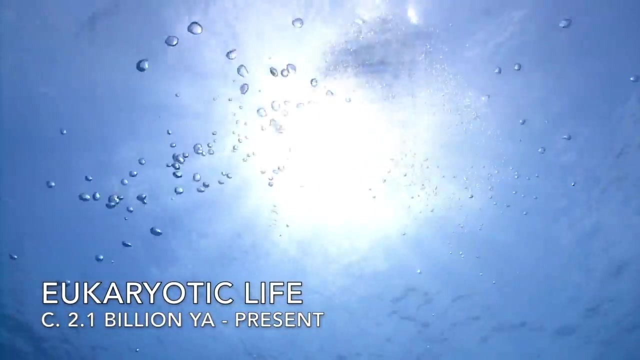 the invention of membrane-bound organelles and nucleus, as well as an organisational cytoskeleton and the internal chemistry needed to support it, would take an extremely long time. Thus, instead of modern eukaryotes appearing fully formed at some point in the Proterozoic 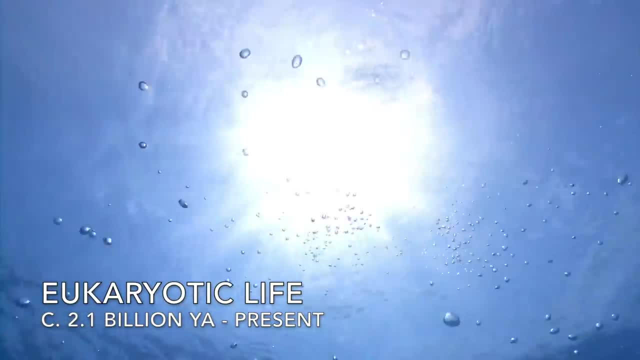 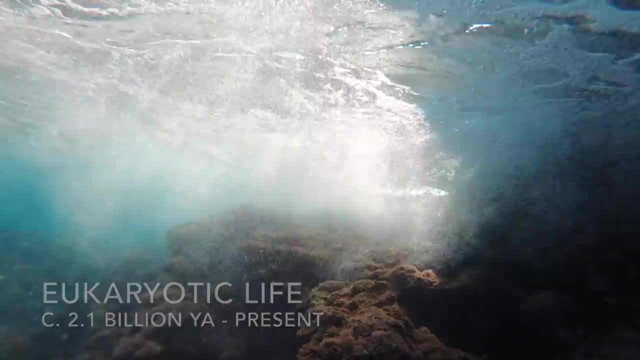 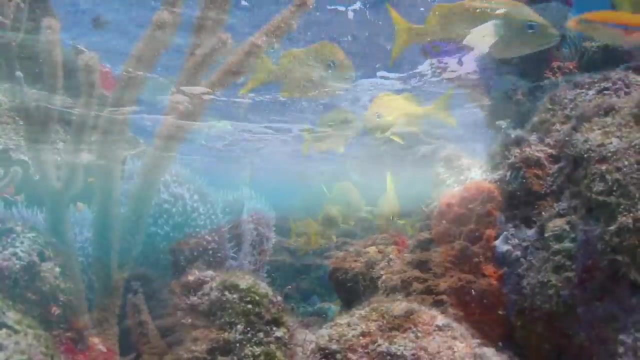 we can expect a sliding scale of complexity, From cells that are barely improved prokaryotes to cells that are capable of combining in their multitudes, differentiating and building the world as we see it today. This increasing simplicity as we trace the fossil record deeper into the Precambrian is matched by